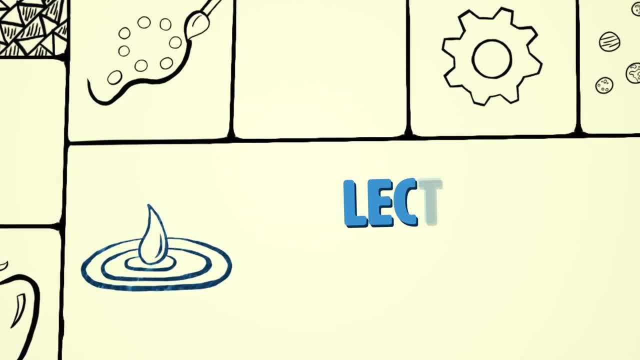 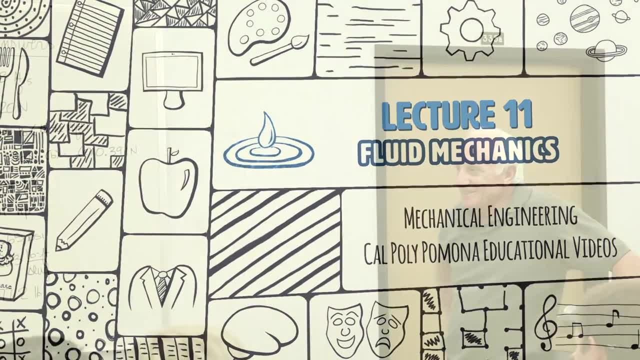 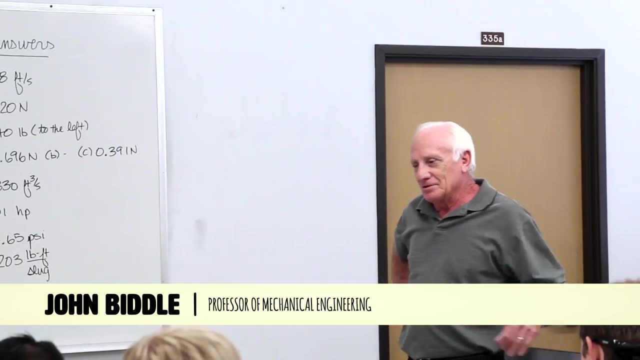 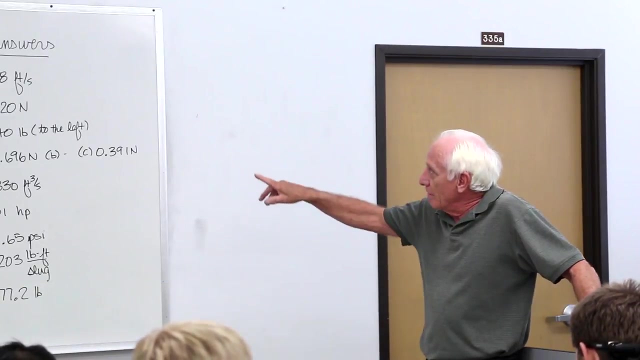 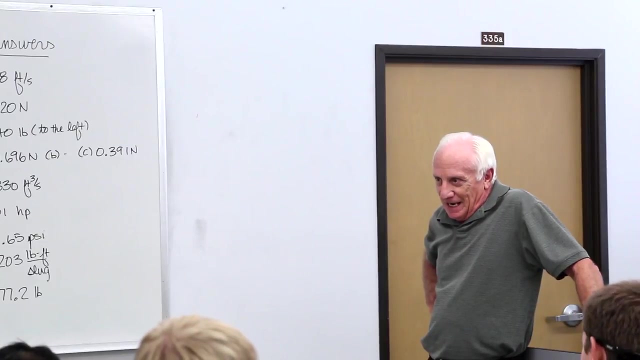 Chapter 5 is applying the Reynolds transport theorem to three most important equations in fluid mechanics. We've done it already now continuity: Okay, so we've done the continuity equation. we did a couple example problems in class and that's the first part of chapter 5,, Homer, Now we're going to do momentum and then we're going. 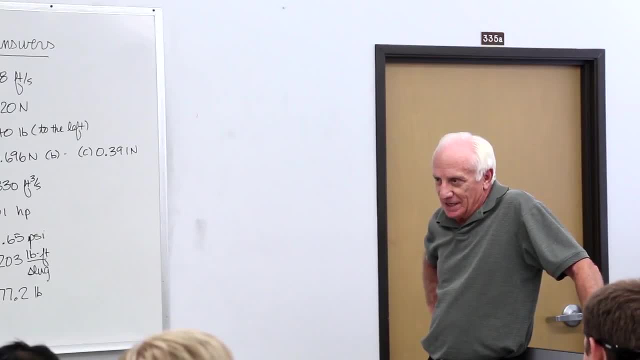 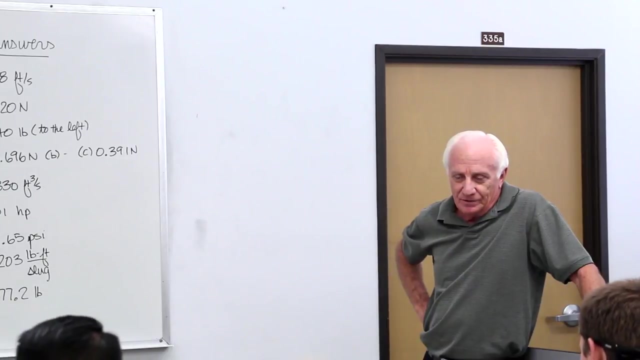 to end up next week, probably Wednesday next week, we'll start at least energy equations, So conservation of mass, then momentum, and then we have energy equations. Alright, in every one of those three equations we go back to the Reynolds transport theorem. in 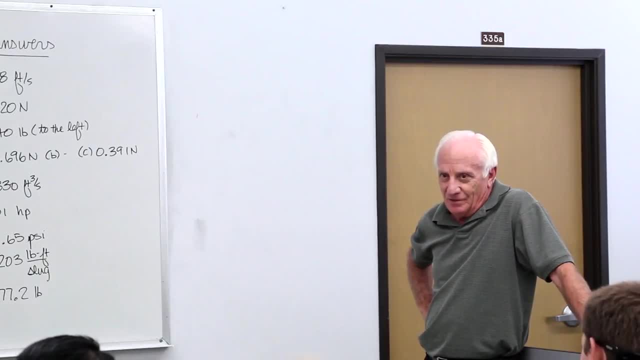 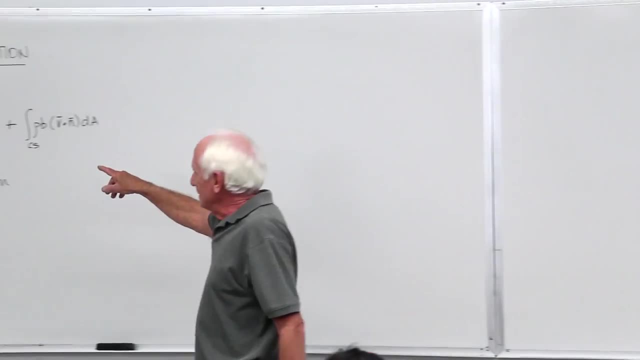 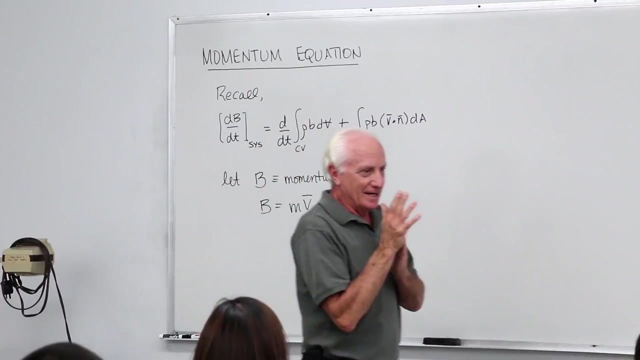 chapter 4, and we start there and we derive the equation from the Reynolds transport theorem. Okay, so we go back. this is the Reynolds transport theorem from the last part of chapter 4.. The left-hand side is the system, the right-hand side is the control line, control surface. 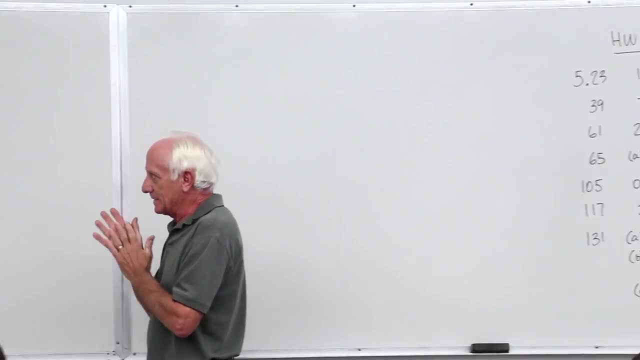 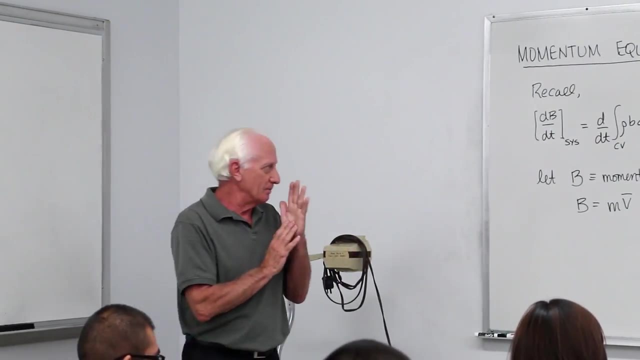 Initially in chapter 5, we're going to do momentum and then we're going to do energy equations And we're going to apply it. we let capital B be the mass And that led to the conservation of mass equation or continuity equation. Now we're going to let capital B 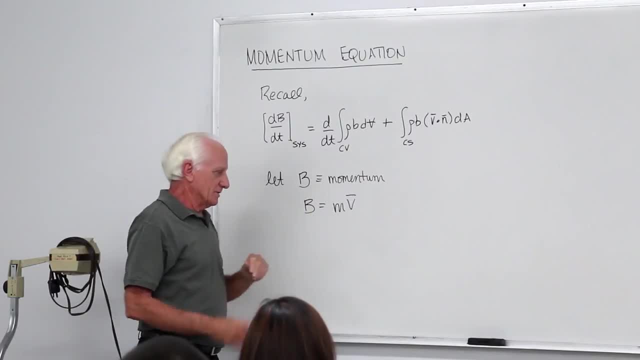 be momentum, and momentum is mass, times, velocity, and little b then? okay, Little b, of course, is momentum. divided by that, mass будет jadi mass, And that's what we call momentum and that's what we're going to use. So we're going to have less our energy, less our energy. 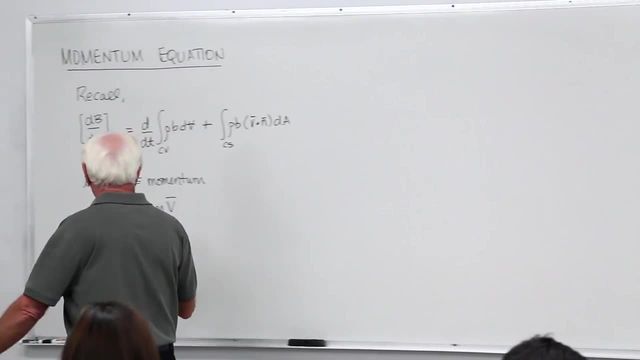 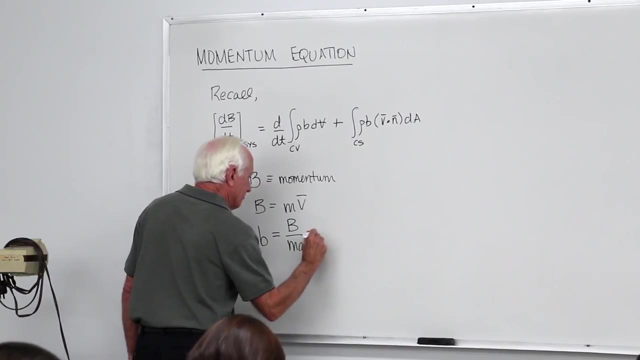 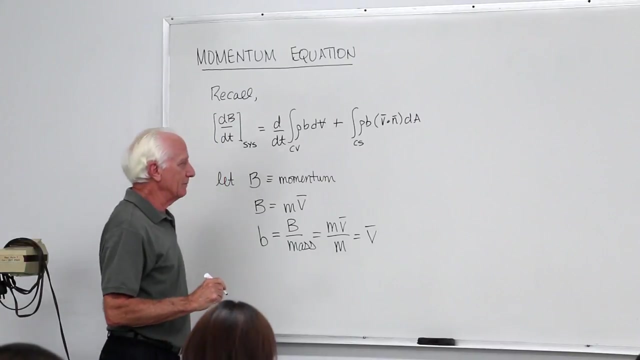 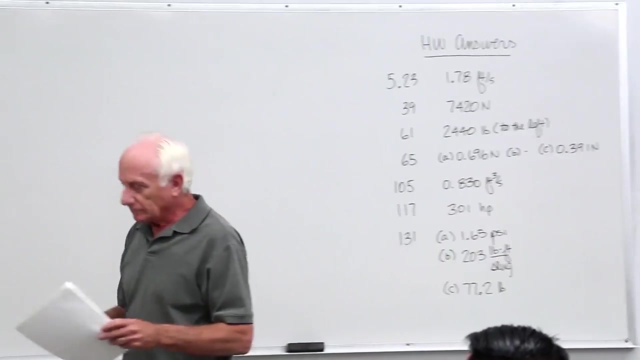 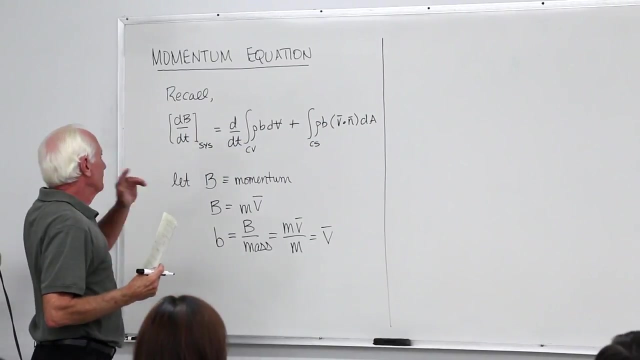 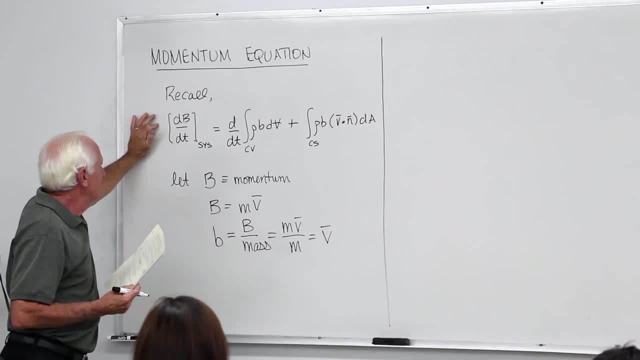 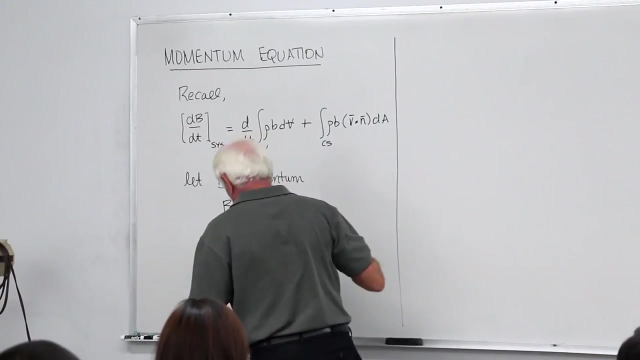 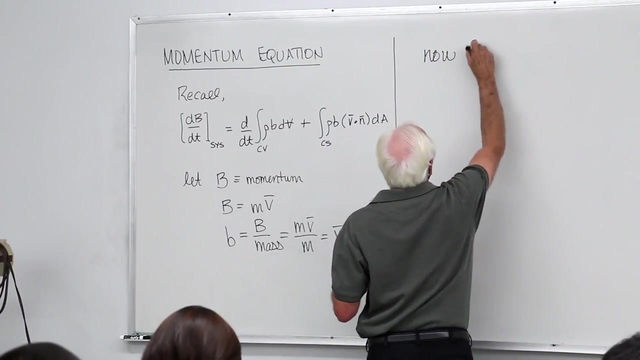 all we know from the system analysis that the change in momentum of a system is equal to the sum of all the forces acting on that system of particles. So the left-hand side, this is a summation of forces that act on that system. So d, b e, t, let's. 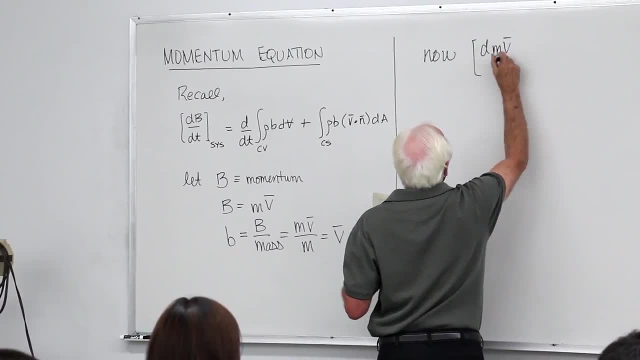 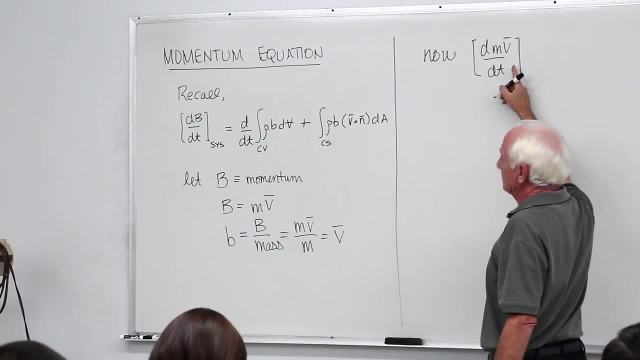 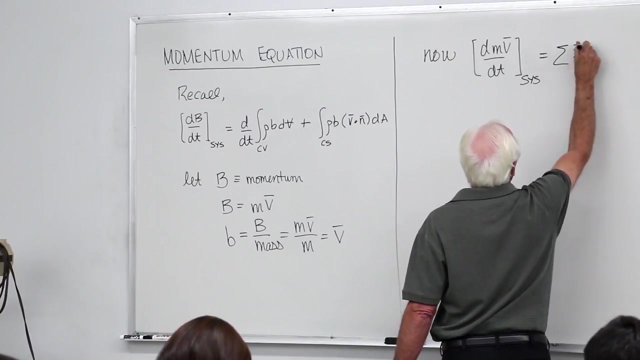 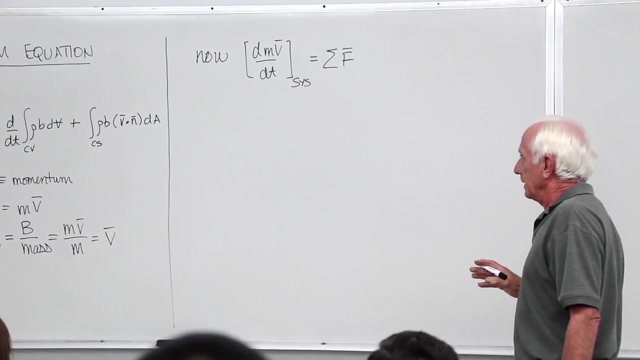 make that the mass times the velocity. So this is the rate of change of momentum with respect to time, or the system is equal to the summation of all the forces that act on that system. That's the system approach. Okay, So the first step is: 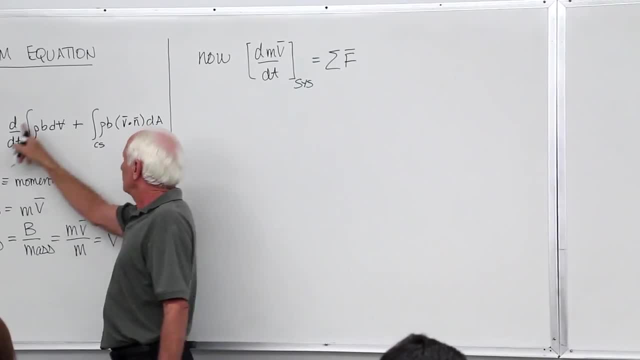 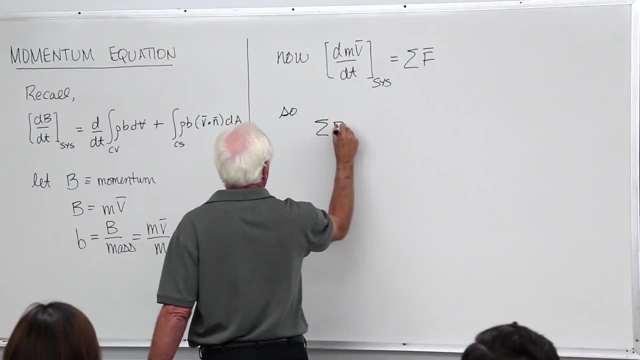 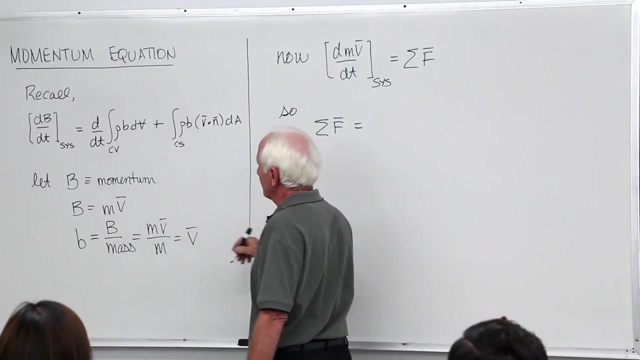 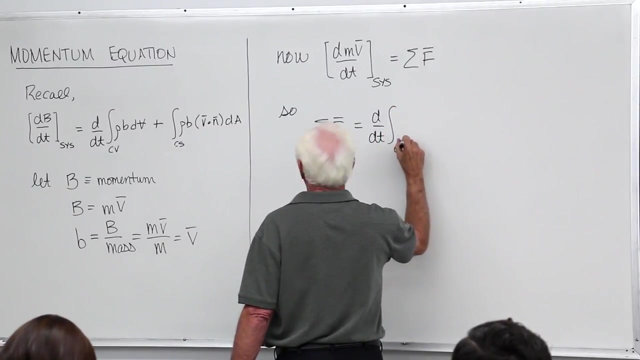 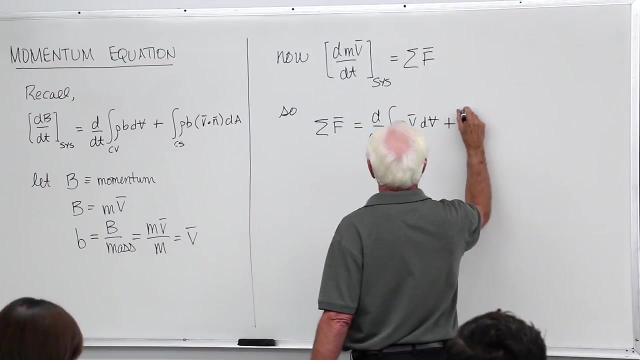 where we see d, b, d, t system, we replace that with the summation of the forces. Vector is equal to now. wherever you see a little b, put the velocity of b, Okay. So we get a velocity of b, Okay. And then we have across the control surface row. 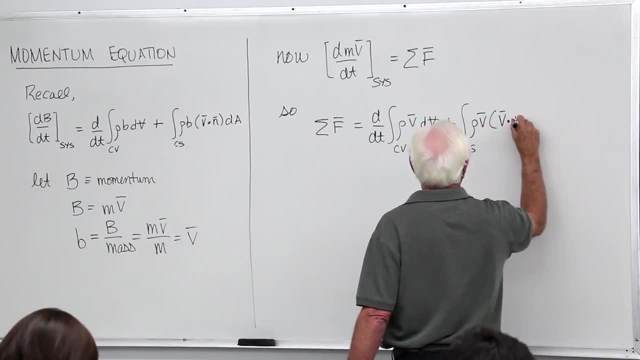 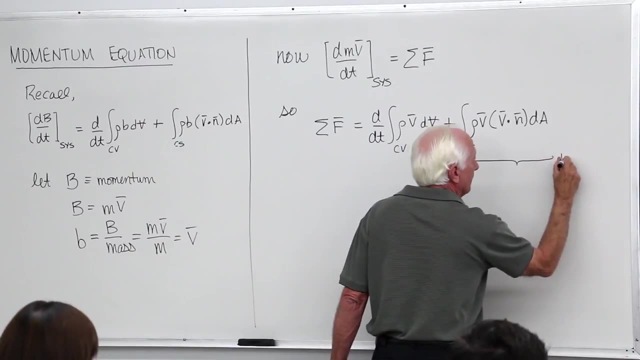 b b, dot n v a Again if uniform velocity, profile v, dot v, dot x will be the same. Okay, And then we have across the control surface row b v, dot n v a, Again if uniform velocity. 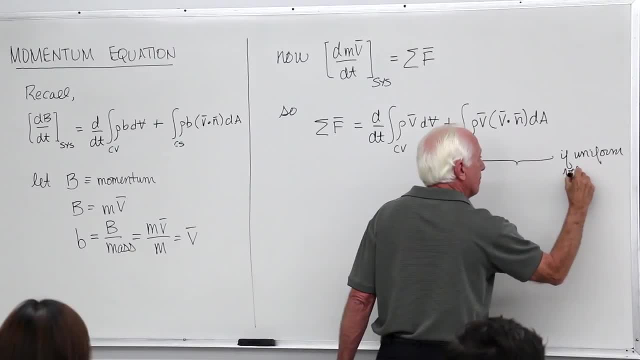 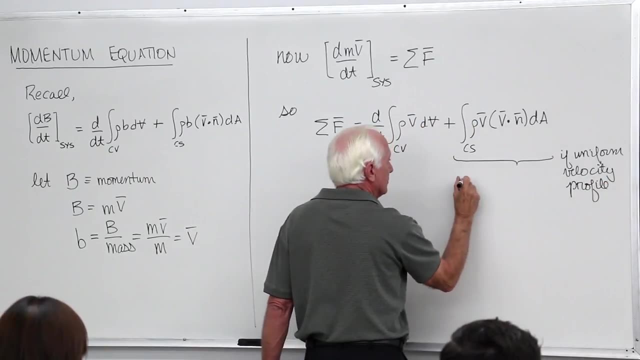 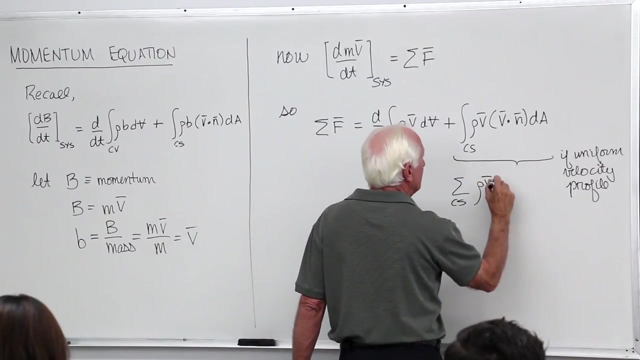 profile. we do the same thing, Right, Right, Yes, Okay, Okay, Okay, Okay. So let's do this one more time. Okay, Okay, All right. this thing simplifies, to summation: over the control surface of Rho V, and this is: 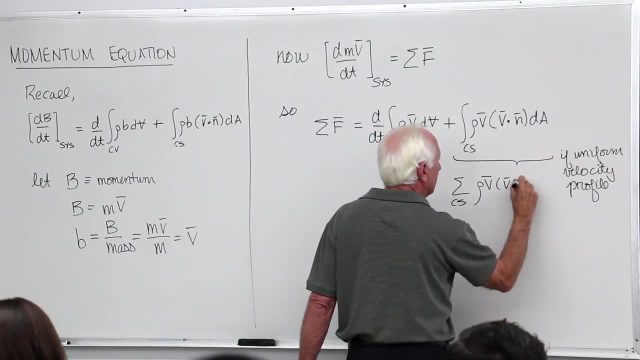 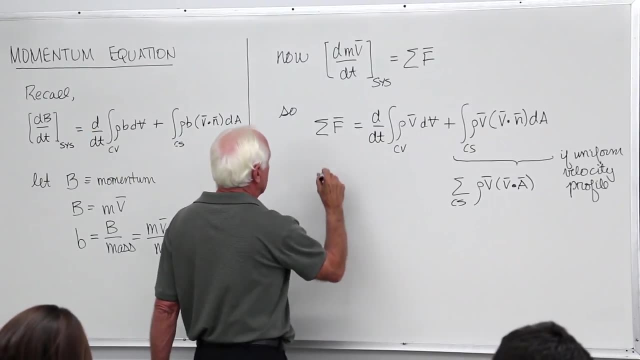 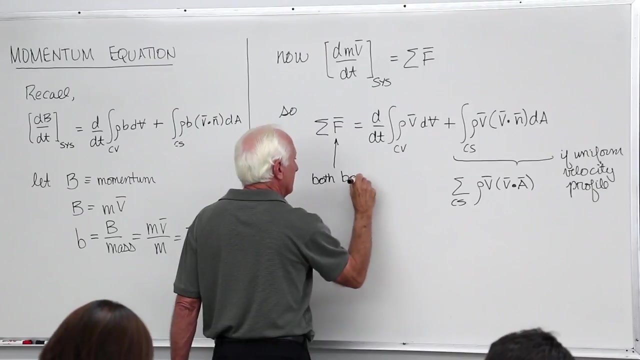 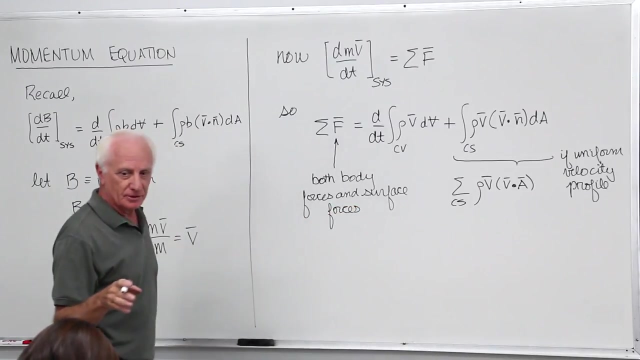 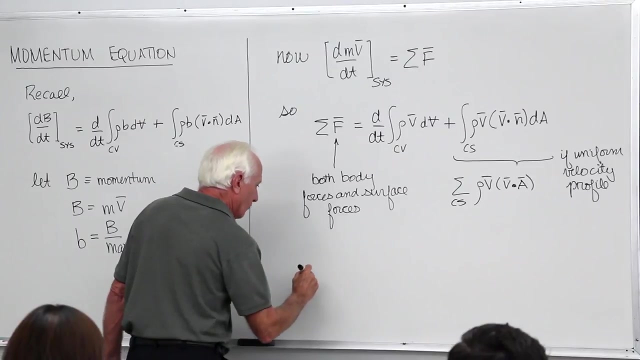 our V dot A And let's see, these forces are both body forces like it's weight, And we call surface forces. If a pressure acts on a surface, that's a surface force. Alright, I'm going to write it down one more time down here, just to keep it in the format. 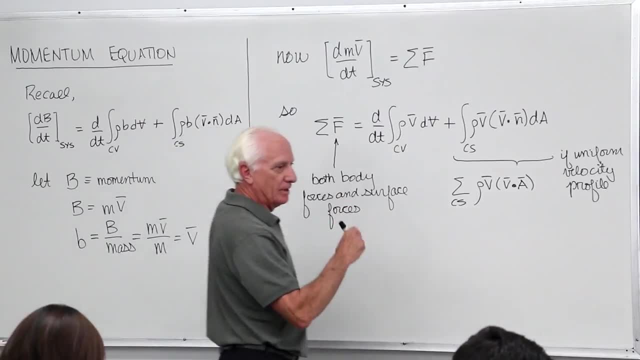 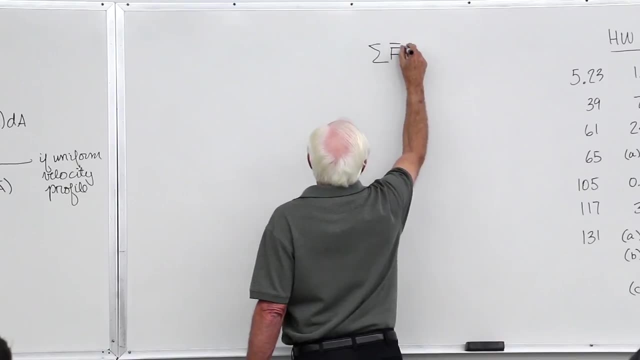 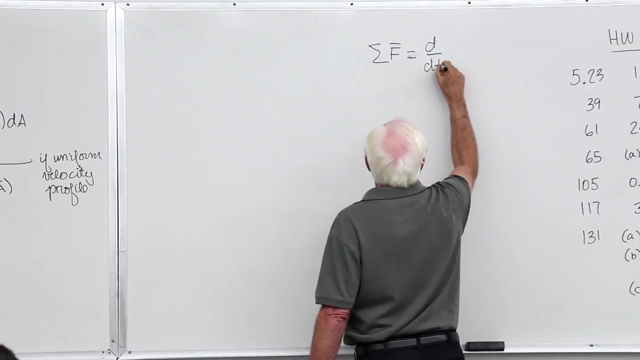 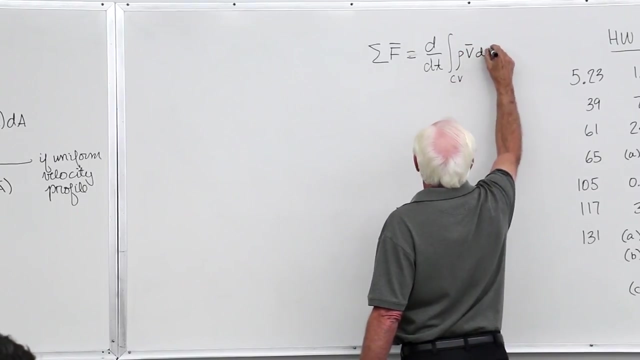 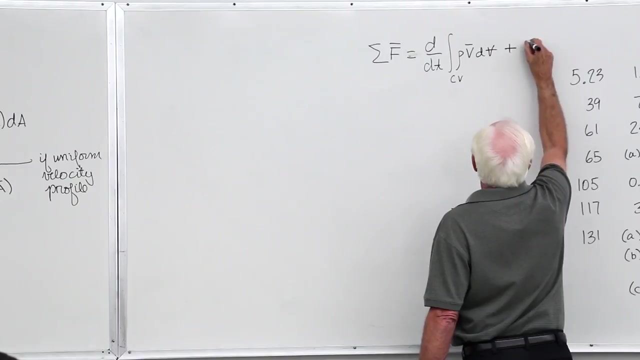 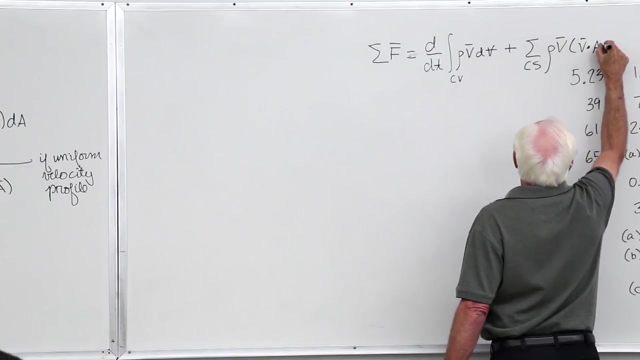 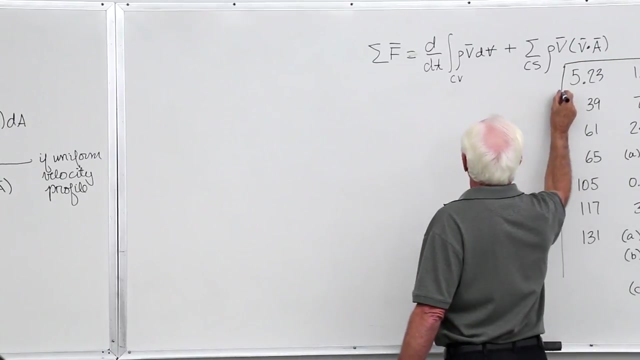 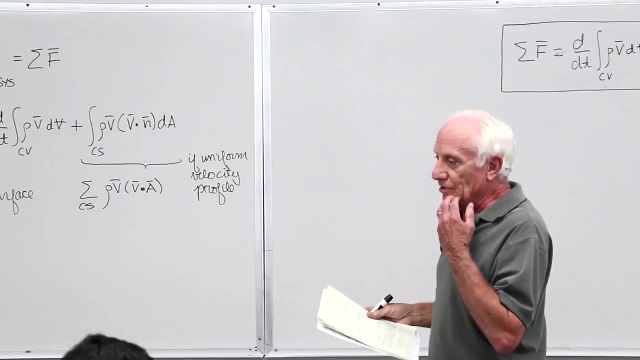 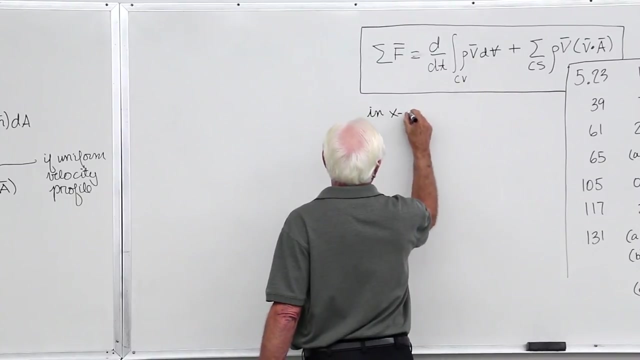 we used today. I think I'll put it over here so we can save it. Now. that's the general form, The vector form. We'll normally deal with the component form of that, so we'll just show you one In the x direction. we have the summation of the forces in the x direction. 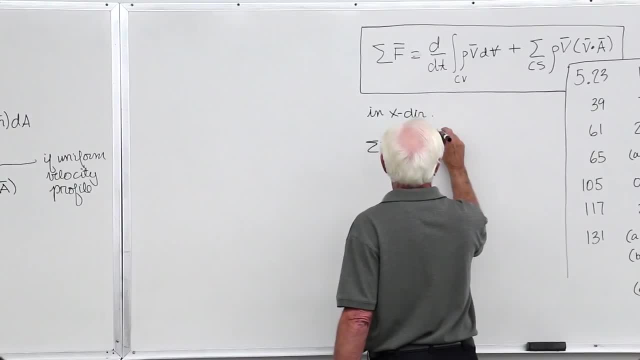 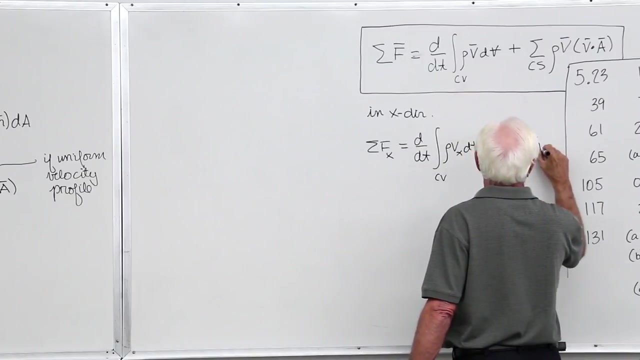 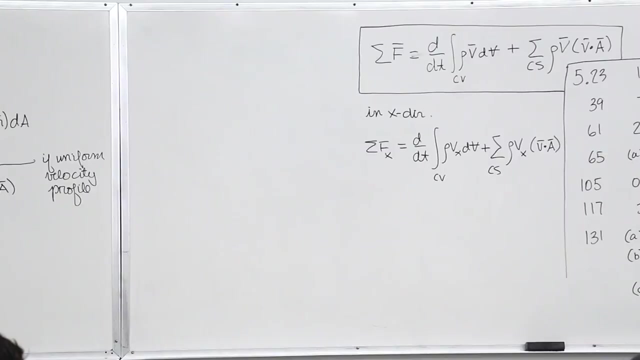 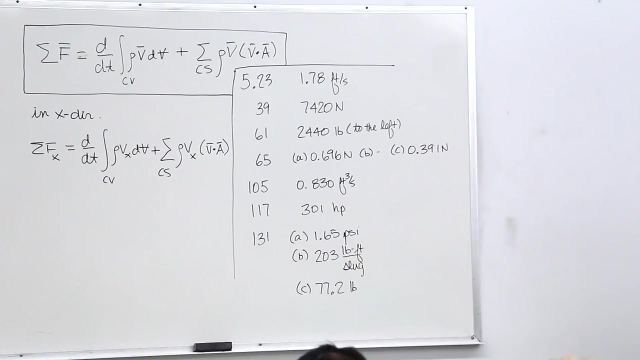 And this would be the velocity in the x direction Plus sum over the control surface, The velocity in the x direction, V dot A, And it would be similar, of course, to the y and the z directions. Okay, so that's the second important equation in chapter five. 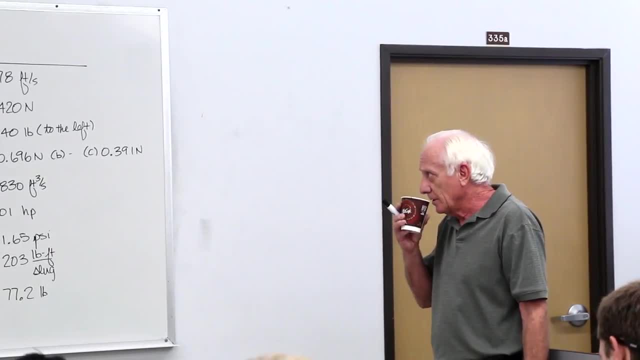 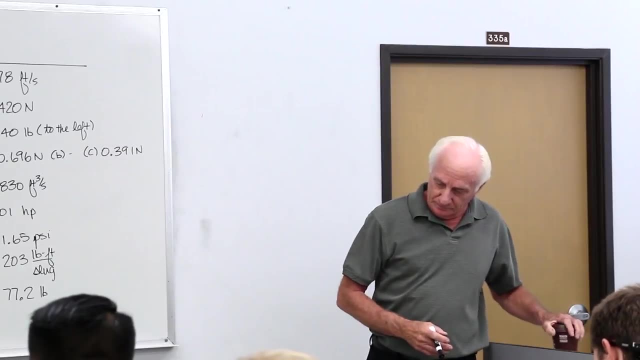 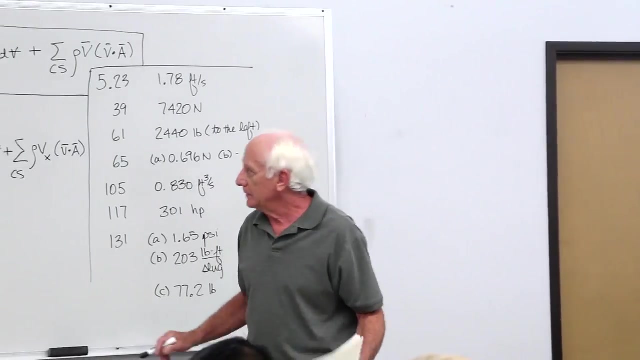 Conservation of mass was the first one, or the continuity equation. This is the second one momentum. Now we can go ahead and look at a simple example of that. Let's put it back over here. I think it's the best place to put it. 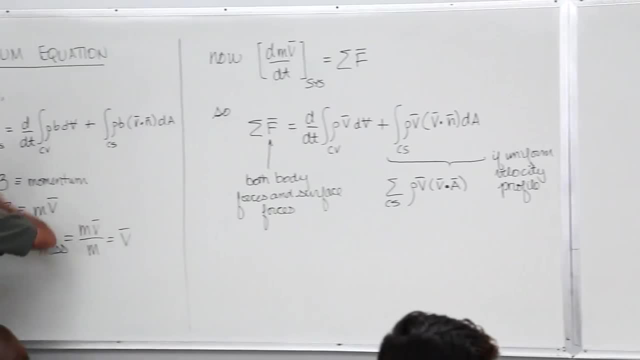 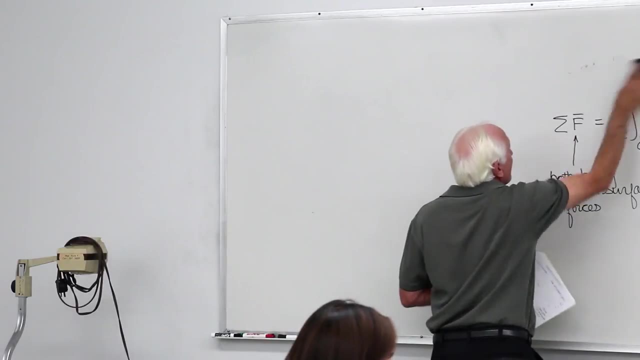 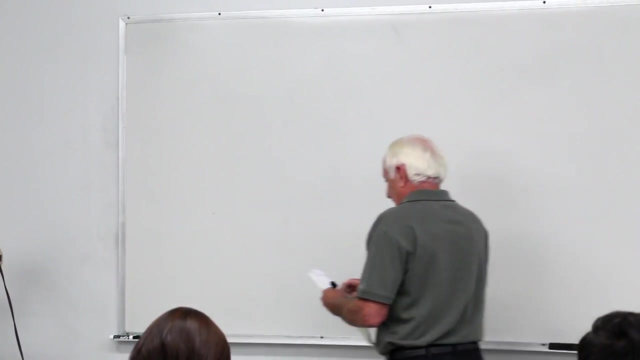 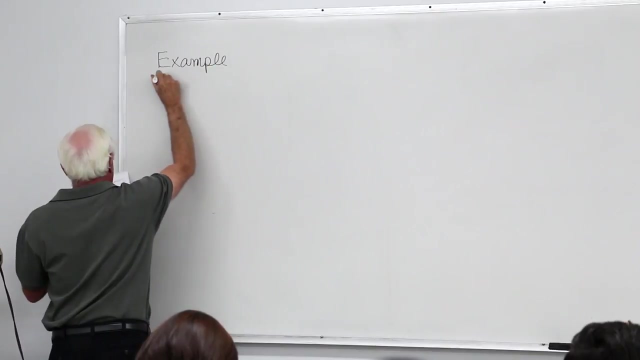 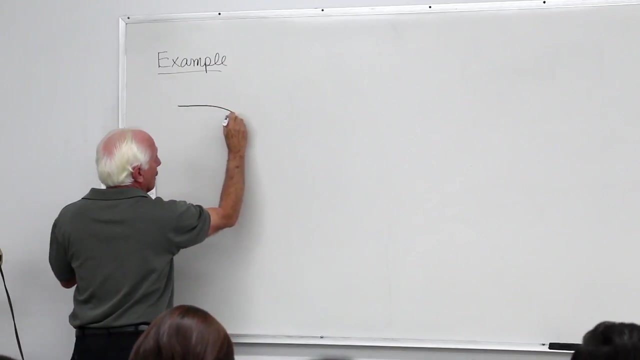 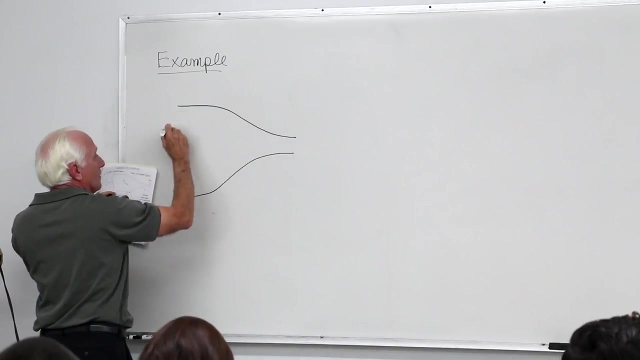 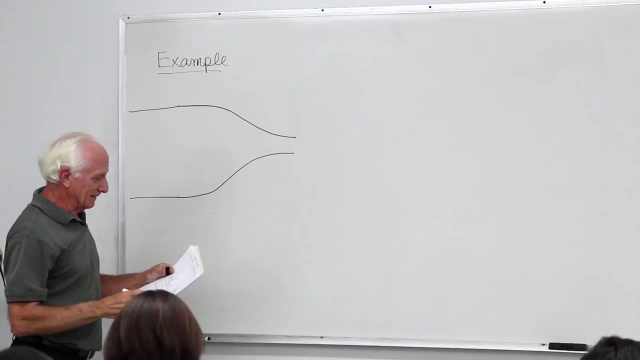 We'll just have more. Okay, Okay, let's see, This is a pipe. Let's just make it like this. Okay, Okay, Okay, Okay, Okay Okay. This is the first one right there, And this pipe goes on. 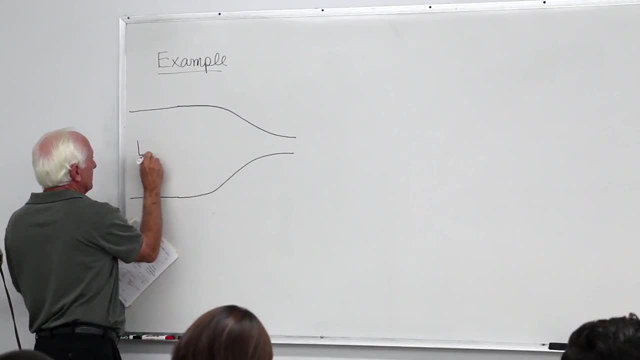 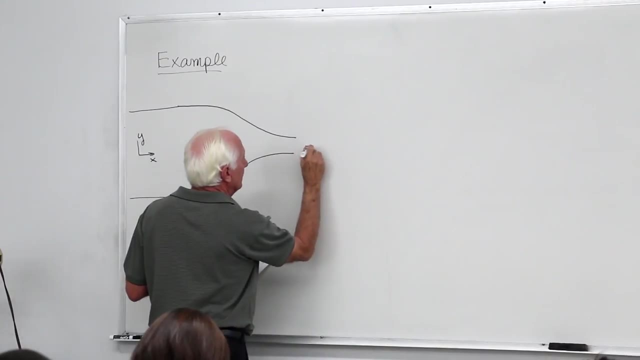 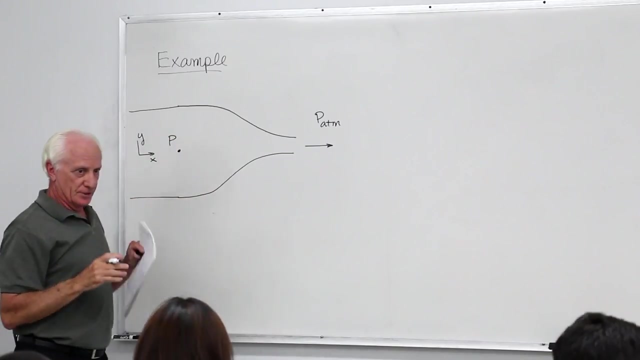 Let me just see if it goes on like that. Let me just see if it goes on like that, And we're going to show the x and y directions. The fluid is leaving here, It's exiting to the atmosphere, But the pressure at this point in the pipe would be P. It's under pressure. it's a pipe under pressure. 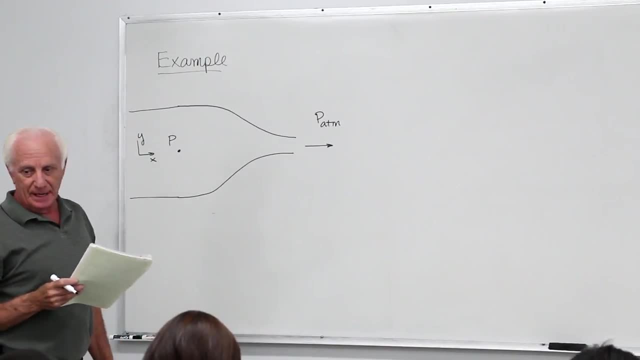 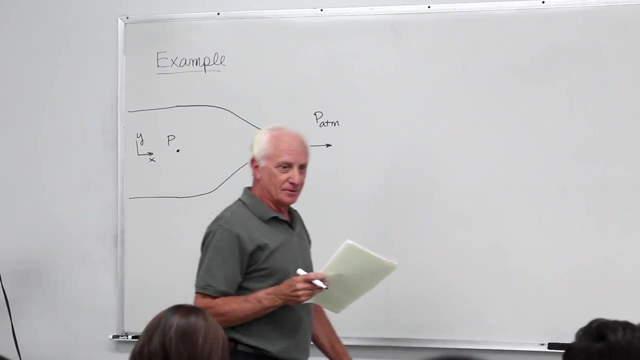 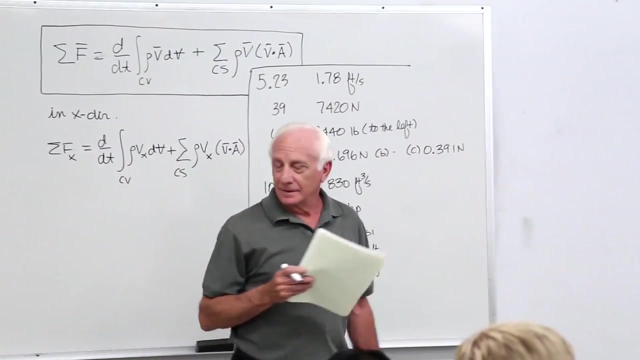 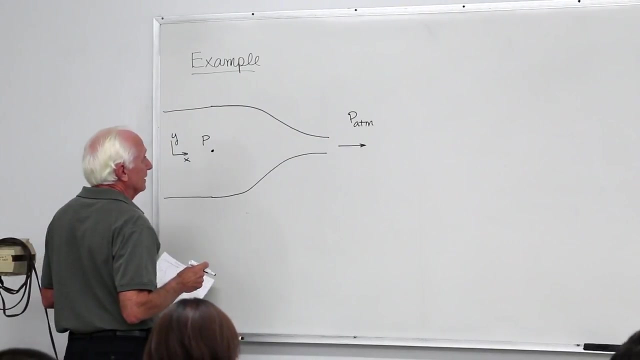 Water comes out through a nozzle. This could be a nozzle in a pipe. This is a nozzle. What's the purpose of a nozzle? The purpose of a nozzle is to accelerate the flow to a higher velocity. Okay, So let's see what else to find here. 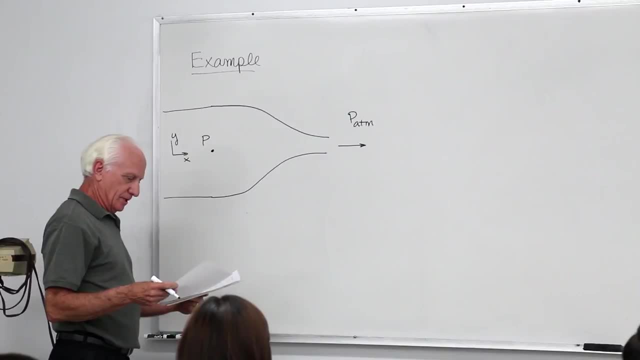 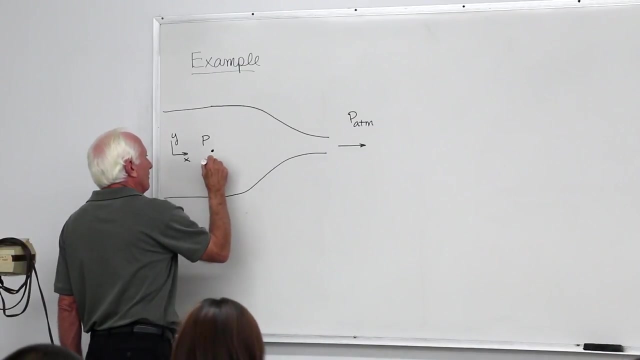 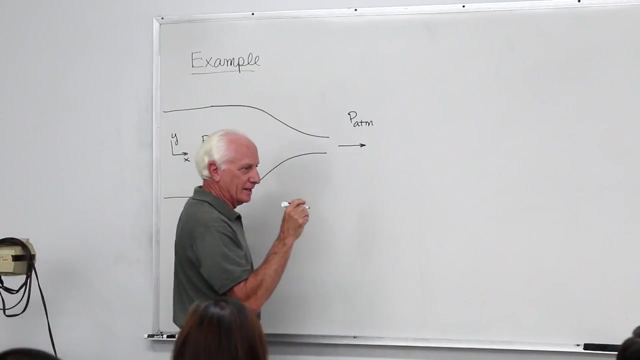 Well, I'm just going to write down the equations that we're going to use for this. Normally, we want to put a location on it: Where's point one and point two? Okay, Point one, Point two: Just outside the nozzle, Outside. 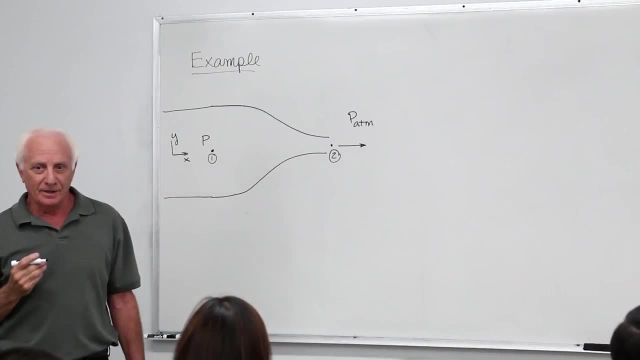 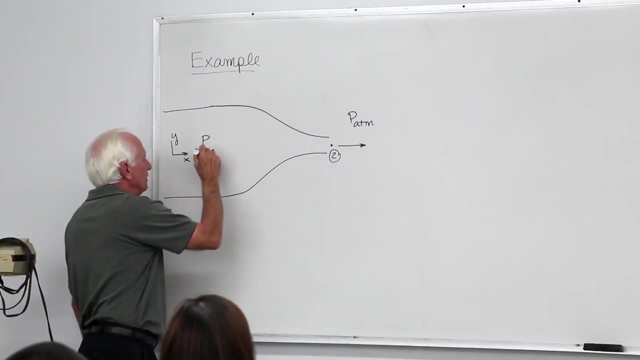 Why? Well, one of the reasons why is, I know, the pressure there. It's zero atmosphere. Okay, Point one and point two. This is P1.. That's P atmosphere over there. I'm going to call this area A1.. 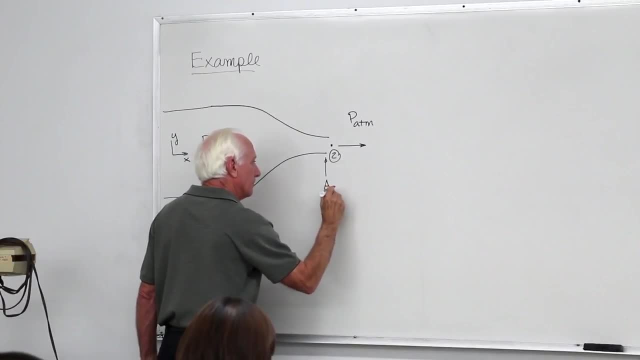 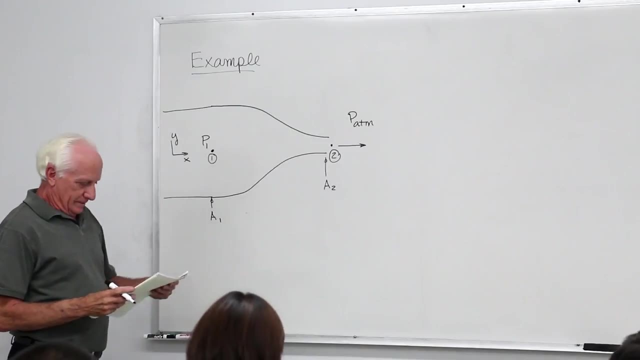 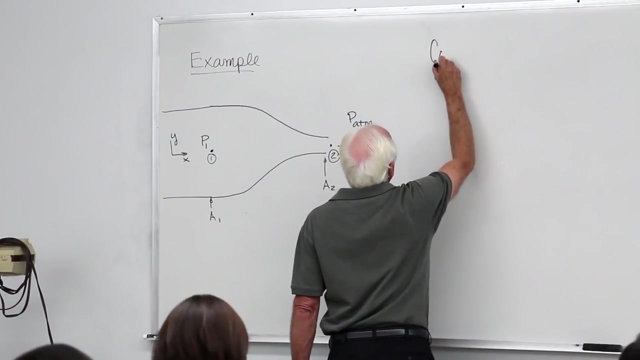 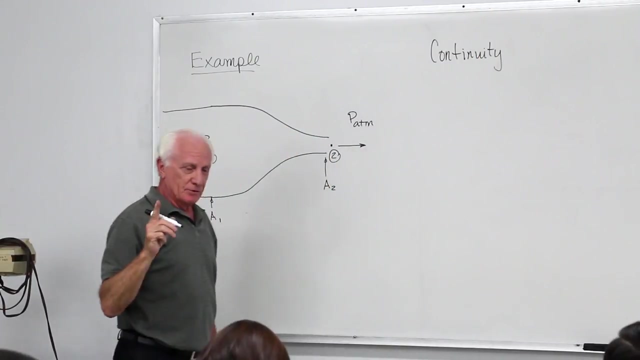 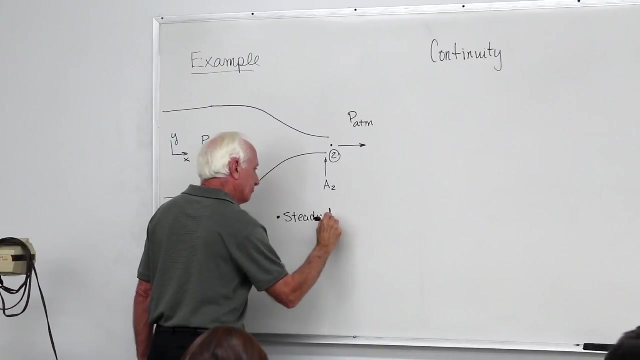 And this area I'll call A2.. Okay, All right. All right, Let's take first of all continuity. Now we're going to make some assumptions. First assumption: steady flow. Okay, Nothing's varying with time. 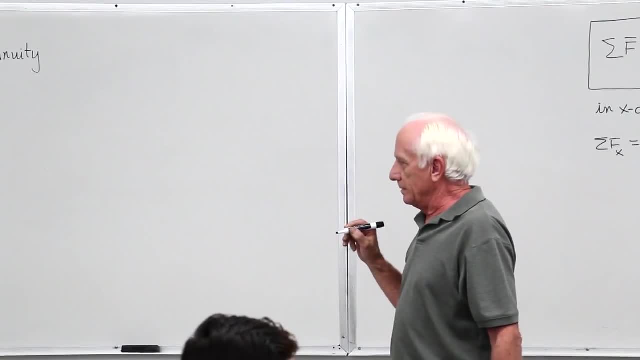 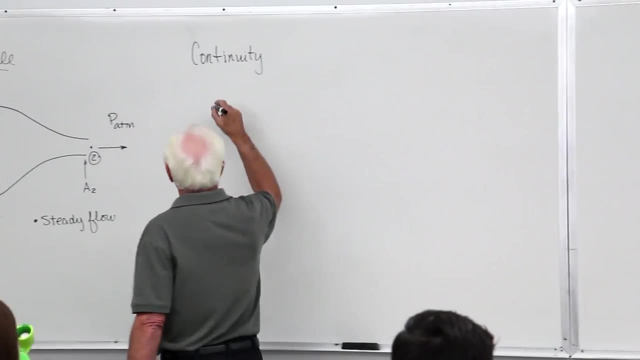 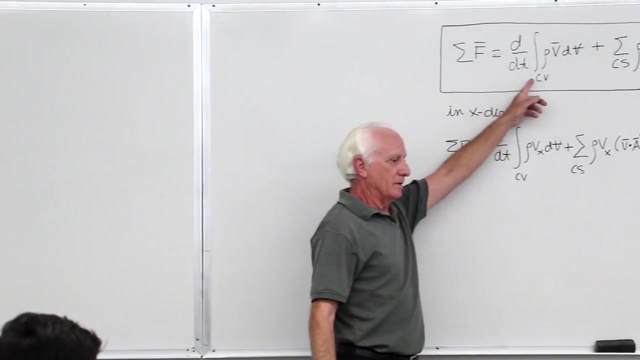 So steady flow means the concentration of mass. The mass flow rate that comes in at one must go out at two. Okay, There's no storage. because nothing changes with time, Here's storage. If nothing changes with time, then that term goes to zero. 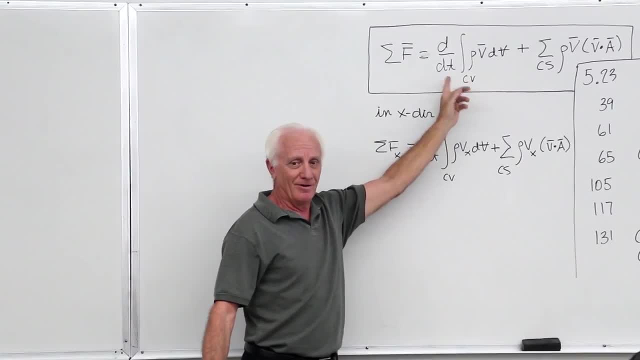 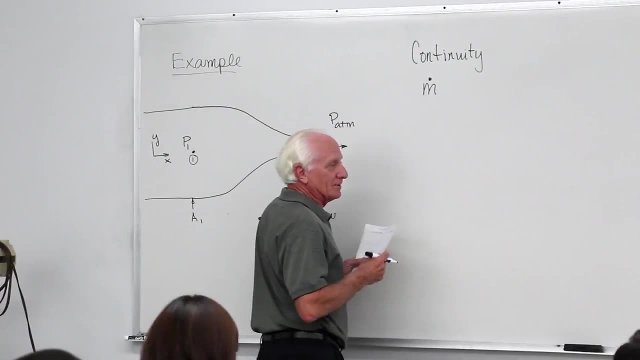 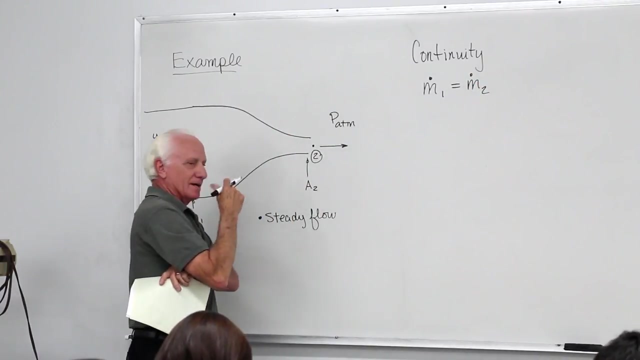 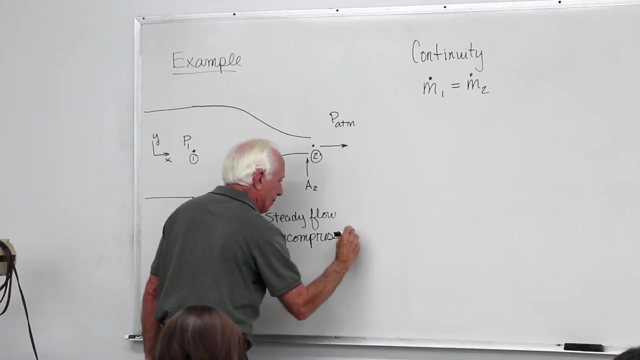 Okay, It doesn't matter whether it's mass momentum or energy. d dt of anything is zero Steady flow. That means the mass flow rate that comes in equals the mass flow rate that goes out. Okay, Now we're going to say incompressible. 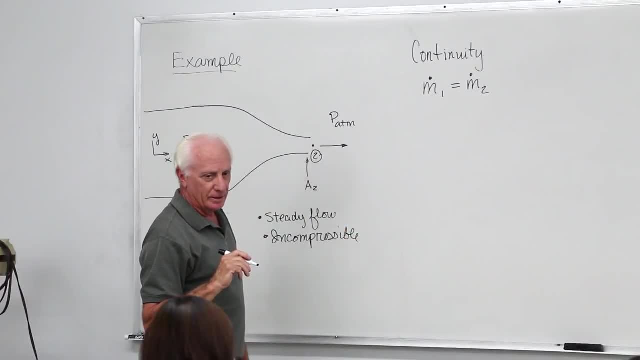 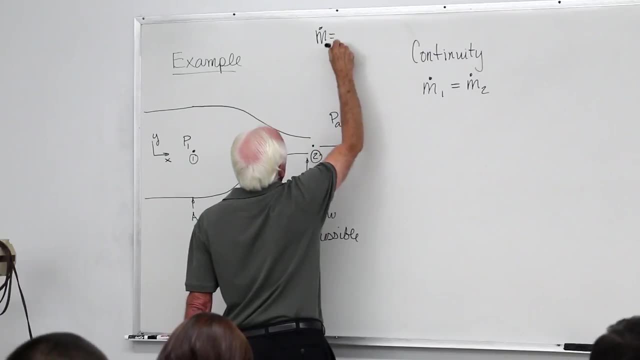 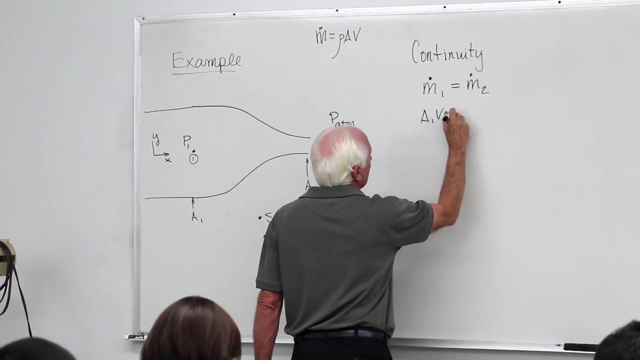 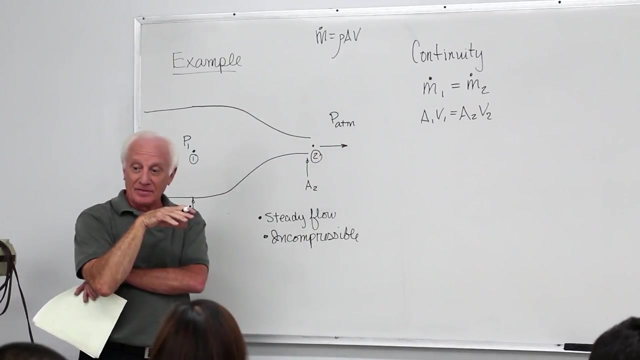 Rho is constant. Rho one equals rho two. And what's m dot? m dot equals rho ab. So the rho's cancel out. We have a one, b one equal a, two, b two. Obviously, the areas are not the same here. 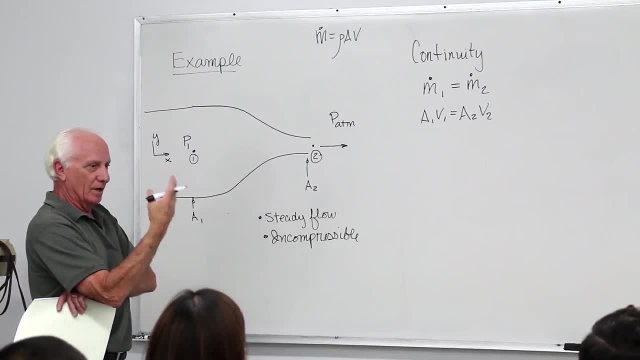 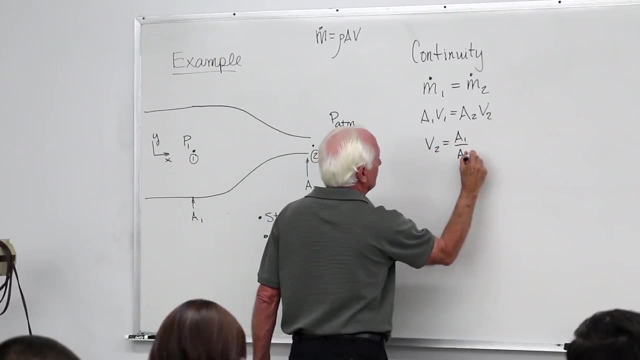 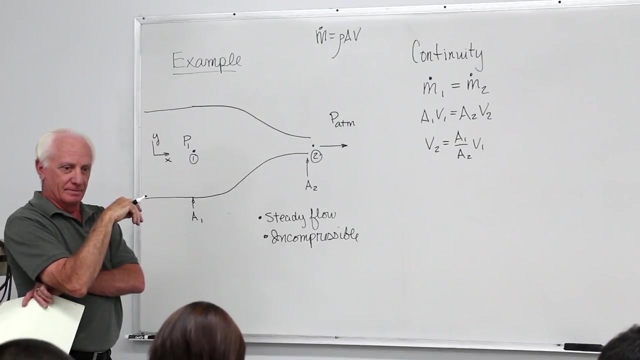 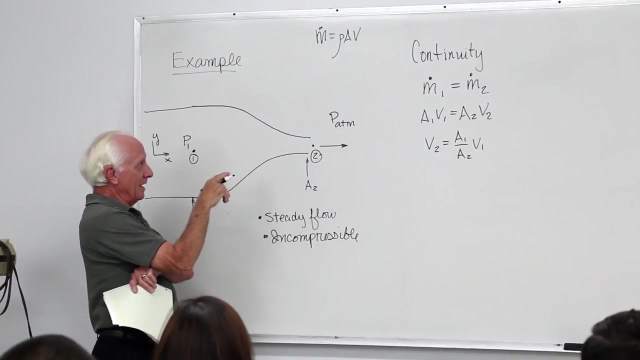 So if you know v one, or let's say you know v one and you want to find b two, then b two equals a one over a two, b one. Those are all from conservation of mass. That means since a one is bigger than a two, obviously the velocity at two is going to. 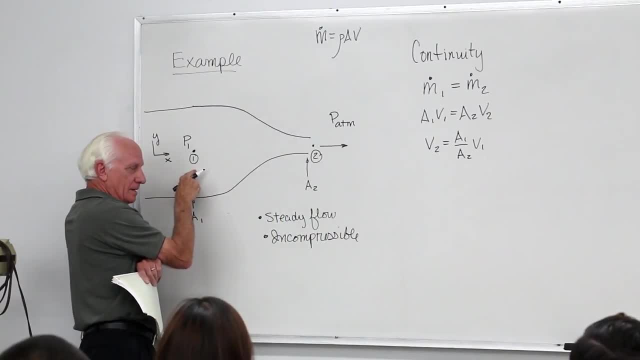 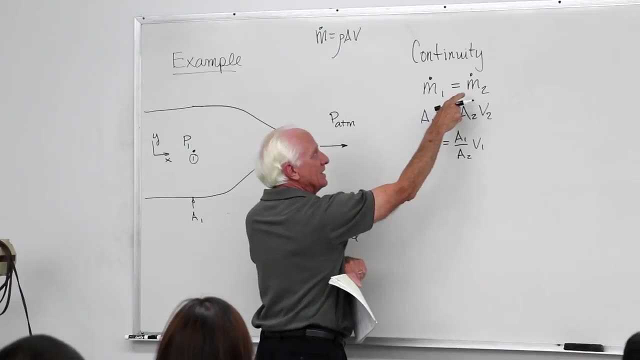 be bigger than the velocity at one, But the volumetric flow rate at two is the same as the volumetric flow rate at one, And the mass flow rate at two equals the mass flow rate at one. Okay, So those are the three equations you got. 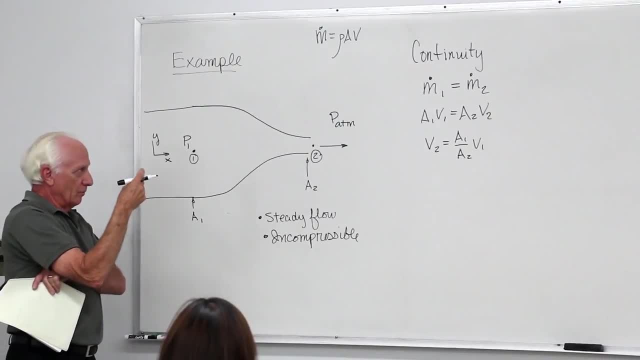 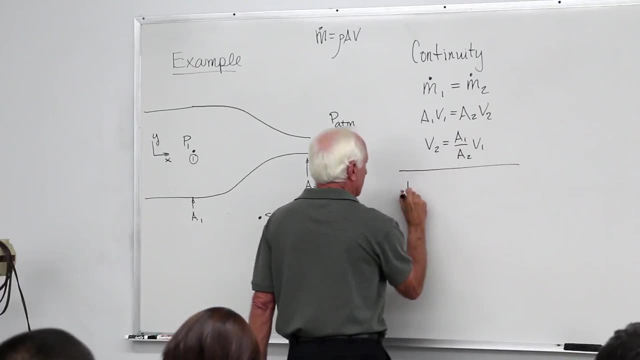 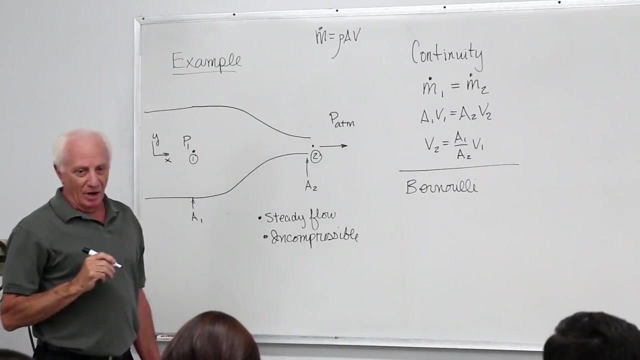 One is the mass flow rate, One is the volumetric flow rate And one is the velocity. Okay, Now let's go to Bernoulli's Bernoulli equation: From where to where? One to two, obviously, Okay. 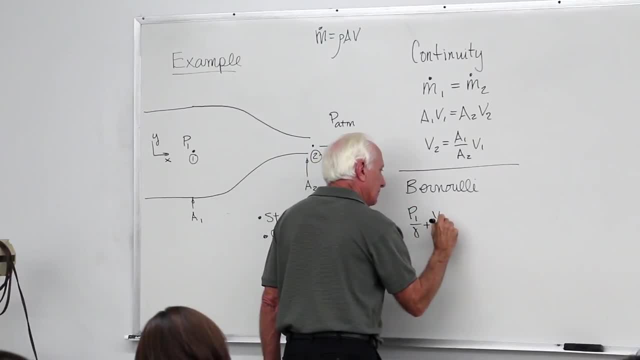 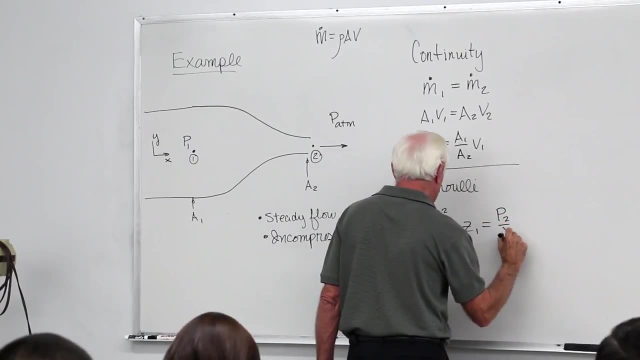 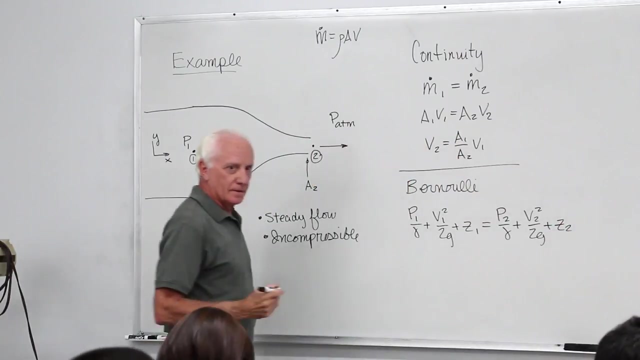 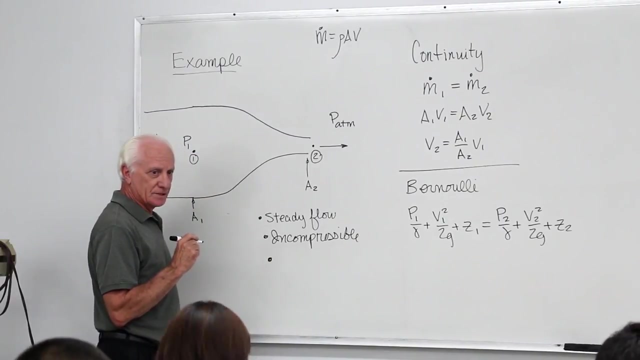 The head form: P one over gamma, v one squared over two, g and z one. Make an assumption. now, if I use that equation Number one, it's inviscid, which means no viscosity, neglect, viscosity. Inviscid means neglect, viscosity. 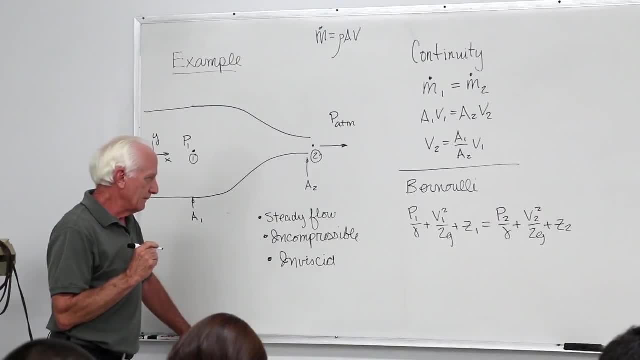 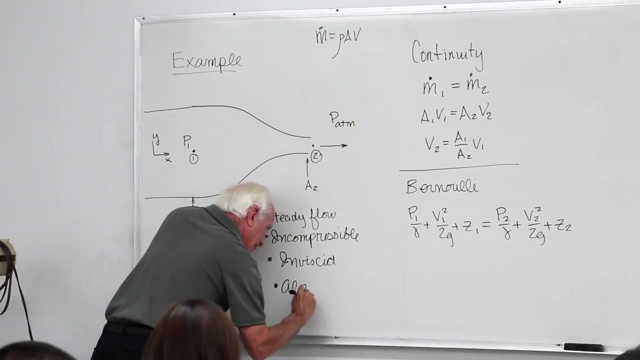 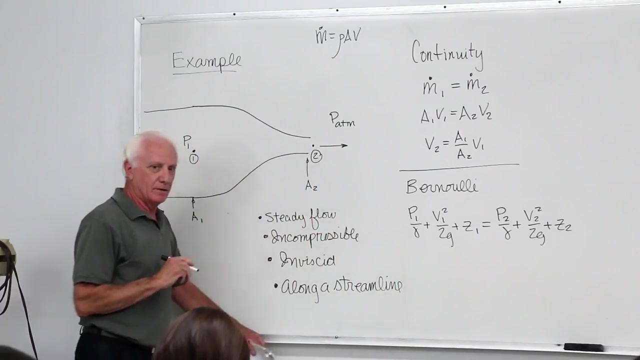 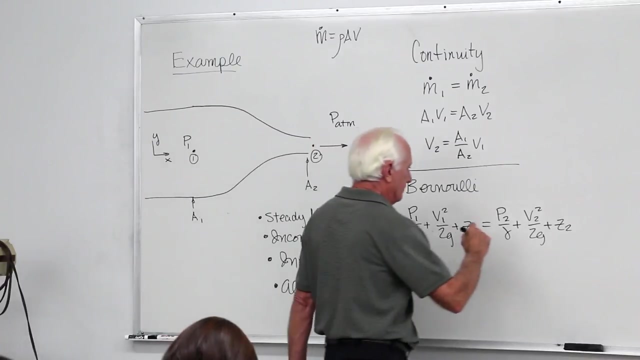 It means neglect, viscosity or viscous effects. Number two: if you use Bernoulli's, it has to be along a streamline. Okay, So there are four assumptions. There's Bernoulli, P, two is zero. Okay, Got it. 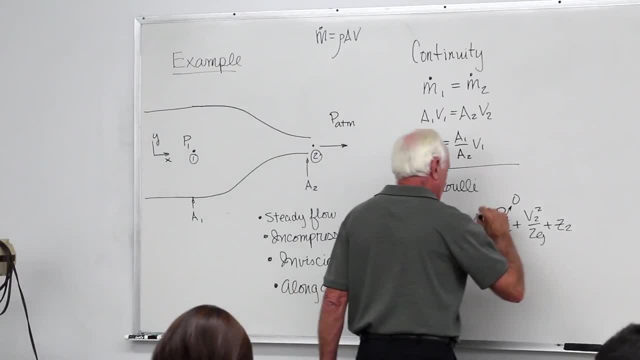 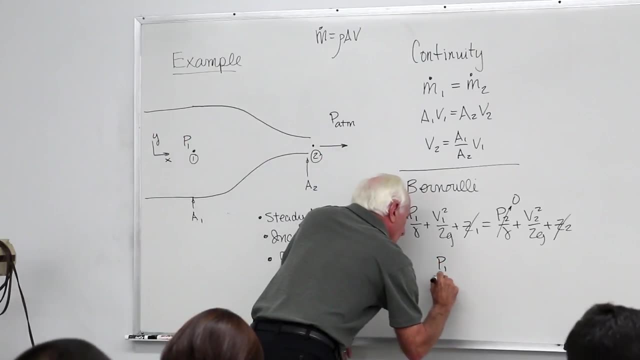 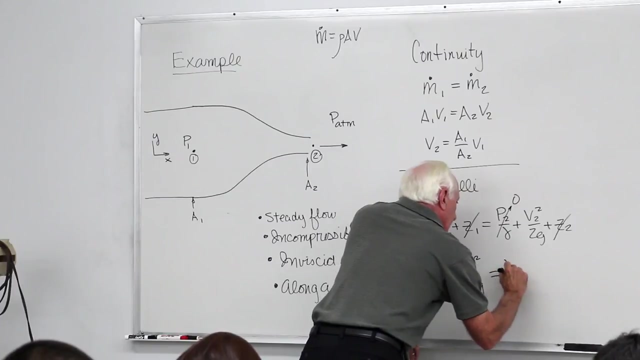 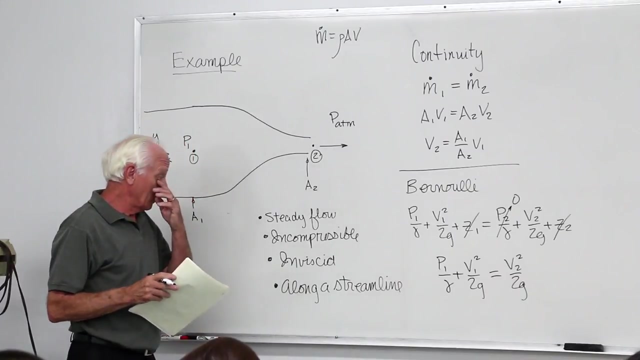 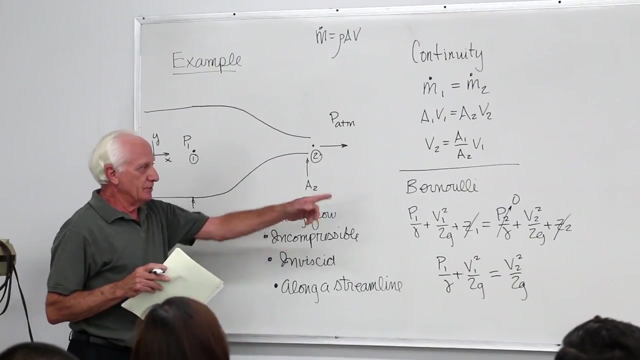 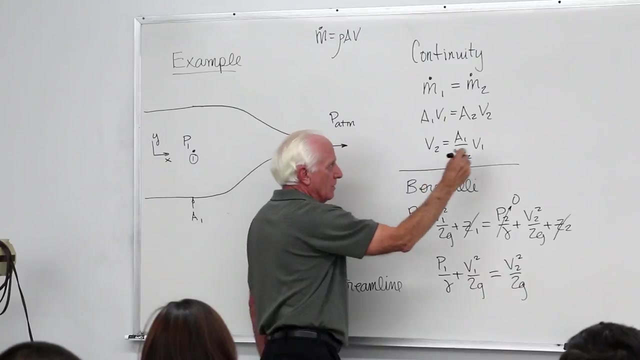 Z1 equals Z2.. Okay, There's Bernoulli's P1 over gamma. V1 squared over 2G equal V2 squared over 2G. If you want, you can combine these two guys together, because here's V2 in terms of V1 right here, So I could put this guy in here for V2.. So 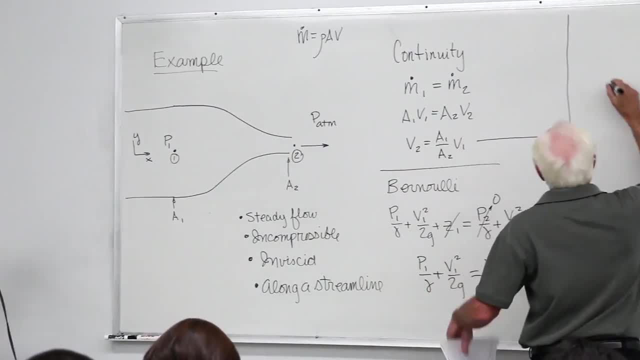 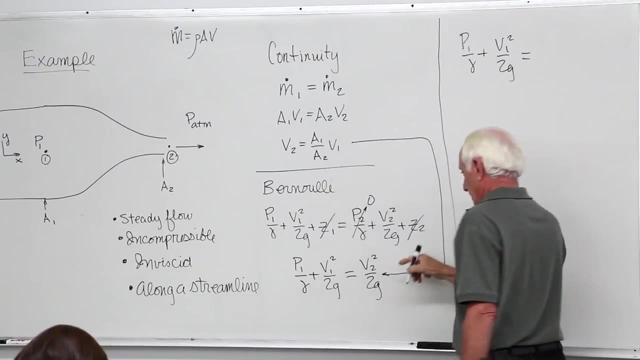 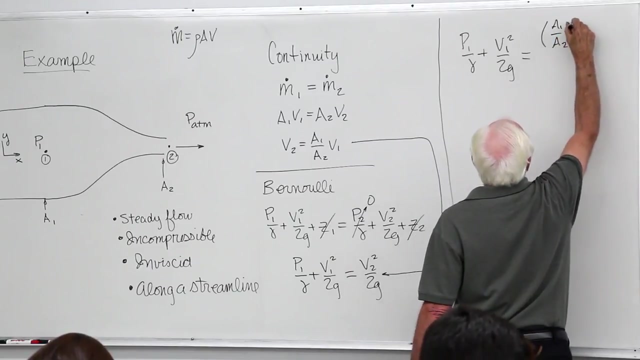 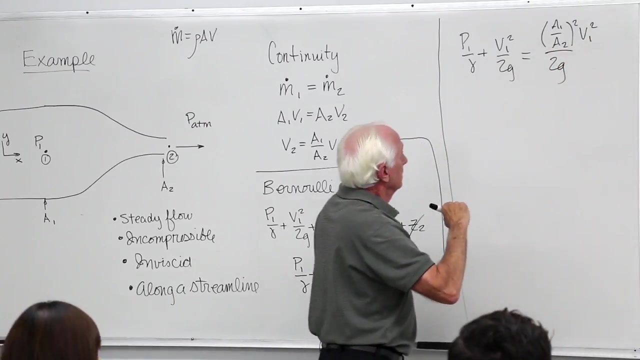 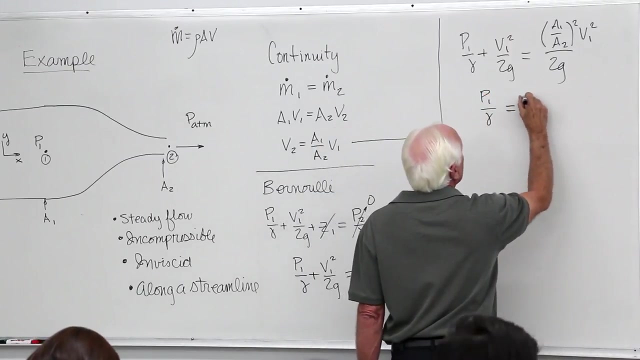 I'll go ahead and do that: P1 over gamma plus V1 squared over 2G, equal- okay, square V2.. There it is: A1 over A2 squared times V1 squared divided by 2G- Okay, P1 over gamma is equal to V1. 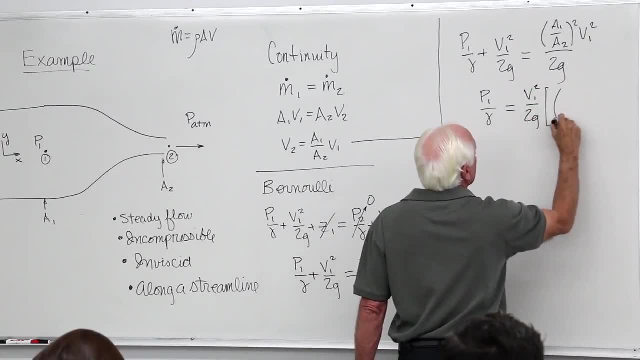 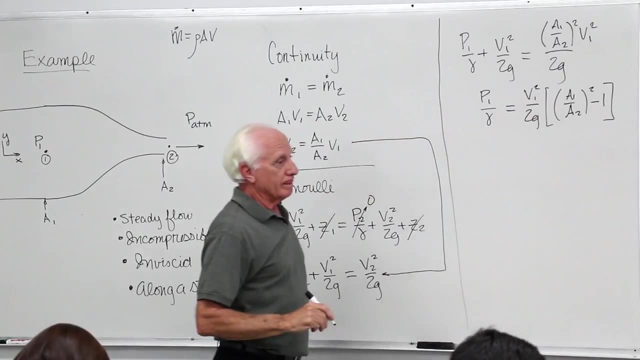 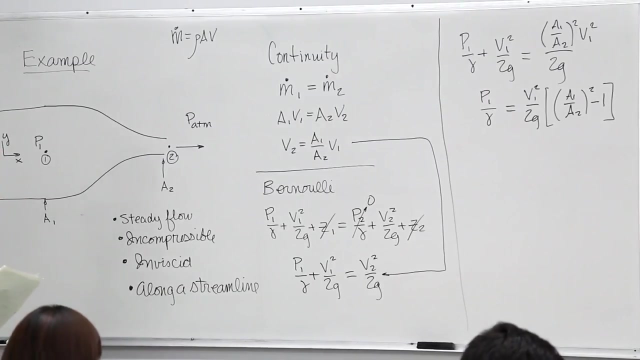 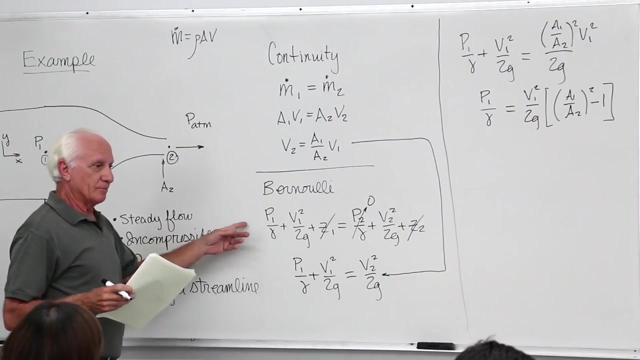 squared over 2G. Quantity A1 over A2, squared minus 1.. That's combining continuity along with Bernoulli's P1 is a high pressure, of course, in the P atmosphere as well. What would we ask to find? 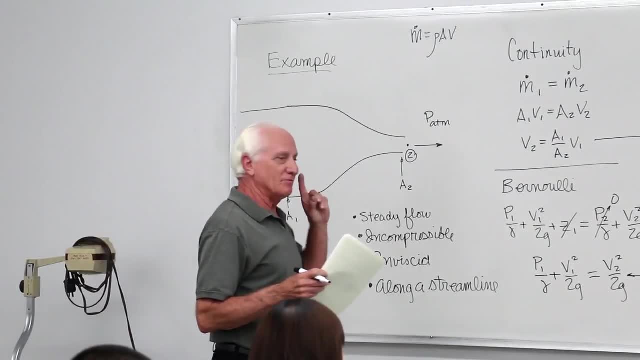 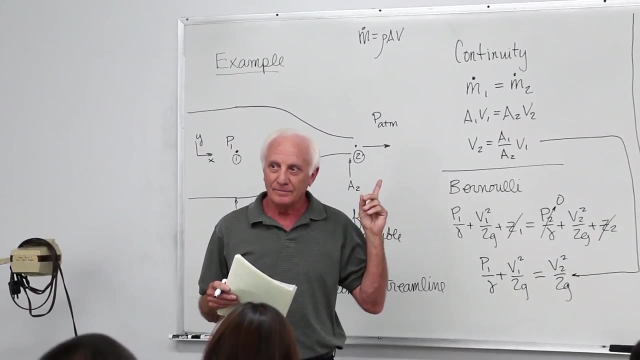 P1?? No, Okay, Thank you. You'd be given one of those two. Either I tell you the flow rate is 50 gallons per minute, you can find V1. Or I tell you the pressure here is 55 PSIG. 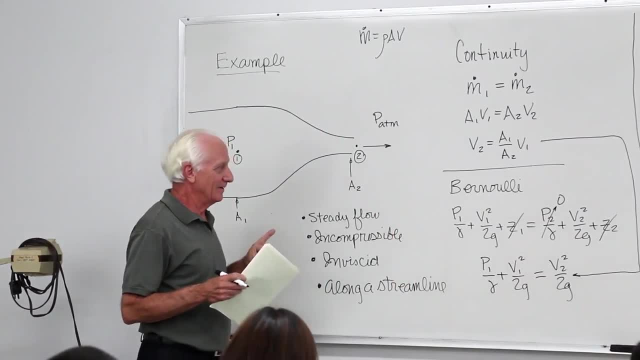 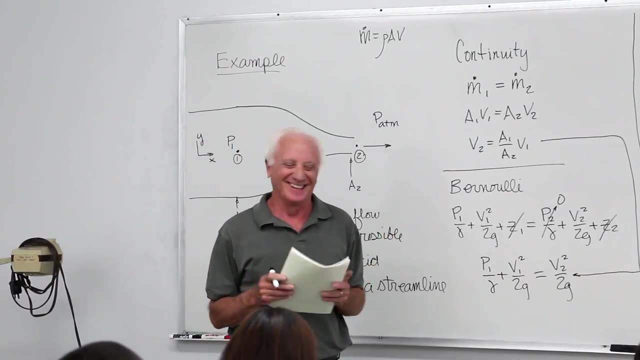 But you've got to be given one. So, but sorry for this problem. what do we ask? You're asked to do nothing except listen to me up here on the board. No, I'm just going over what kind of equation you're going to get. 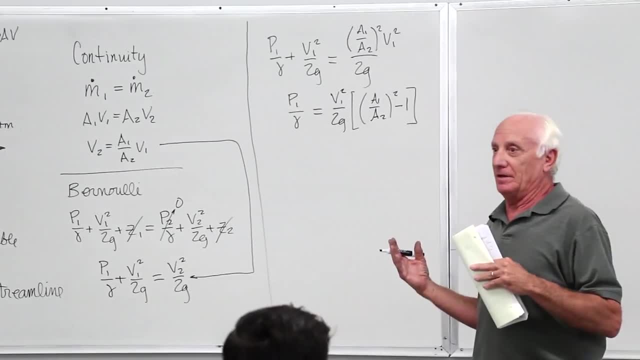 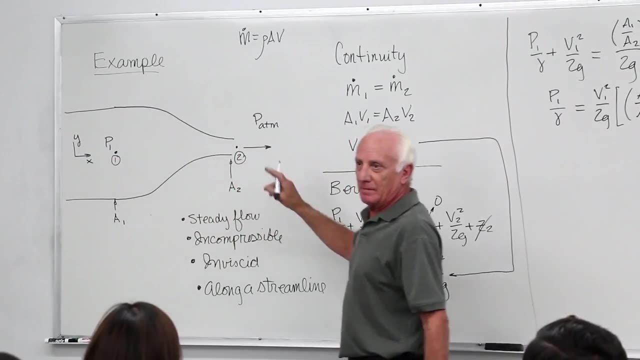 We'll talk about the equation that you could use in a problem like this, And I, when I'm done, typically what you're asked for. I'm not going to solve for anything. You can be given P1 and ask for the mass flow rate out of there. You could be given the. 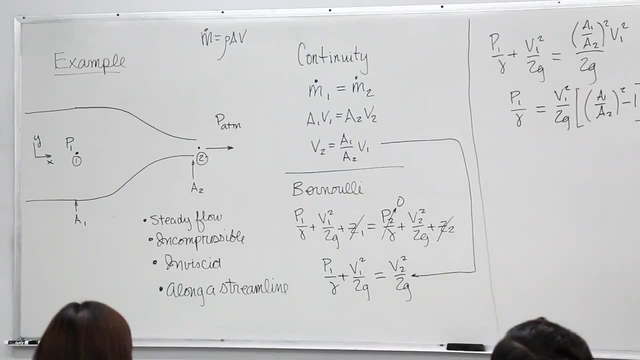 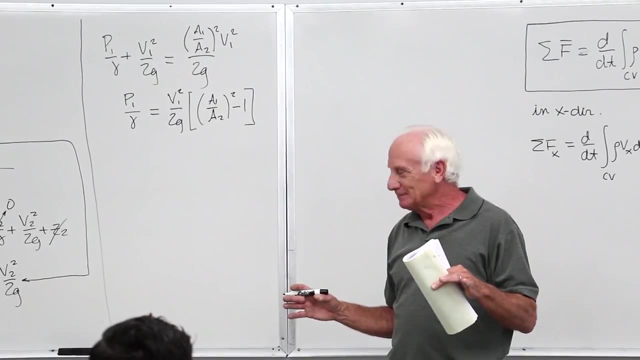 volumetric flow rate and ask for P1, all right, But I'm not asking for anything. Just I'm showing you what equations are in your library to use, Because on an exam you've got a library to use, You've got a library. It's partly in your head and partly on your paper sheet. 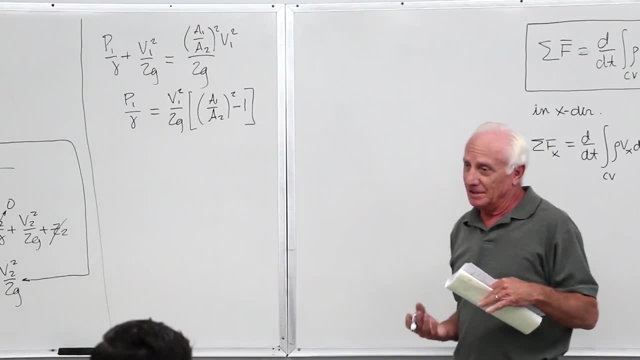 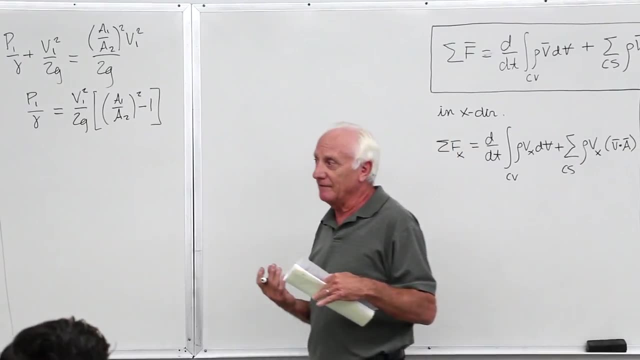 You've got to figure out what in your library you can use to solve that problem. So you better start writing stuff down. If you don't know where you're going, then start writing stuff down. Look at it for a while. That's the key. If you don't know where you're going, 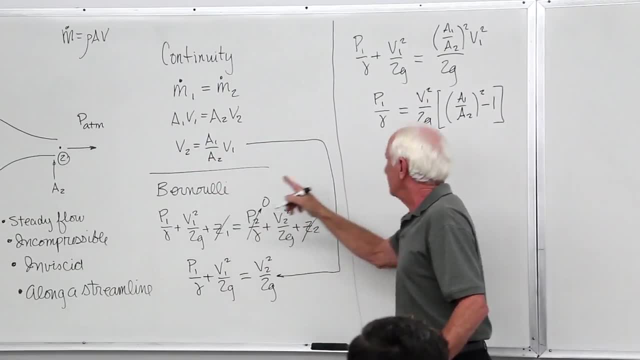 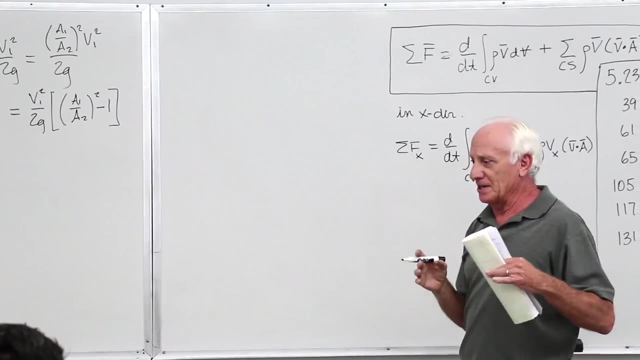 start writing down momentum and see if something jumps out at you on an exam. Some people say, oh, you're getting stressed and don't think straight. Well, I'll tell you the way you think straight is: start putting stuff down on paper and looking at it. 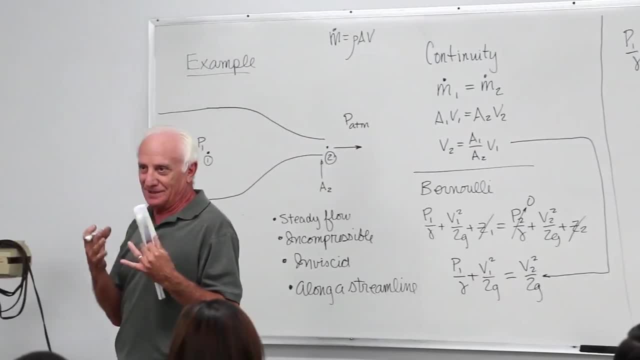 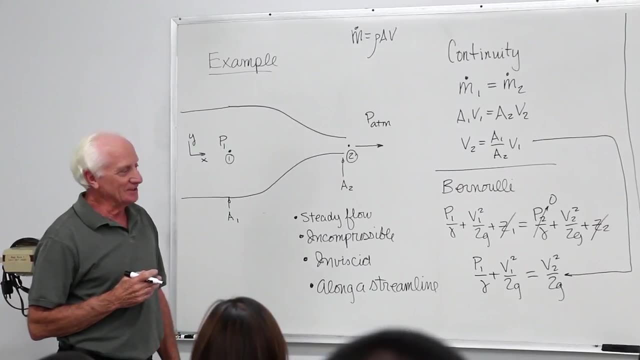 That takes some stress off your mind. So, yeah, that's good to do. I know it takes a minute or two, but if it saves you, that's good. then If it saves you, that's good. Okay, that's these two guys. 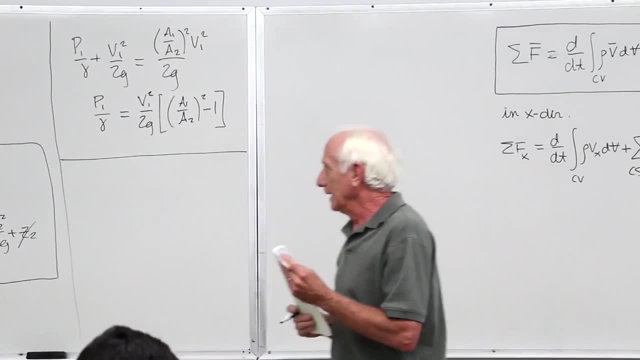 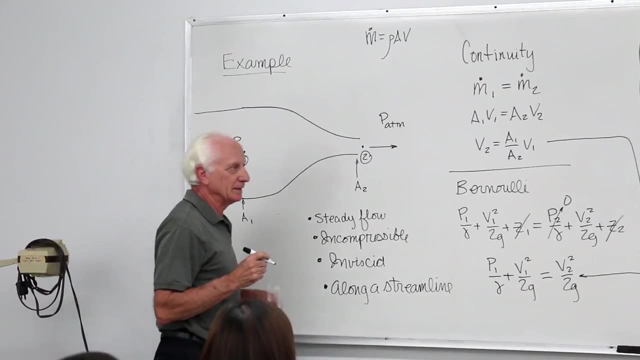 Now we tackle this guy over here, Maybe I'm going to say: you know what? I want to know what force it takes to hold this, This thing, in place. So now I'm going to do momentum. There's no Y, there's no Z. I'm going to do X momentum. 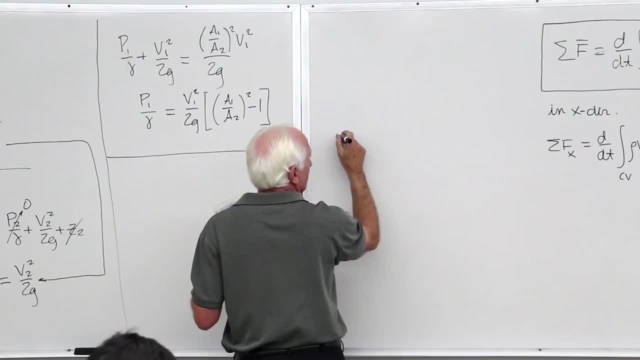 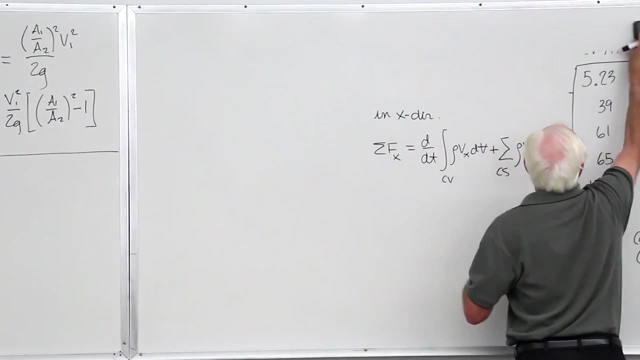 I better put this long, so I'll put it up here. I'll put it right here. Yeah, that's fine. It won't be him. Matter of fact. there, he is right there. Alright, I'm going to draw this picture now. 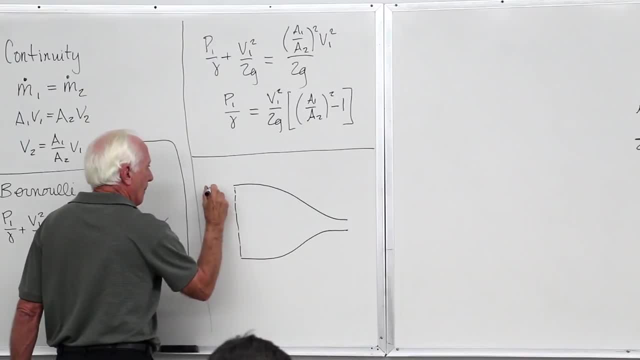 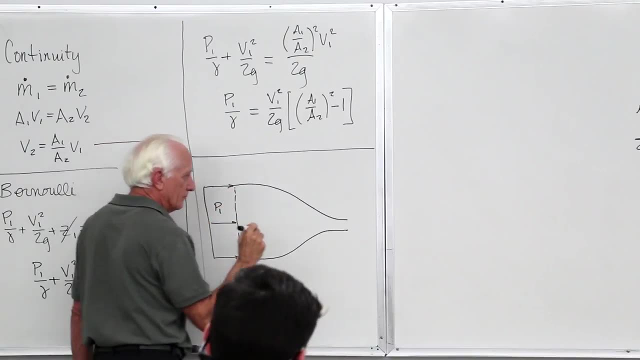 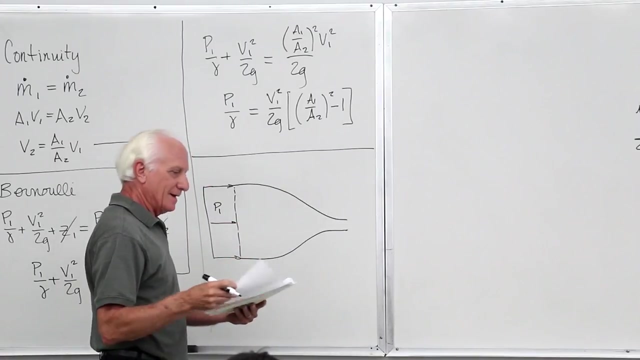 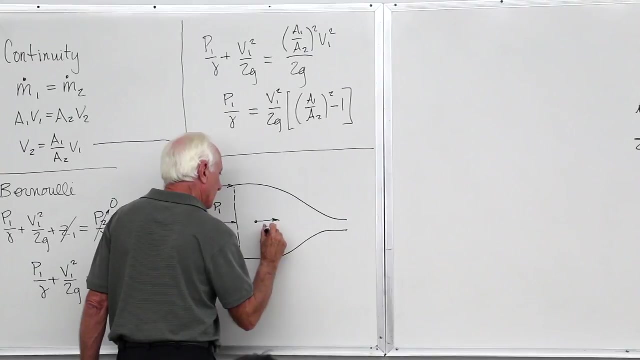 Okay, That's P1.. I'm going to assume that. assume direction on that, I probably do. I'll just assume that the force is in the plus X direction, since I don't know any different. Now let's put the. make it easy for us. 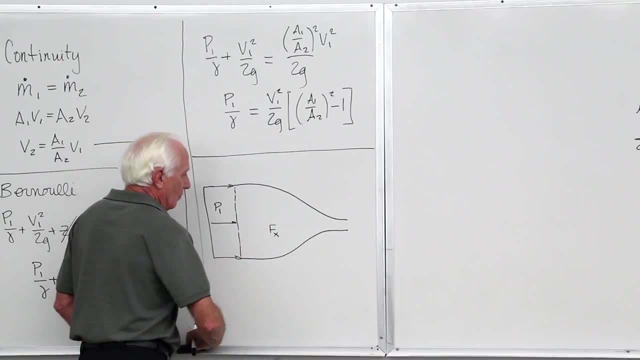 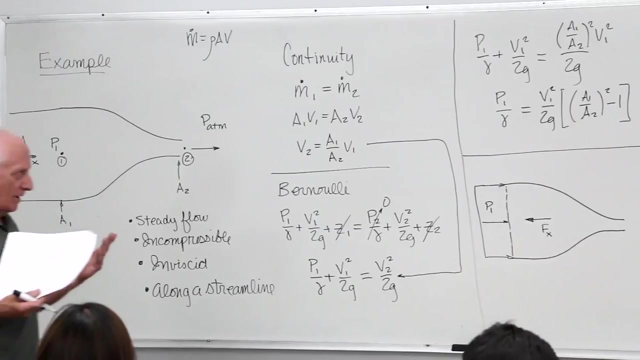 Um, What force? Let's say: what's the force required to hold this thing in place? What's the force required to hold this thing in place? I'm going to assume it's pulling backwards. If I'm wrong, guess what statics? I'll get a minus sign If I'm right. 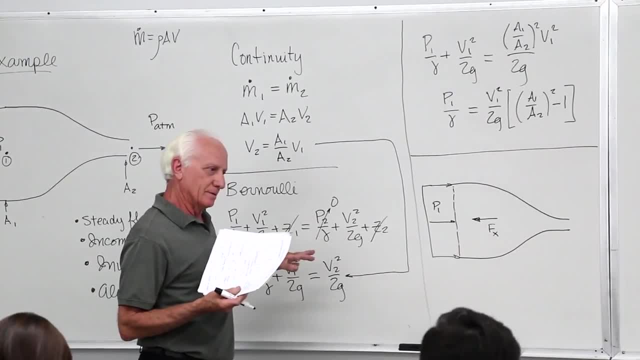 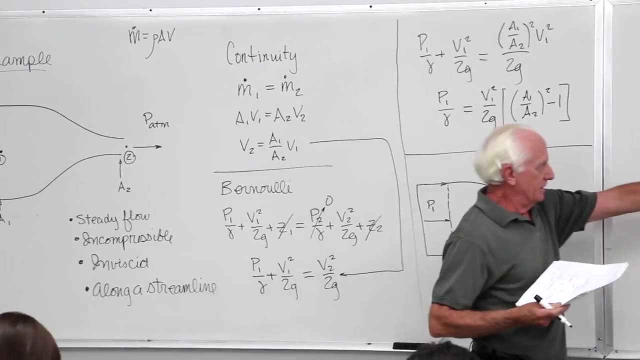 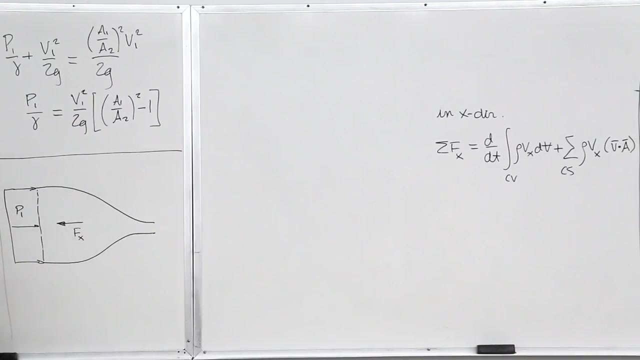 fx will be positive. So if you don't know, you guess It'll come out in the wash when you're done. Okay now, what's this diagram here? This is the left-hand side. All the forces that act on what? The control surface. Where's the control? 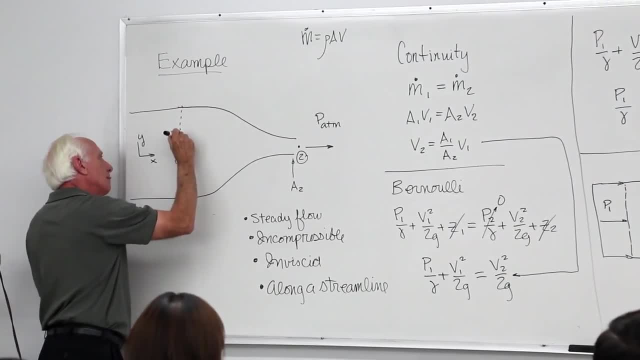 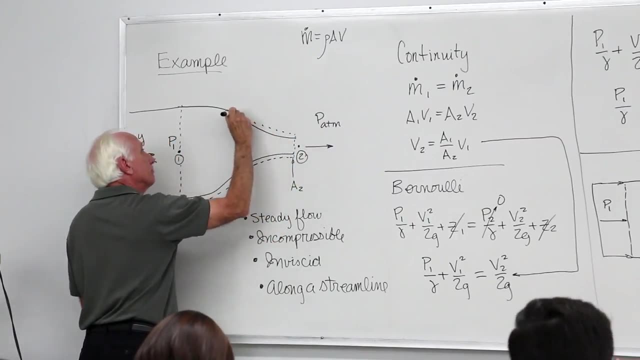 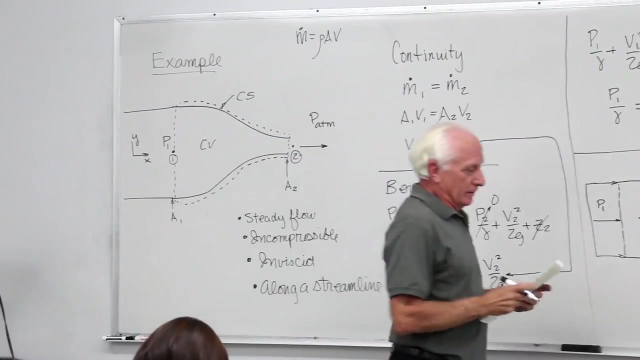 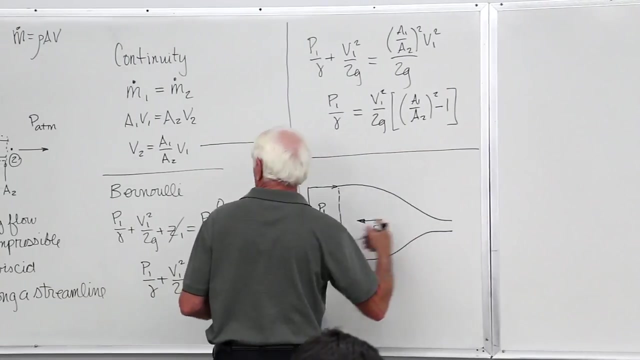 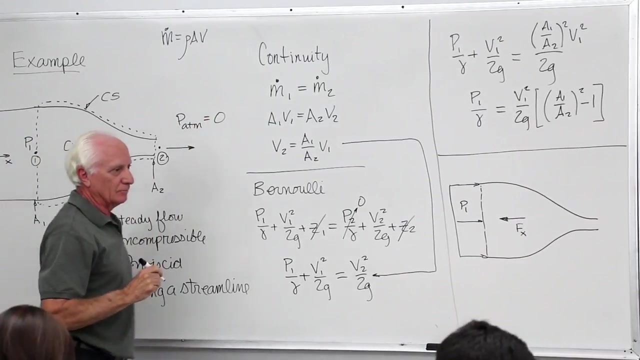 surface. Well, here's the control volume: Control surface, control volume. Okay, there it is. Where else to transport it there? Momentum, How about at this point here? Well, you know what p-atmosphere is: It's zero. 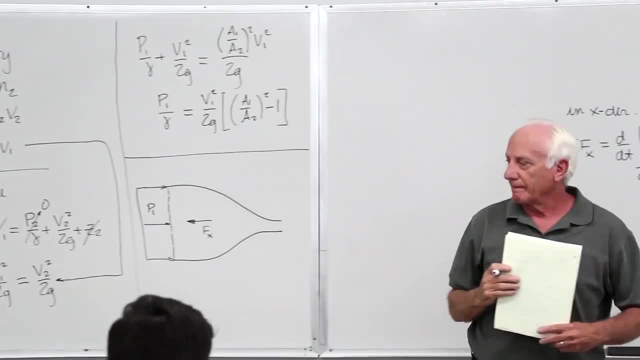 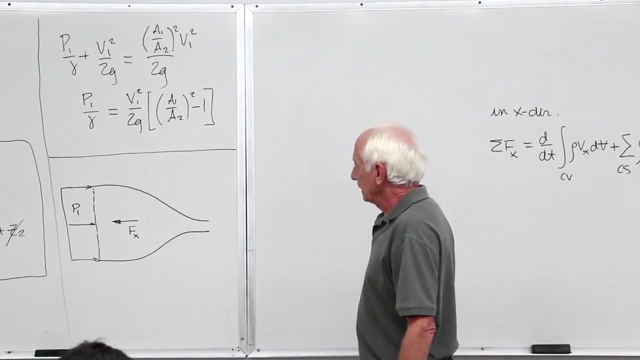 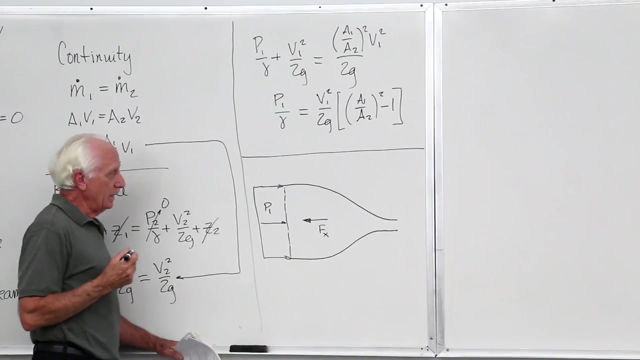 When somebody says p-atmosphere, that means zero gauge, So you don't show any pressure here. There it is. By the way, that's not a force theory. You have to multiply that pressure by an area, So the force would be p1, a1.. Which direction? 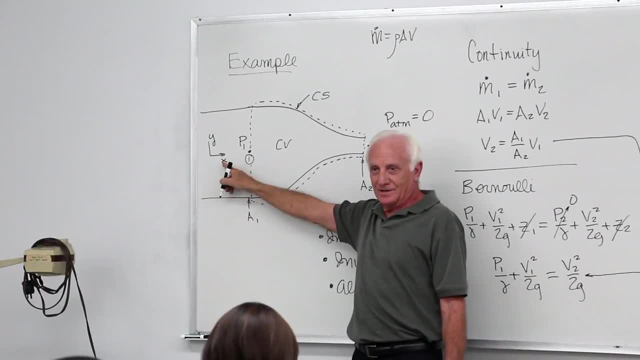 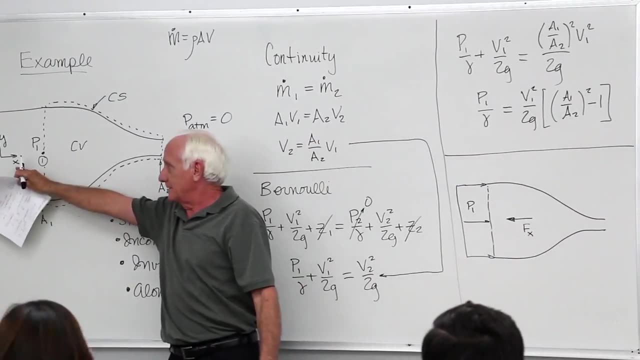 Always, always, draw your arrow directions when you start this guy, or you're going to get really messed up. You can't use any equation there without doing this. It's just like statics or dynamics. You're going to get messed up, So draw your. 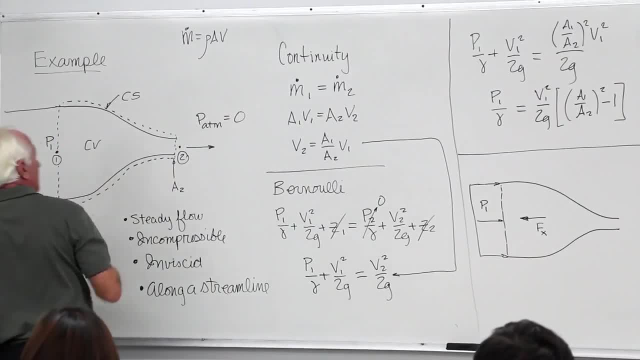 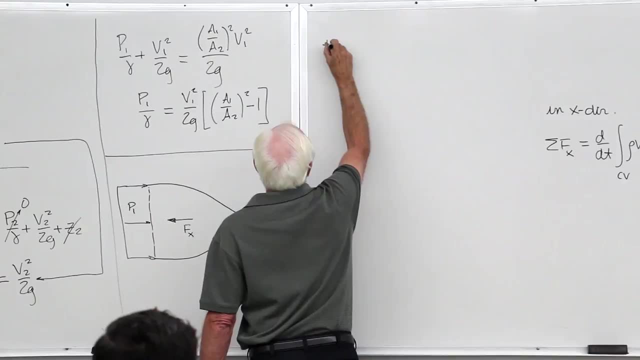 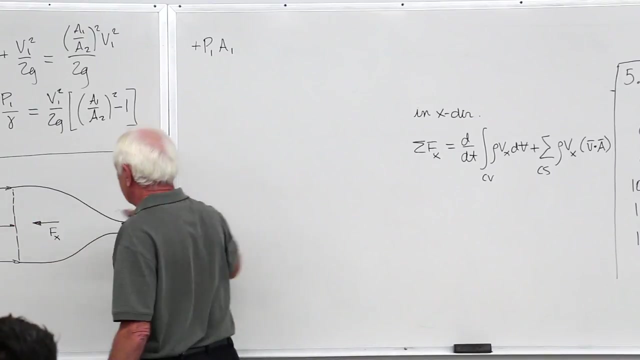 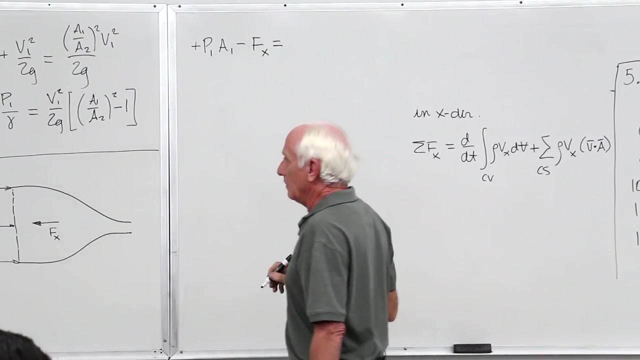 directions: Okay, p1, a1.. Okay, first term, which way To the right? Plus p1, a1.. Okay, I'm assuming we have to hold this in place. I'm assuming we have to hold this in place. So we're pulling back that way. Minus fx Equal. Okay, Now we do what. 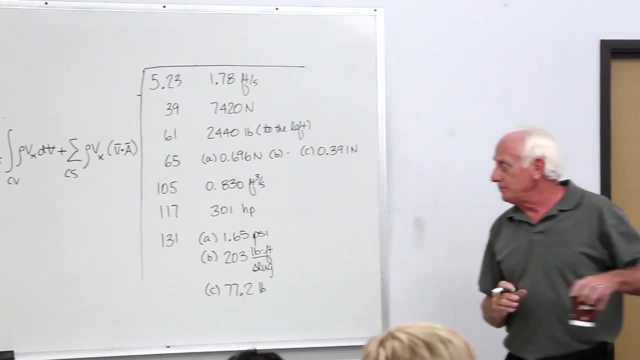 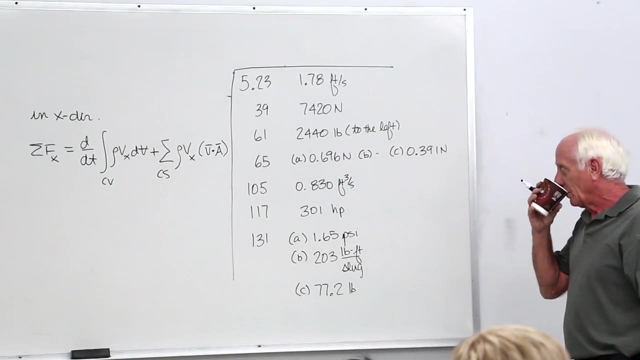 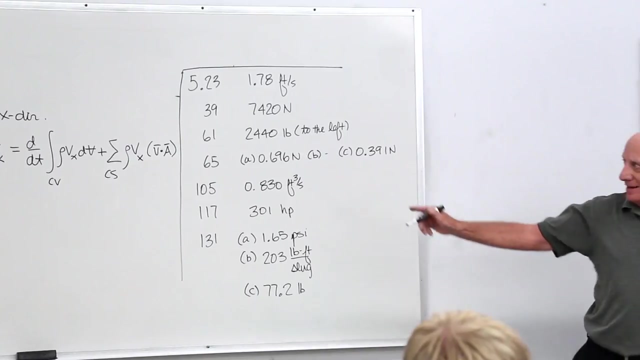 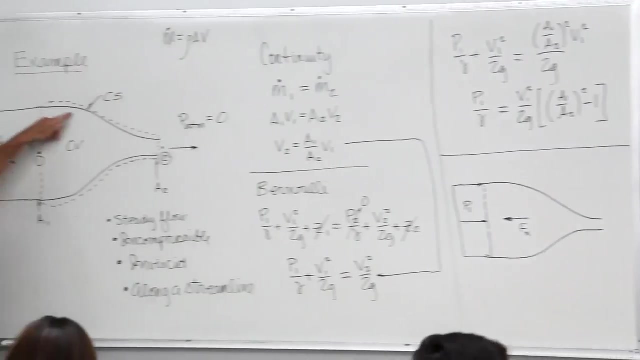 it says there. What it says there is: go around the control surface. Go around the control surface Wherever fluid enters or leaves the control volume. there's going to be a contribution from this term, So go around the control surface until you reach a point where flow crosses. I'll start lower left. 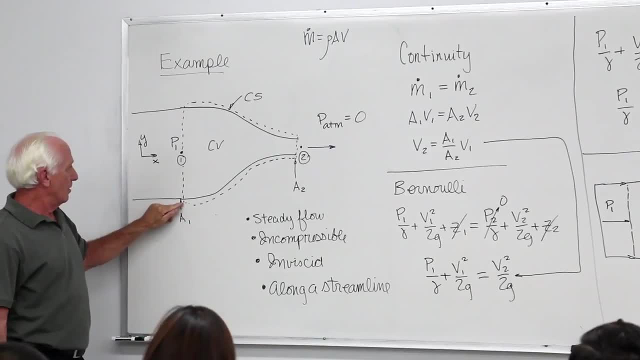 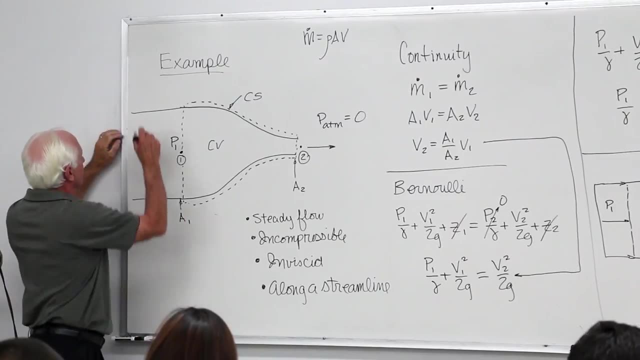 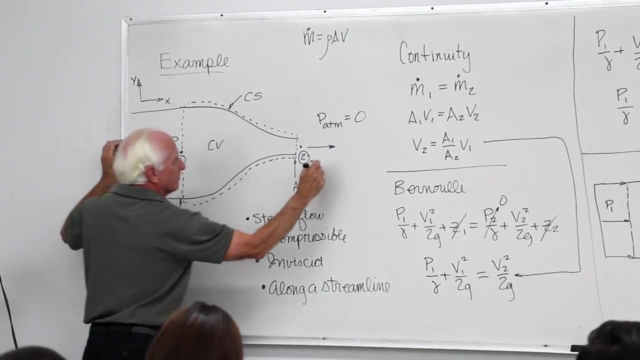 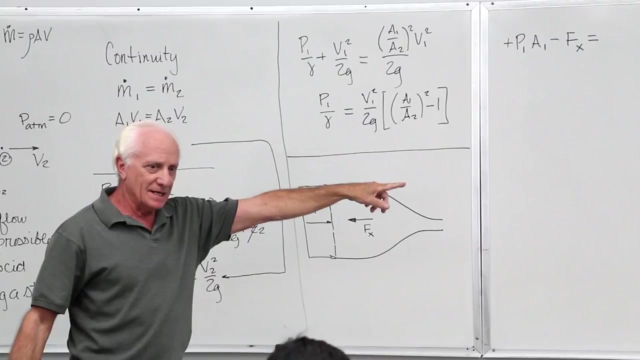 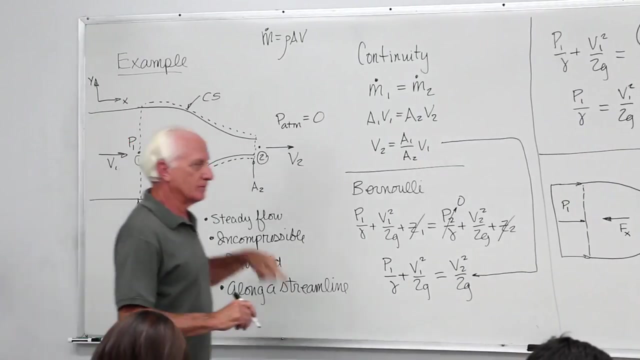 hand point. right there I go upward. Oh yeah, there's a velocity here V1.. Yeah, v1.. Do it as saying Okay says take the density there times the velocity in the x-direction, Rho, times plus V 1. V 1 is in the plus x-direction. 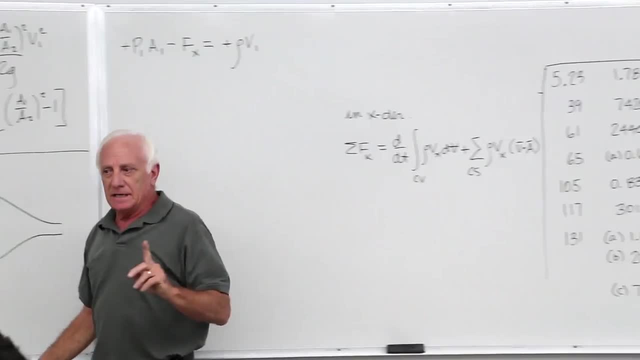 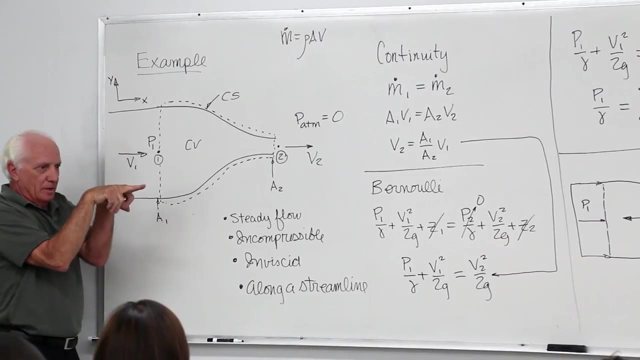 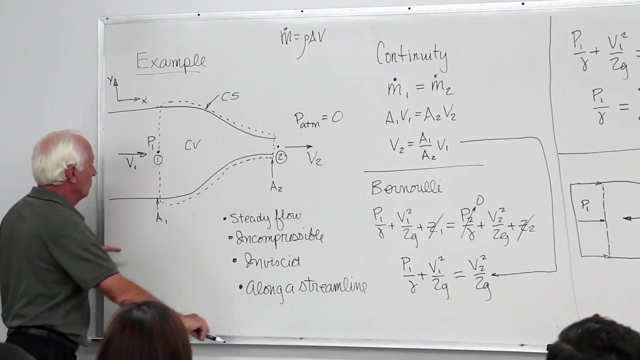 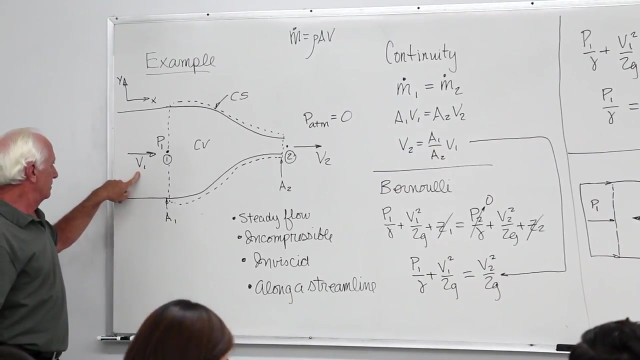 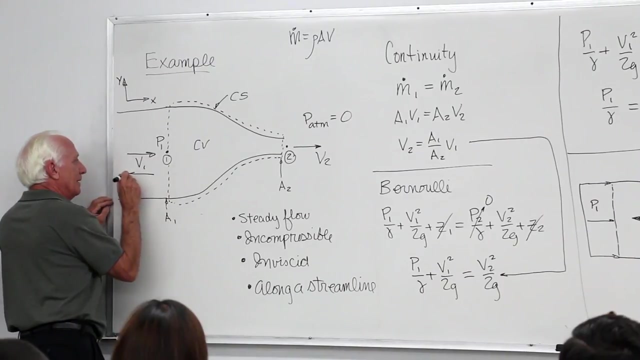 okay, now find V dot a there. Oh, the vectors are collinear. the angle between them is cosine of 0, 1. okay, so it's one. the sine is 1 and magnitude of the velocity V: 1. magnitude of the area a: 1. so it's gonna be area vector velocity. 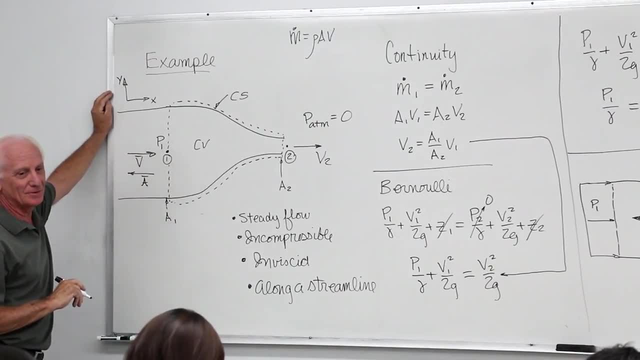 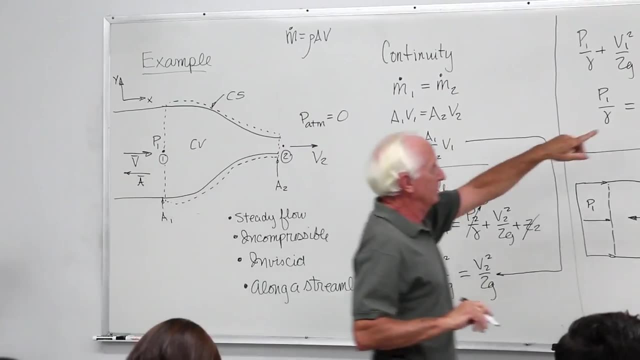 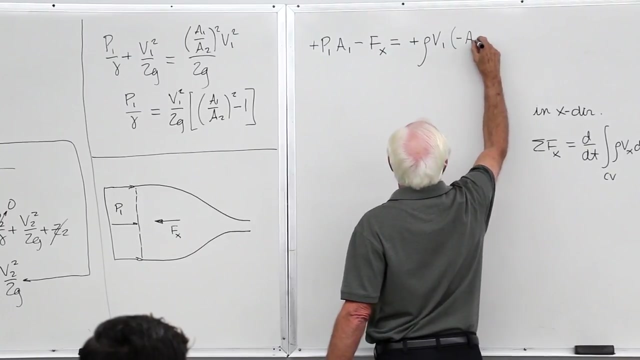 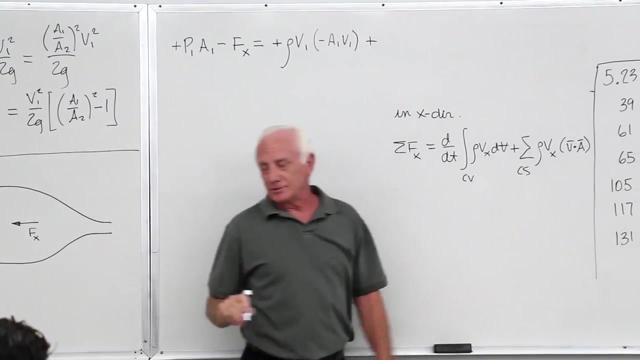 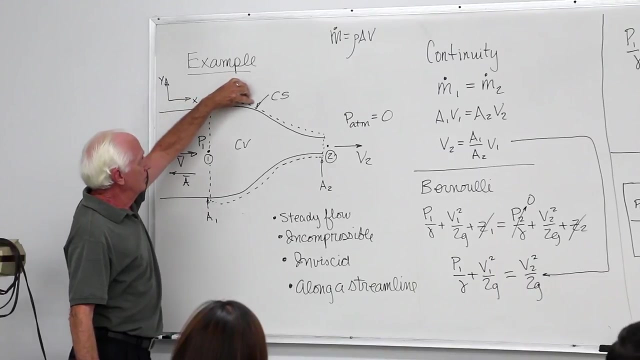 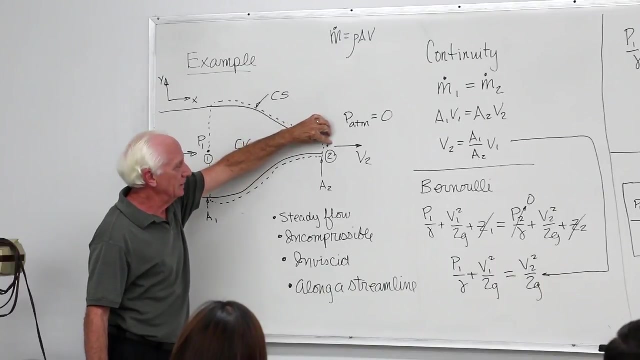 vector cosine of 180 minus 1- okay, minus 1, okay, and a 1 V 1, all right. keep going around the control surface until you find a place where fluid enters or leaves. no, no, no food entering, no food leaving, no, no, stop, yeah, yeah, yeah, leaving, leaving, okay. Rho times the. 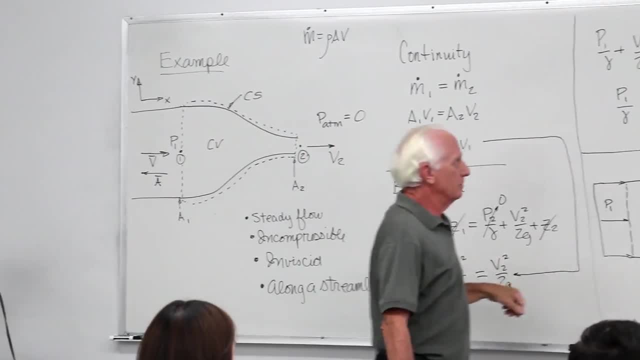 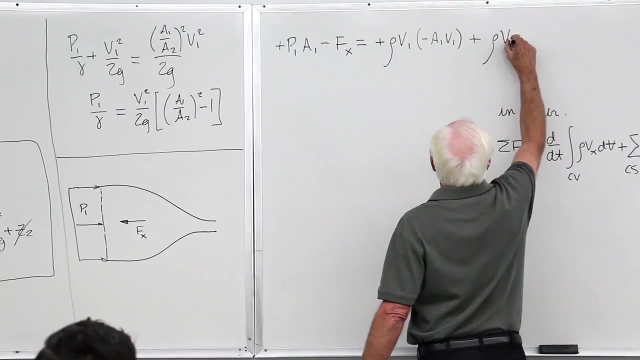 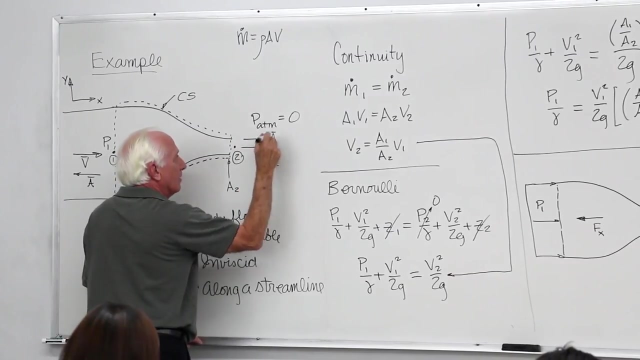 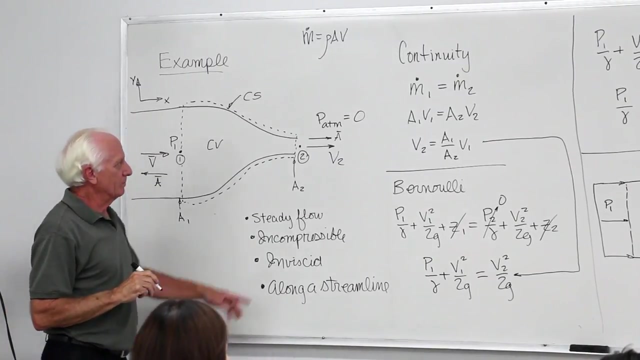 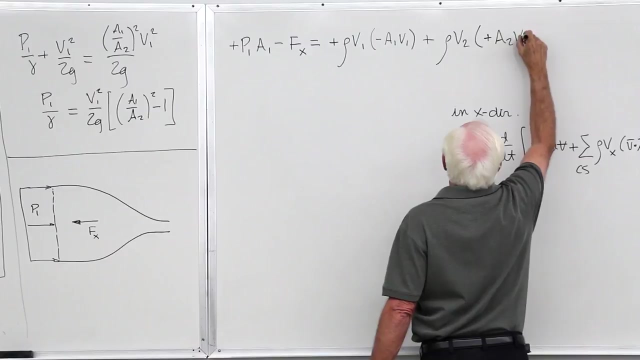 velocity in the x-direction there Rho, which way? velocity going positive, positive Rho V 2 times V dot. a area vector always points outward from the control surface. cosine 0 plus 1 plus 1, no more fluid crosses the surface on the bottom, on the. 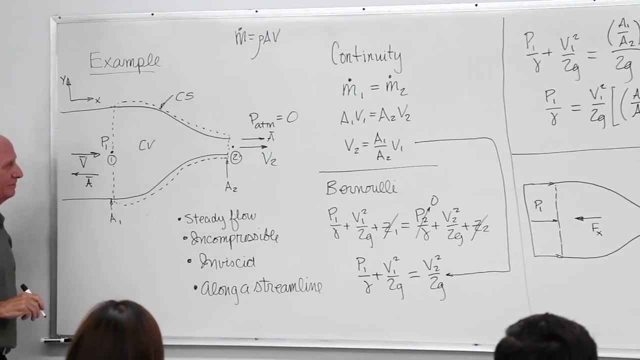 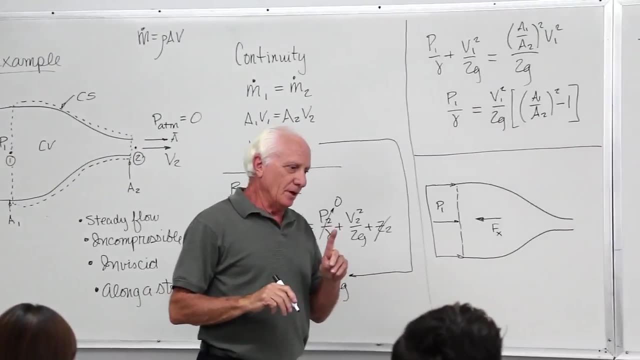 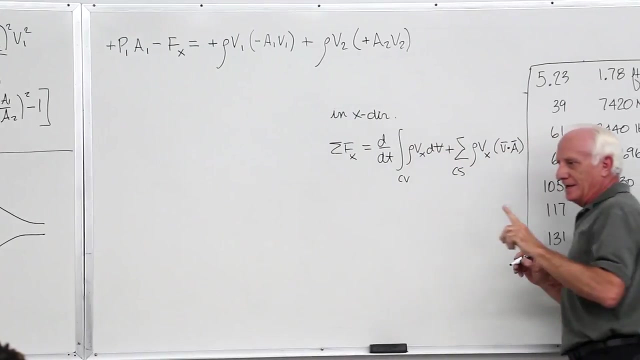 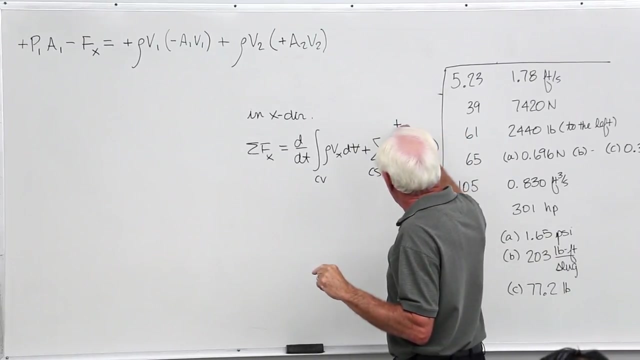 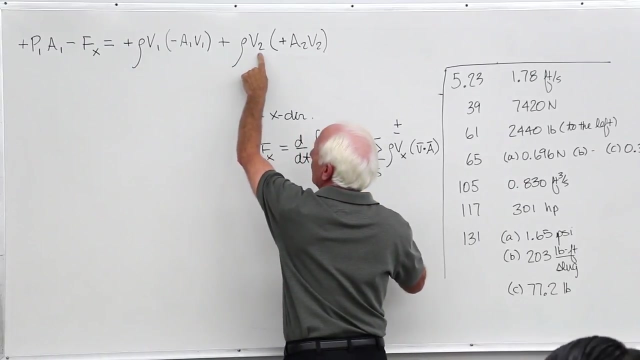 bottom. no, no, no, no. okay, now, just so you know there are two. and then just to tell you about two signs, two signs in this summation here, two signs, and you better do your book keeping correctly. the velocity in the x-direction can be positive or negative. application one: it was positive, D 1 at location. two: it was positive, V 2. 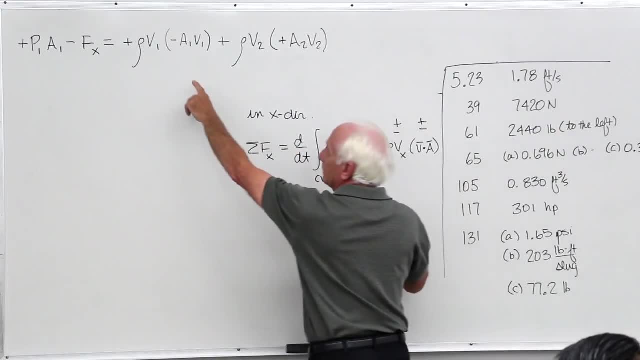 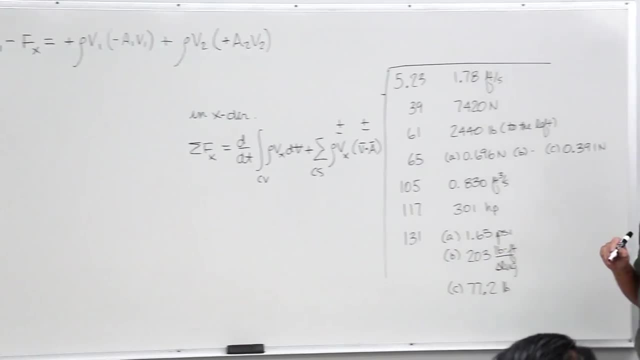 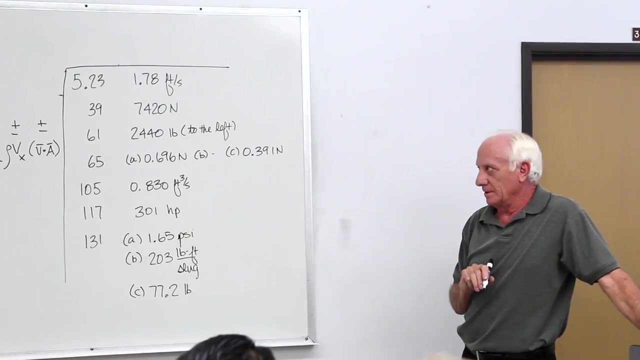 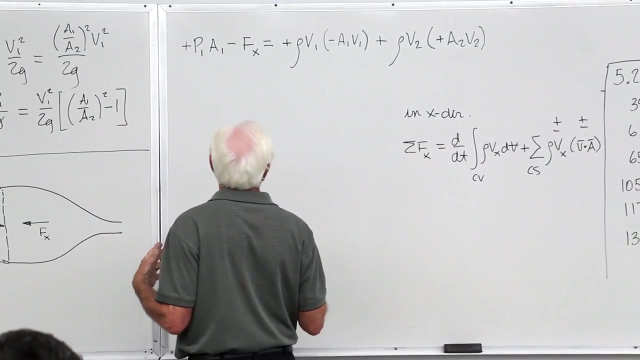 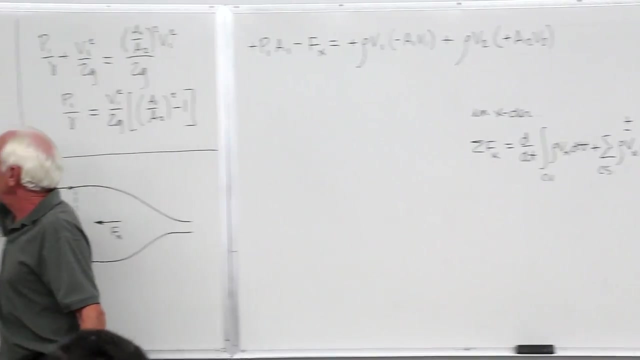 comes a second sign, V, dot a. it can be positive or negative. it was positive at negative at the end. so, yeah, you always want to check two signs when you tackle that turn. that's where you do your bookkeeping incorrectly and you get the wrong answer. okay, now, if you want to simplify, yeah, go go ahead. a 1 B. 1 a 1 B. 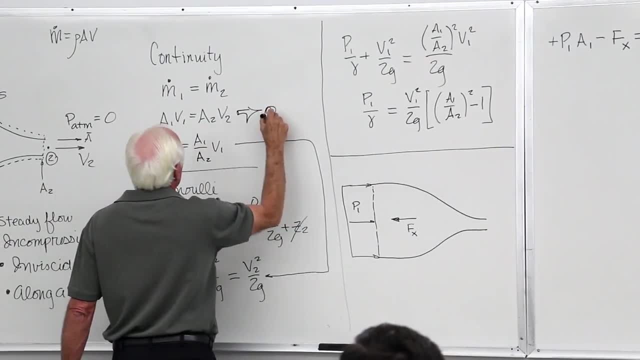 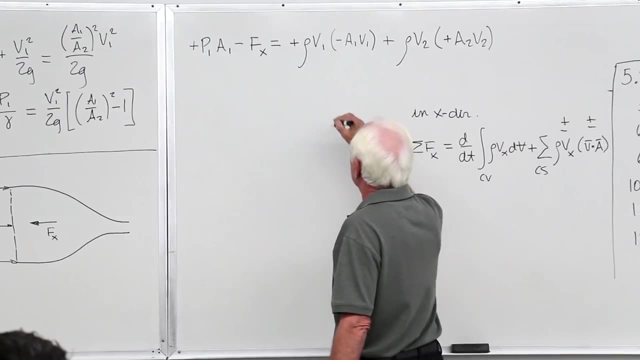 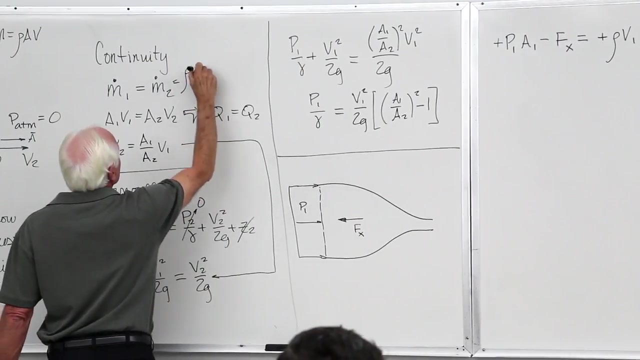 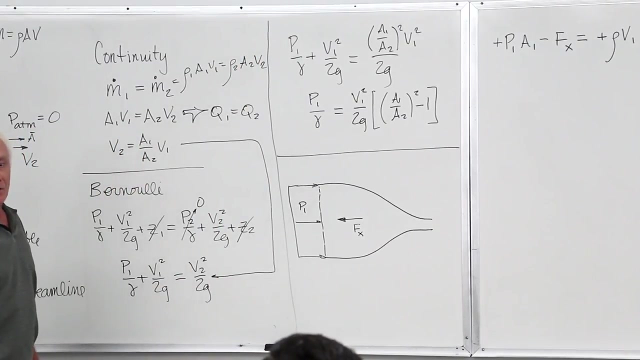 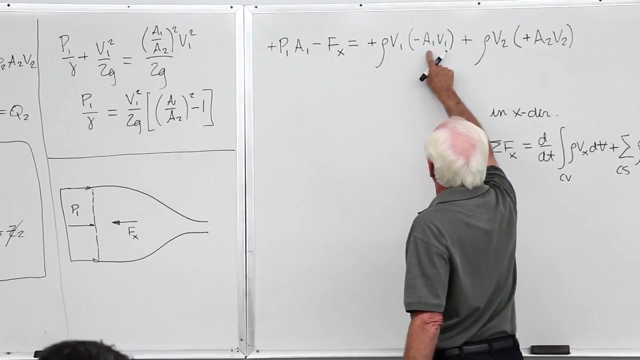 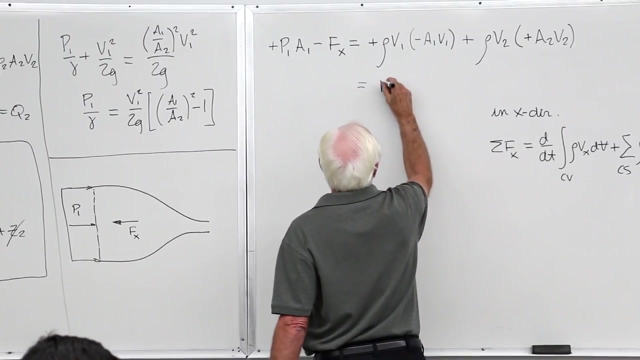 1 is Q 1 equal Q 2. how come conservation of mass Rho times a 1, B 1 equal Rho 2. a 2, B 2. how come? conservation of mass Rho distance is ended up. okay, this ends up. so we have M dot and this guy now. 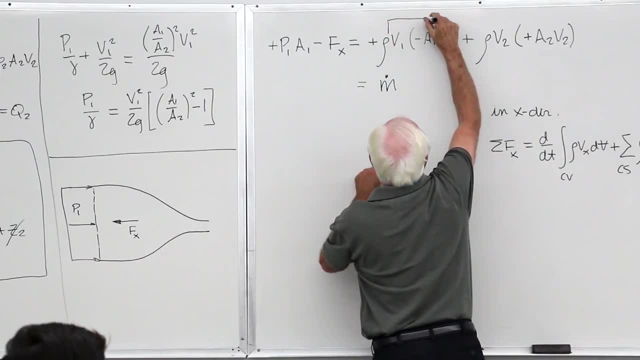 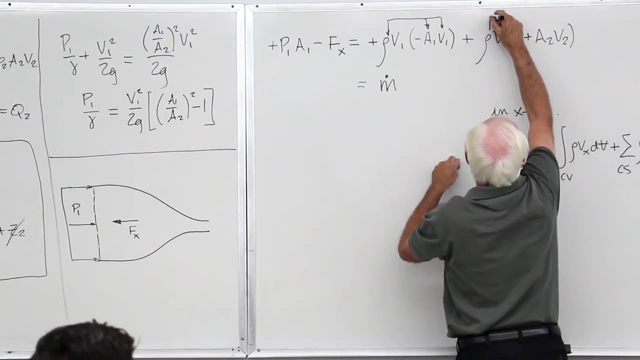 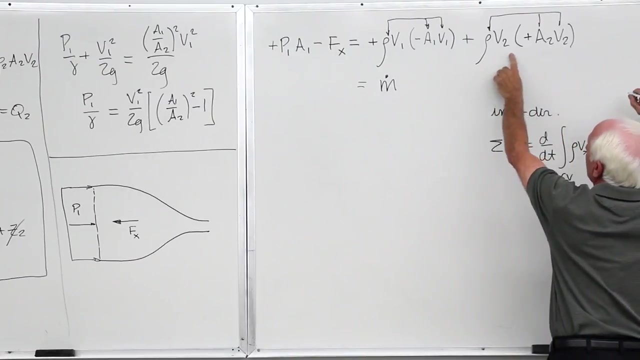 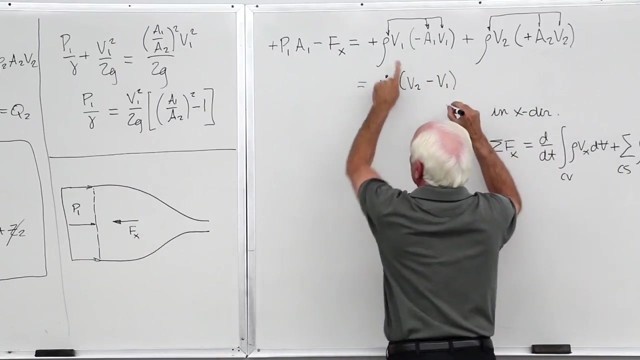 these three terms are M dot. if you want to just include them, I'll just take in this one. that's M dot. okay, and then what's the positive one, V 2, and what's the negative sign of V 1? and what's that? equal to P 1 a 1. 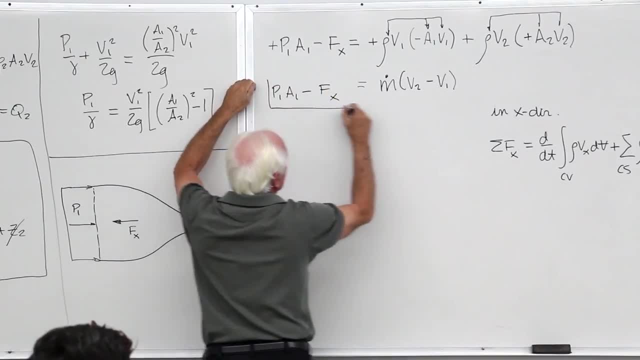 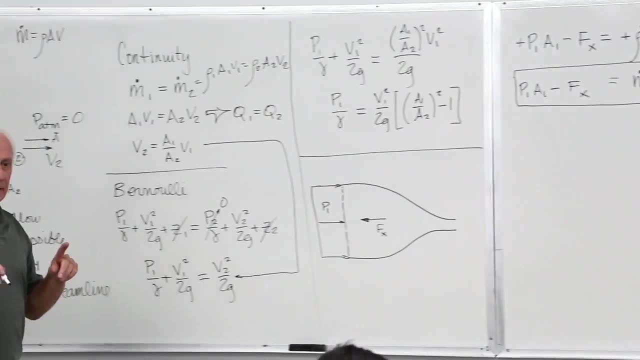 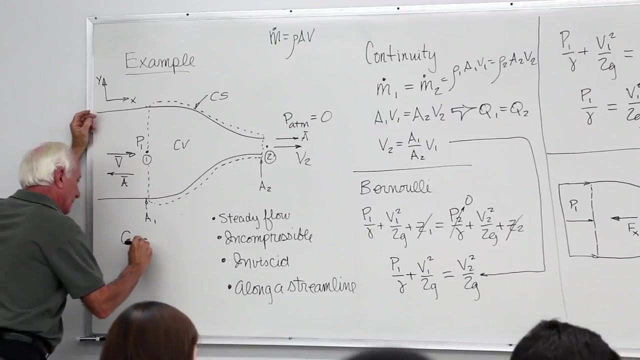 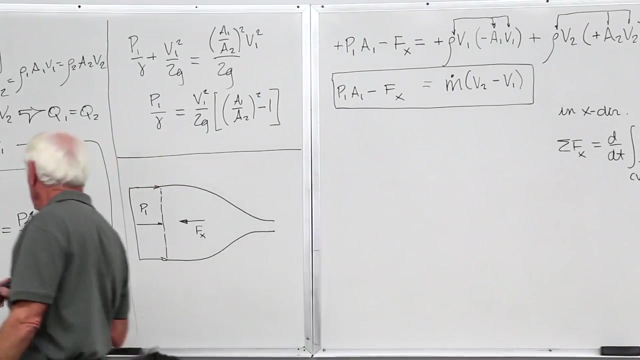 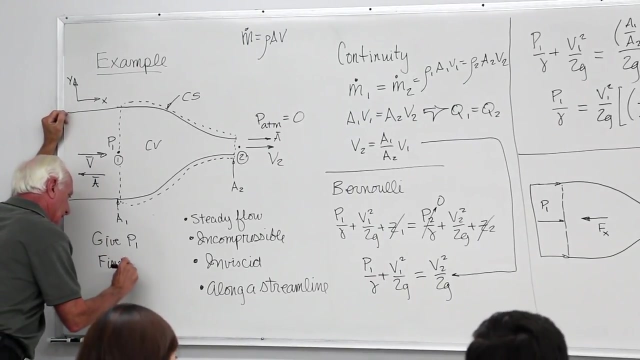 minus F X. okay, now Stirrie, any different? we're talking about the negative one with the M dot. however, the negative one goes in the negative of the. they can only, if it go in between here and then you have, wave these numbers over here and then you go. 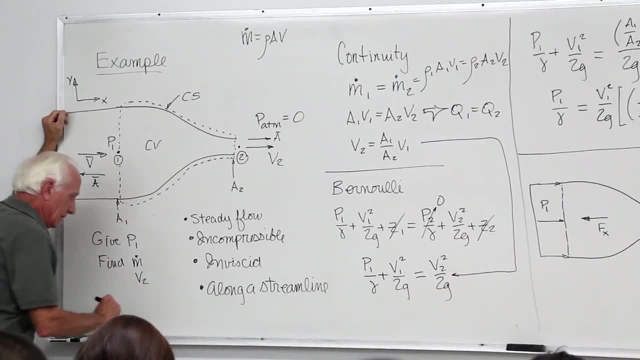 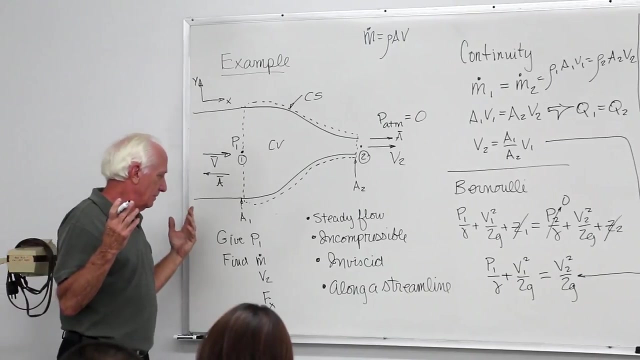 That's where we are dead. now you join this vibe, oh well, the other labels you see in here. it's got a V M dot value to V 1 is equal to 4, D1, P1 given, and then I need to for a in place. I just picked those three. I can say: find flow rate, Q2, find V1, find. 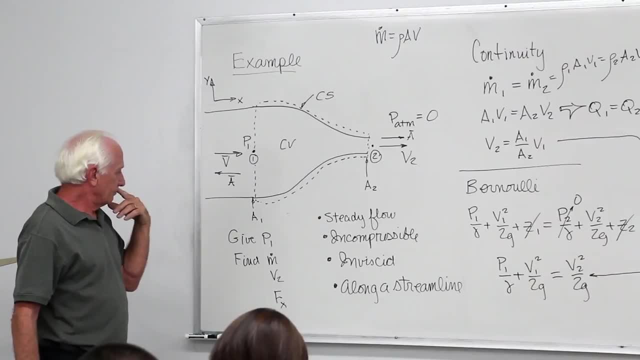 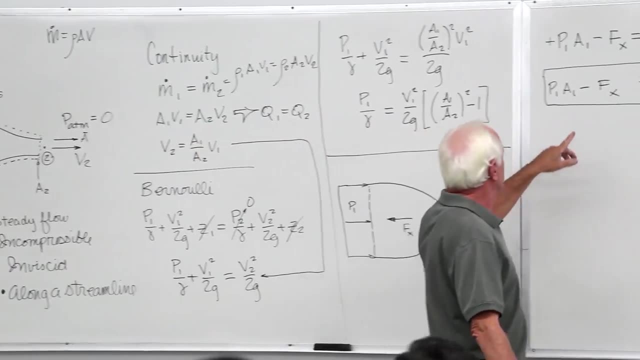 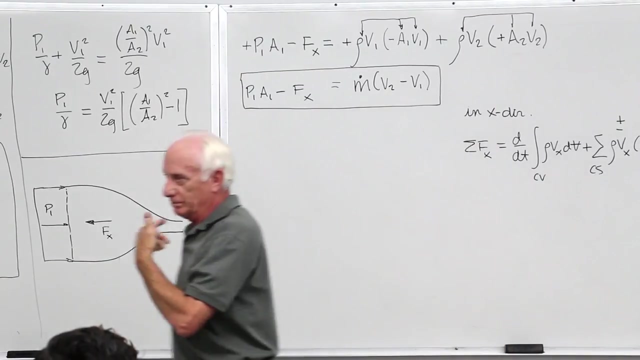 FX. Okay, Let's try and find FX. Try and find FX. Okay, FX. Do I know M dot? Not yet. Do I know P1? Not yet. V1, V2, that's a bad place to start. Given P1,, given P1,. 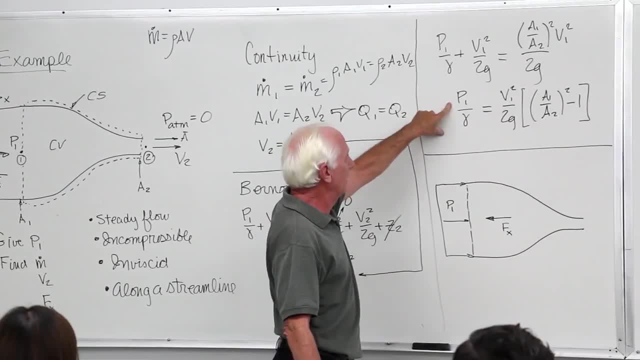 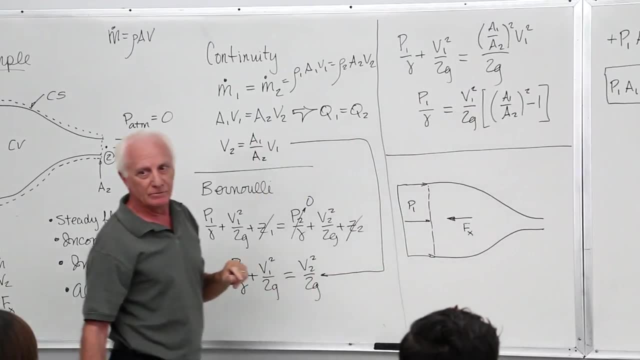 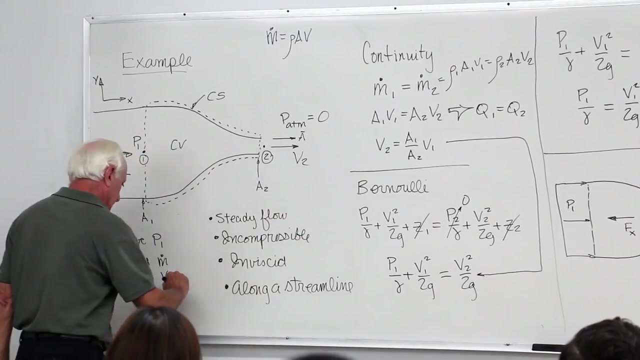 let's see P1, P1, P1.. Ah, there's P1.. I know A1, A2.. That's given, Guess what I find. You got it V1.. Once I know V1,, can I find V2?? Yeah, you got it. Got it Once. 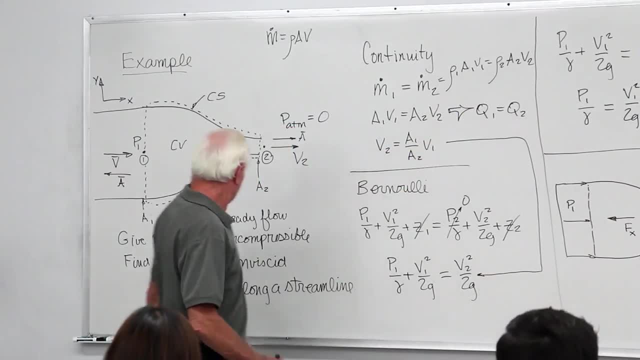 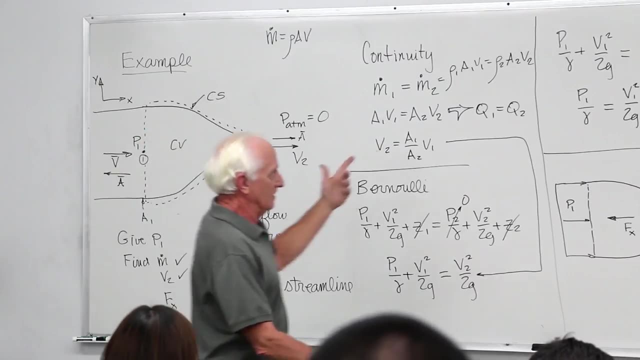 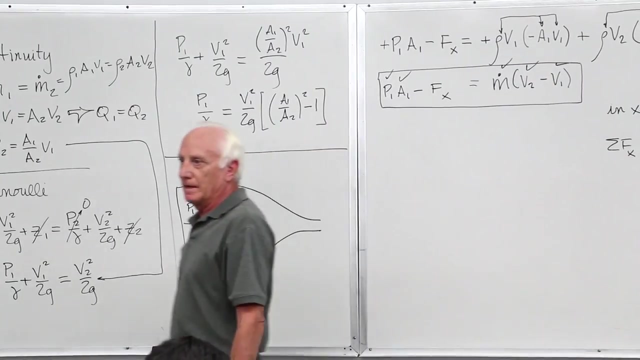 I know V2, can I find M dot? Okay, Of course I can. So I'm given P1, I'm given P1,, sorry, Given P1, given A1, found M dot, found the velocities. There you go. Solved for FX. If you get confused, write all those. 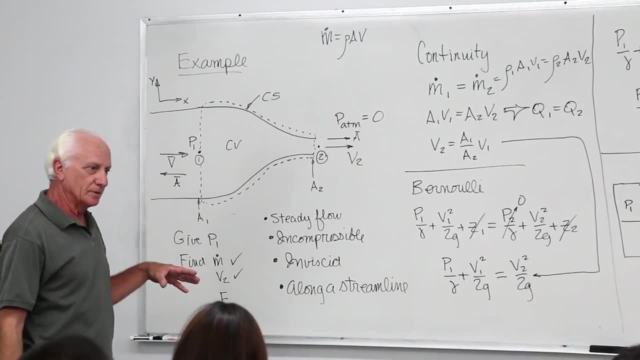 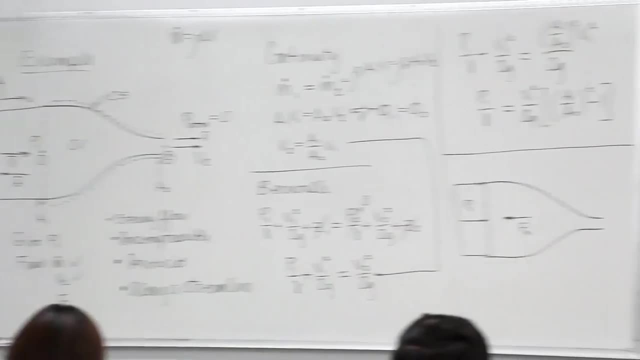 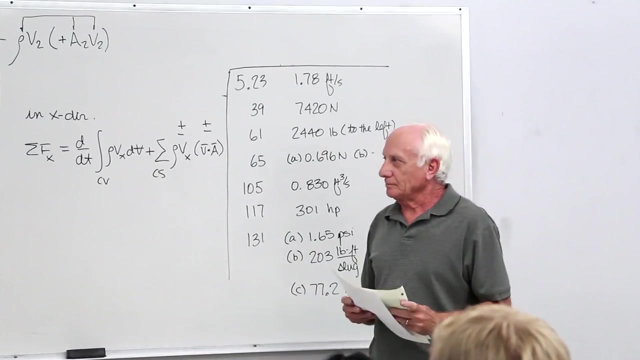 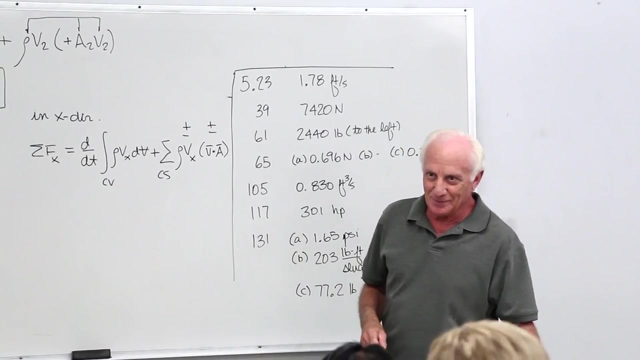 equations down and stare at them a while. Maybe something will pop out at you. Hopefully it will, But they're all linked together. Okay, now Let's take a look at some homework. Yeah, go ahead. Can you explain why the a vectors go to the last one? 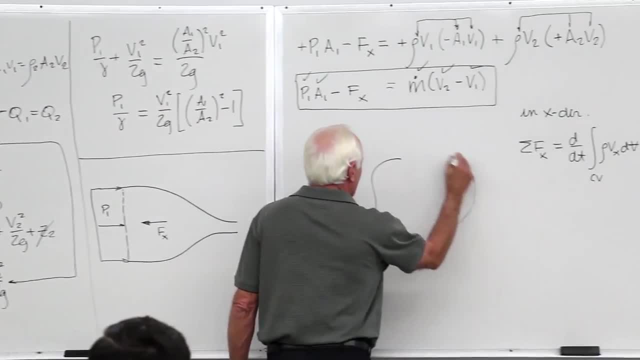 Yeah, yeah, I'll do it over here. Here's a control volume. Here's a control surface. No matter where you are on this control volume, if you're on the right side, you're going to be used for that, Yeah. 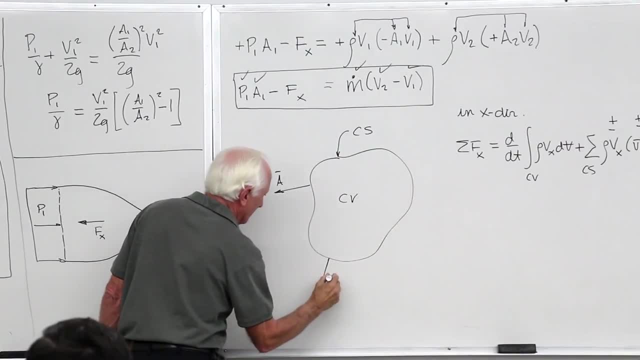 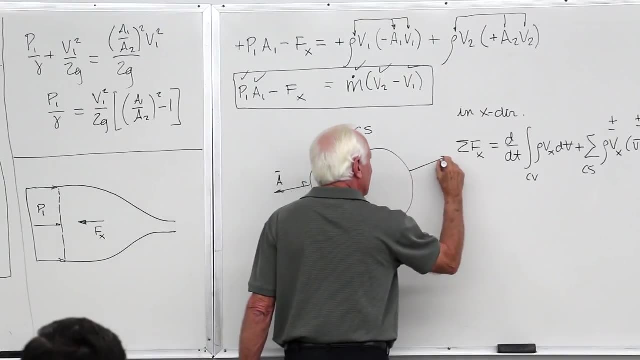 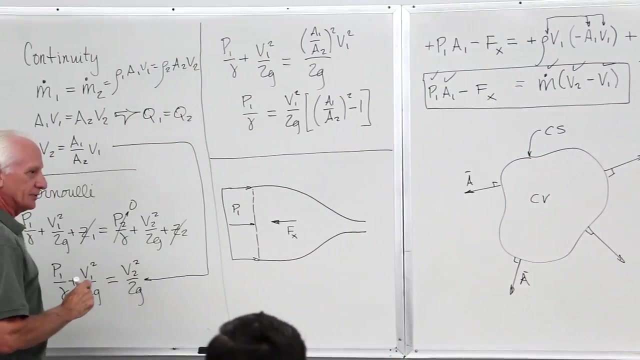 This is a 1.. This is a 2.. This is a 3. the A vector always points out: normal by definition. by definition. That's the way the area vector always points out. It's just like this. you know it doesn't. 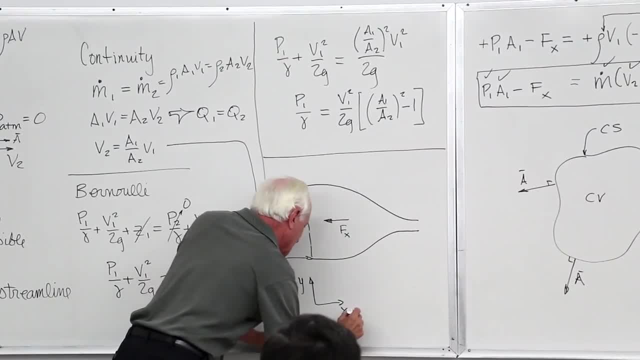 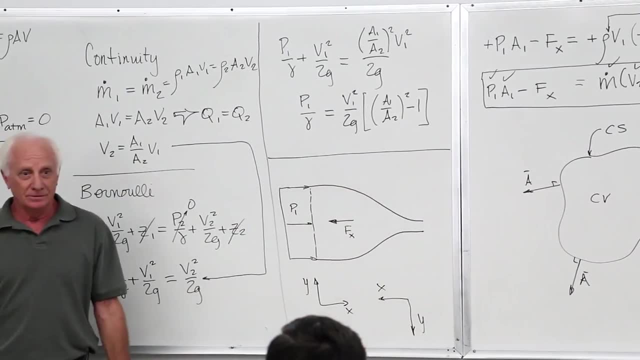 matter. It can point in or point out, but make up your choice. You know, some guy says I like that. This guy says: oh, I hate that. I'm always off the wall. I always call that positive. You do That's okay, I guess, but I don't, And most of. 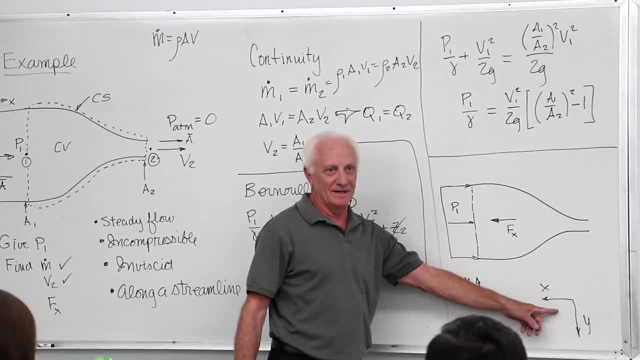 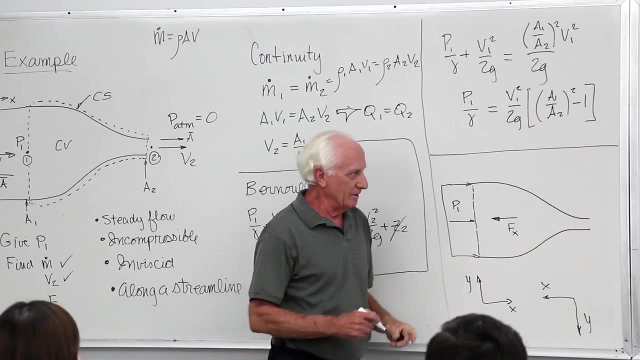 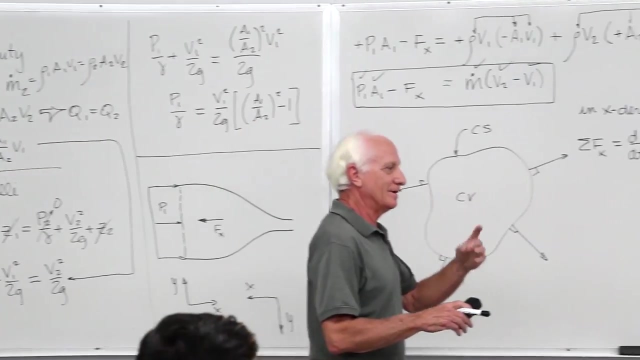 the world doesn't. But is this guy wrong? Of course he's not, But most people do it this way. That's just the way we do it. That's the convention. Convention Area vector points outward: normal from the control surface. Homework over here, Yeah. 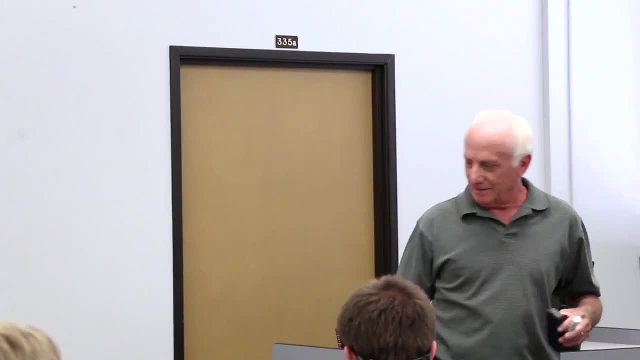 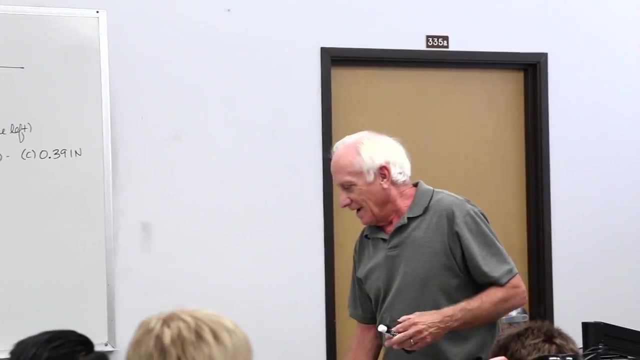 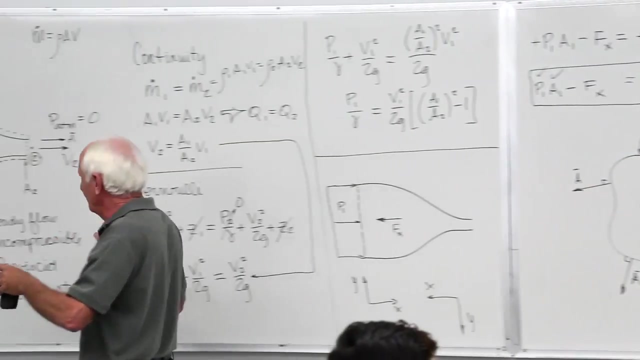 we got it all the way around here, right? Oh, this is Okay. Just this one. Okay, If you didn't get it, let's see Christian. Okay, All right, Let's go over some. we'll come back to this and we'll spend all next class time. 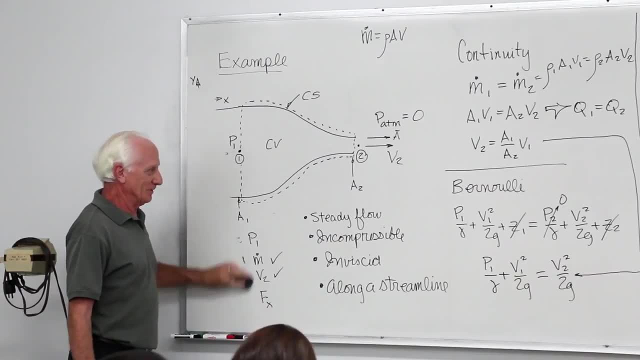 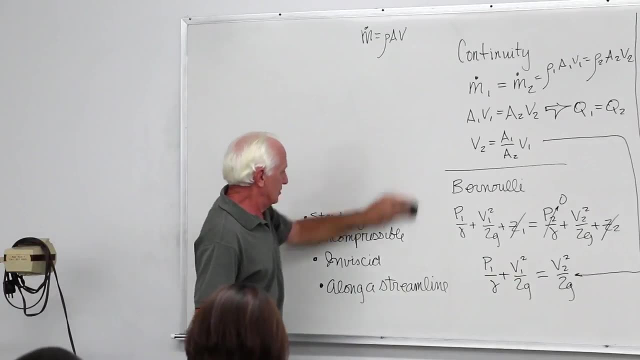 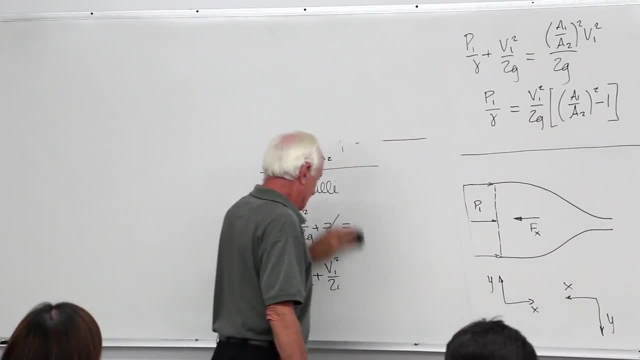 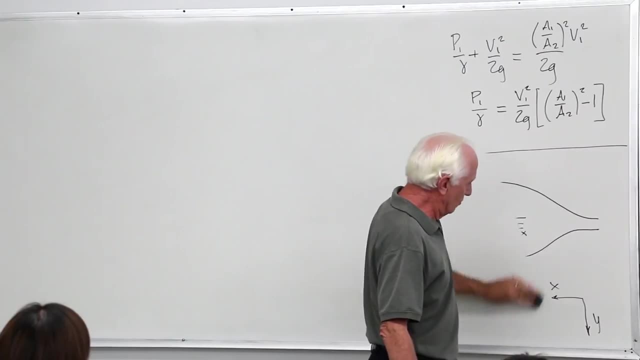 5.. We did momentum in Chapter 5. And most problems you get. this is especially true of things that you can find with a pen. you have to figure out which ones you need to get the answers you want, And that's why you want to have those in your library ready. 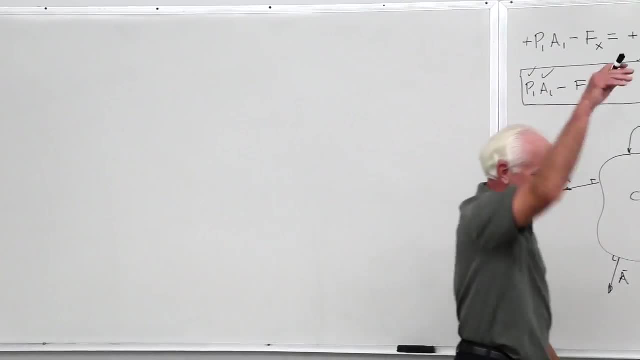 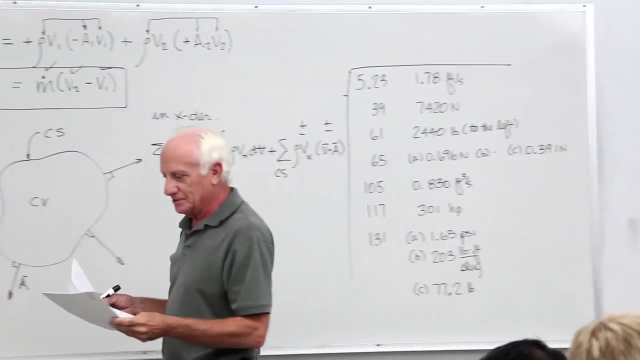 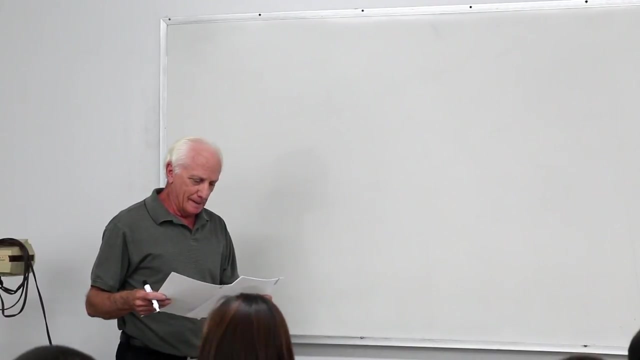 to use and to look at. Okay, Let's take a look at this. I'm pointing some things out here now about the homework I saw, Plus, we'll go over some problems. This is similar to a problem that you were assigned, which was problem 350.. Okay So, 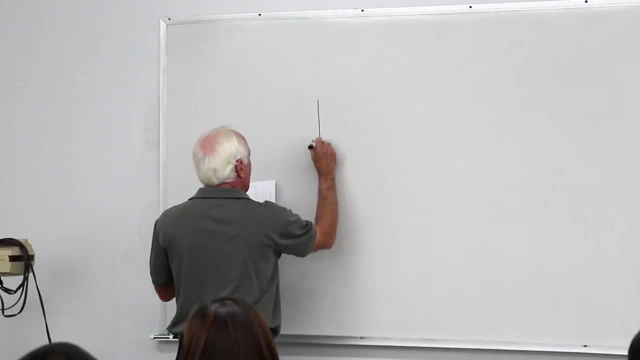 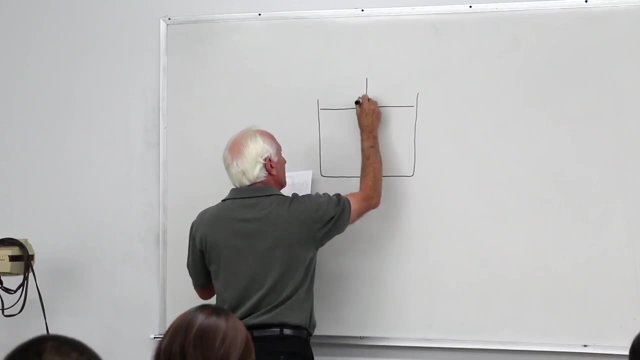 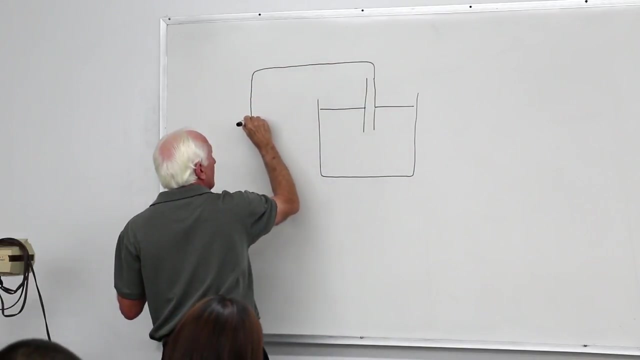 I'm going to draw a picture similar to that, but not the same thing. This is a siphon problem. Here's the siphon. It comes out of this reservoir, It goes up over here, goes down and like this: 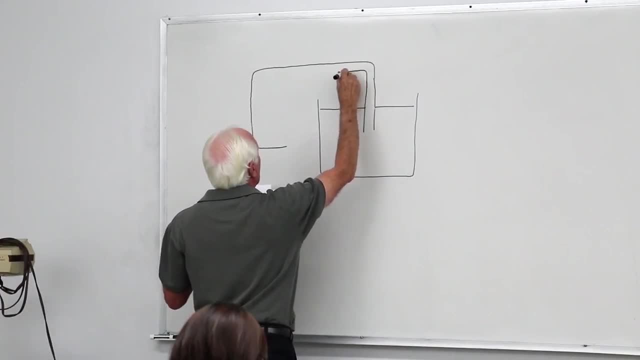 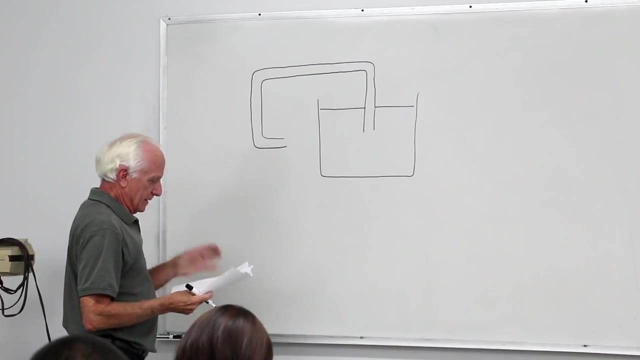 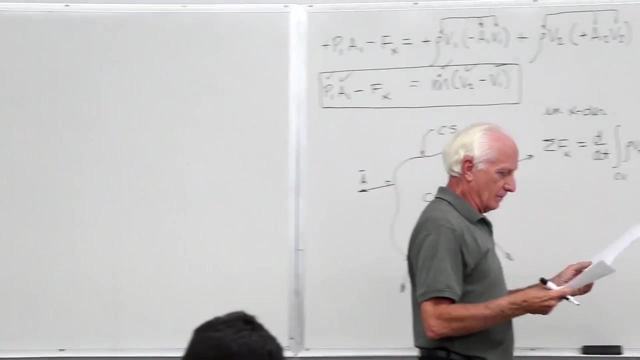 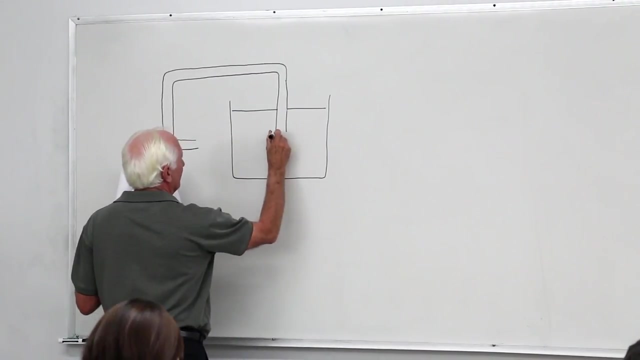 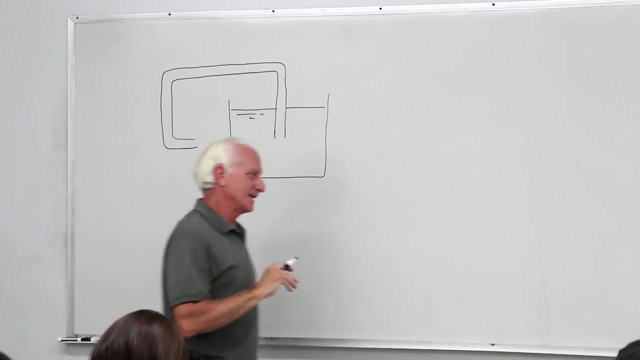 And let me just check it here and see if that's: oh no, I don't think that was in 350.. Oh, there, it is 359.. I don't, I'm not going to draw, Okay. So there is. I'm doing it my way. It's very similar to his way, but I'm not his way. 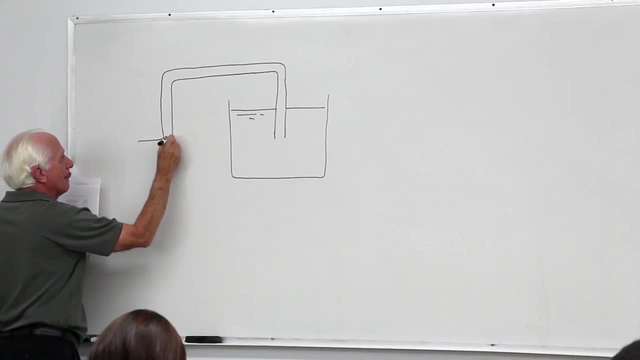 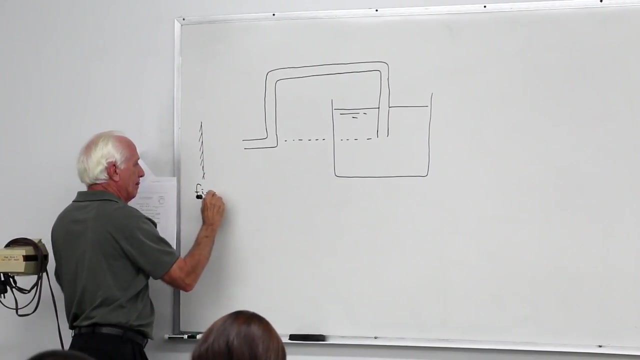 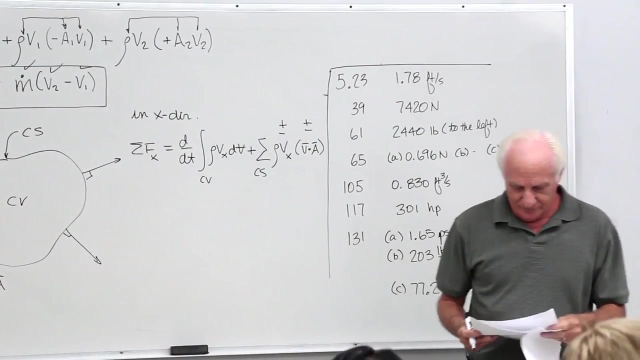 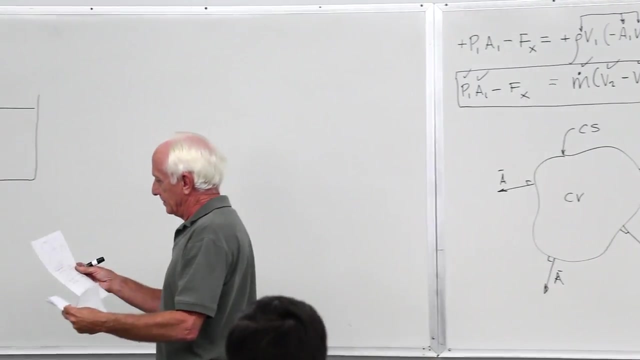 I think this is better. These guys are in the same line here. It doesn't matter, It's only a picture. Here's a fixed wall. The wall comes out. It's the wall. It's a siphon problem. I'm going to put some dimensions on here, just in symbolic terms. 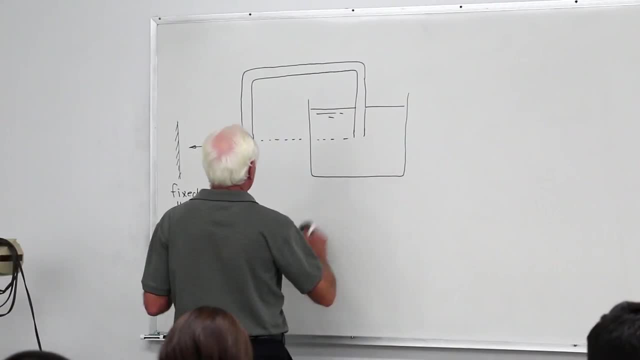 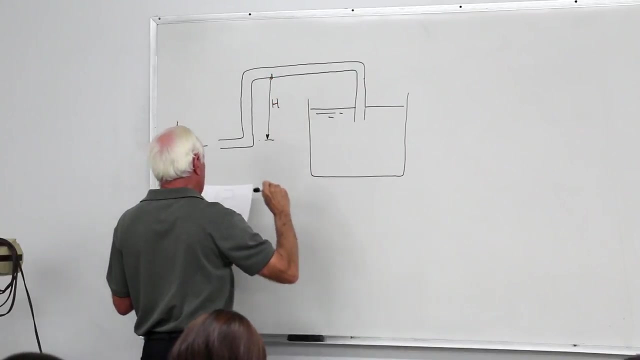 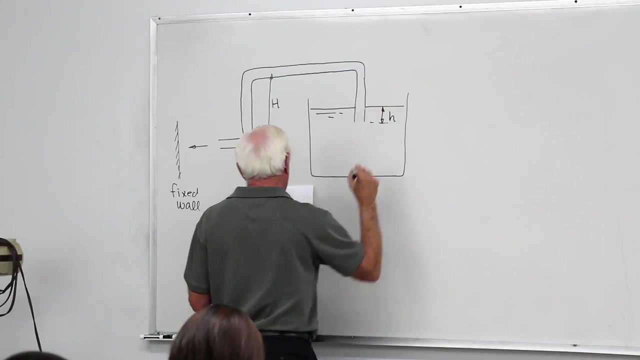 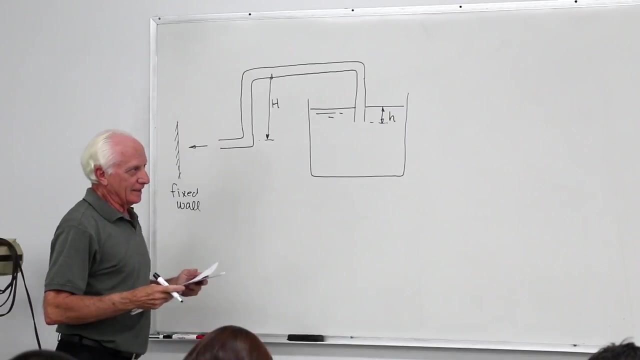 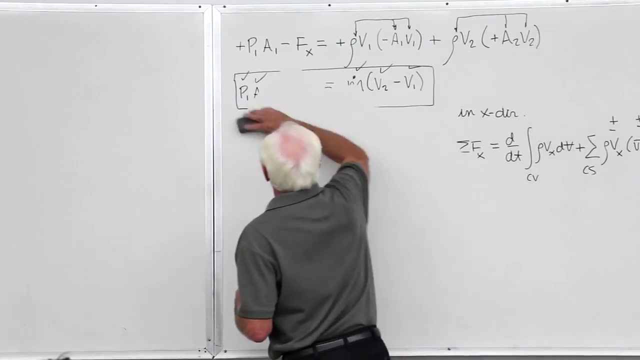 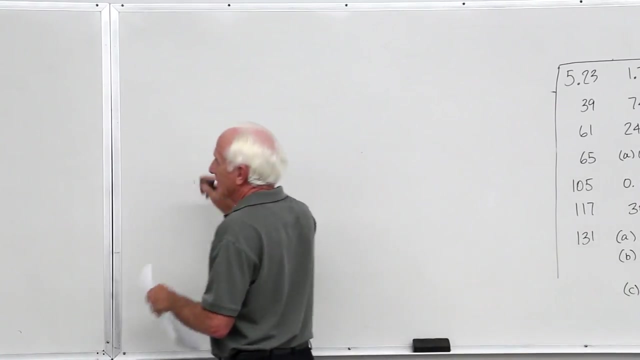 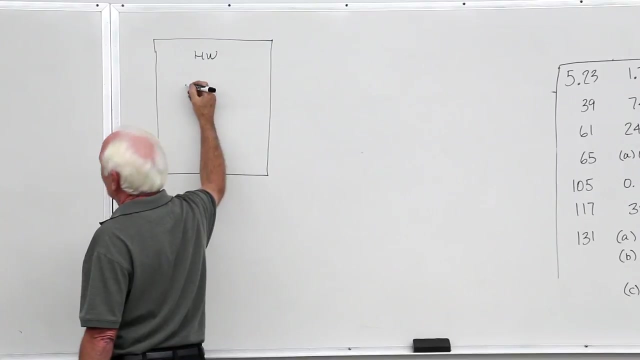 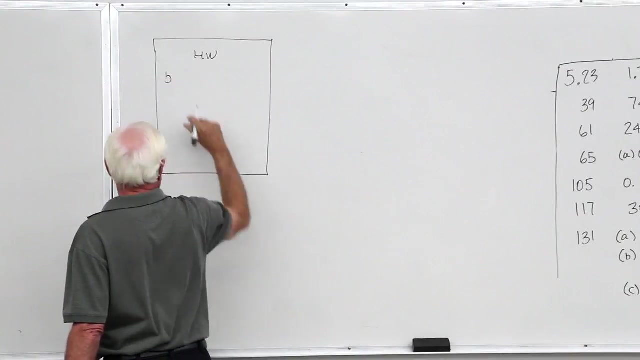 Yeah, that's. I'm going to change this. Excuse me, Sorry about that. This distance is H, capital H. This distance is little h. Okay, So here's my homework. I don't know how to make something. I'll say it's probably 459.. 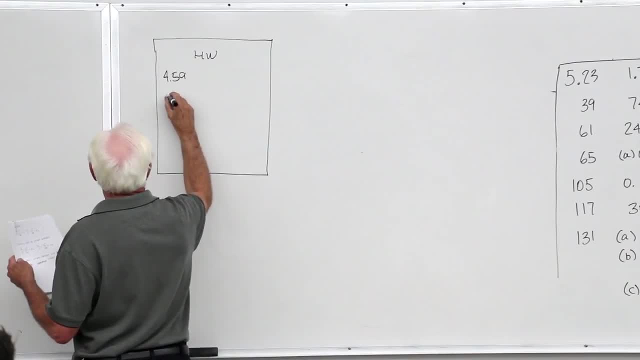 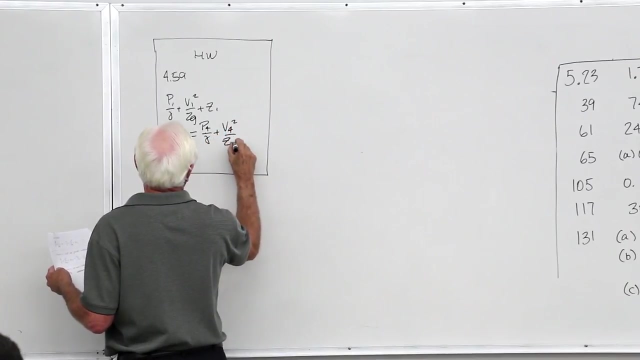 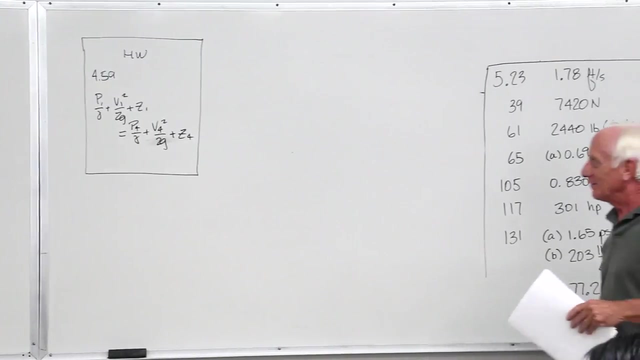 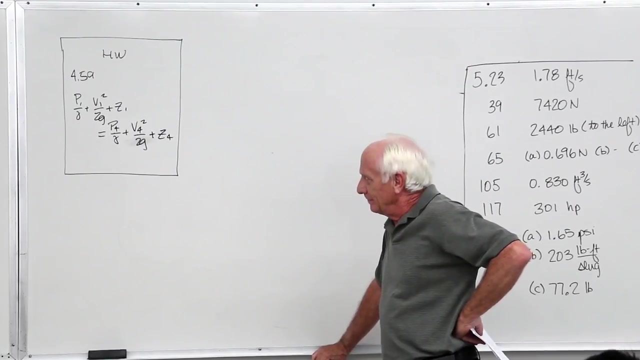 Okay, And then you write it down: Okay. Now, of course that's bad, Because when you start there, if there's something wrong with your work- and I'm trying to find out what's wrong with your work- I'll say: where is 0.4?? 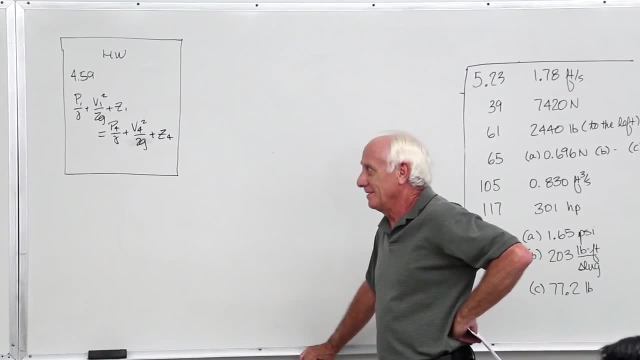 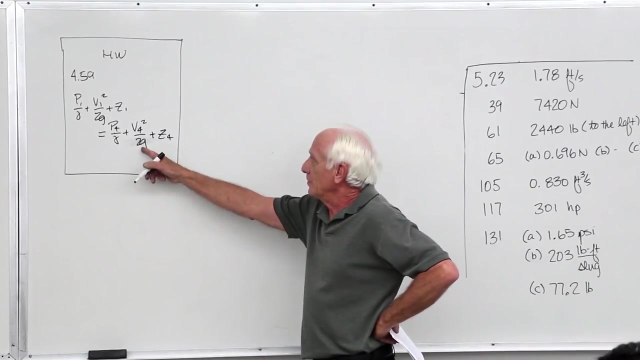 Matter of fact, you know what? I don't even see a picture. Oh yeah, that's bad. If you want to maximize your points on an exam, you better tell the instructor, and that's me, where these guys are, Because if you're, if you have a small error somewhere, just a small. you put G 32.2,. 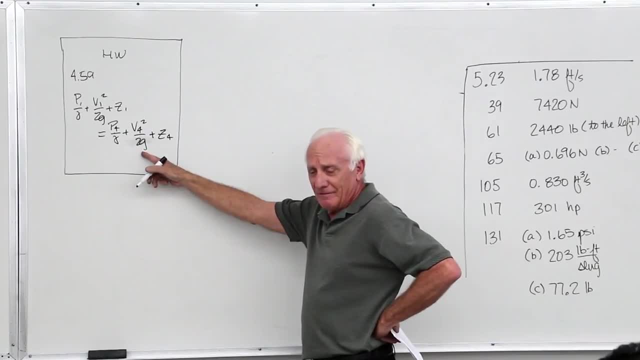 and that's it. That's a high problem. It's not major. But if I can't find that error, what's my choice? Take off a lot of points. I can't find it, So here's a lesson, then. 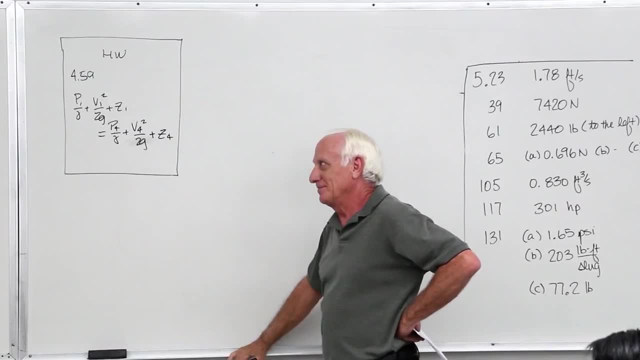 First of all, these guys all require sketches. And on an exam, especially on an exam, how do you clear your mind? You draw a sketch. Most engineers love to see a sketch. They hate to see a spreadsheet. Spreadsheets are boring, Sketches are interesting. 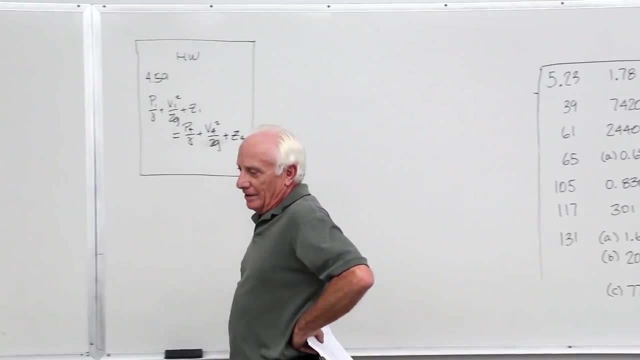 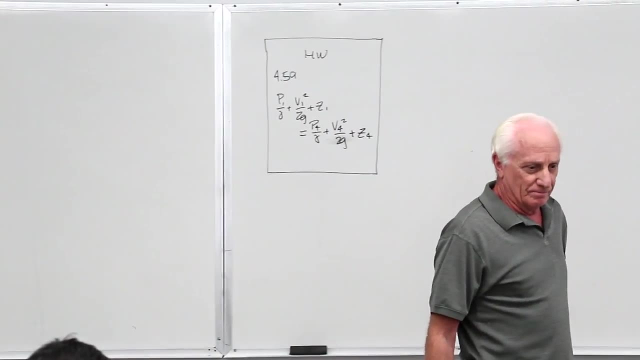 Go to a meeting of SAE or ASME in Detroit or Atlanta, Have a nice lunch there at the hotel, then go into a room. The guy turns the lights down on the room. He's got a 20-minute talk. 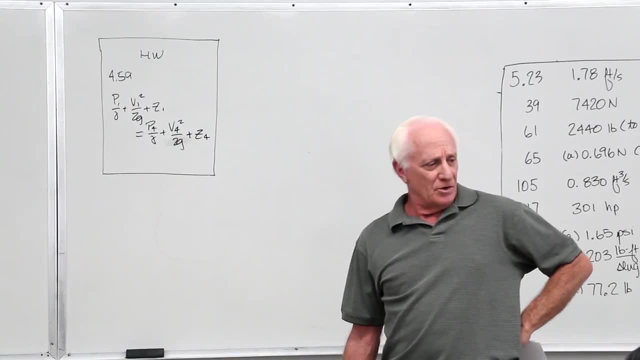 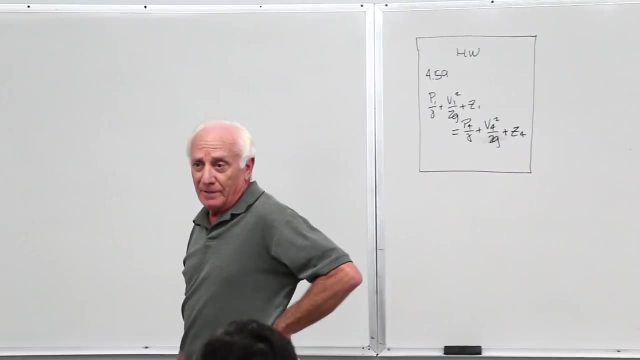 There was a spreadsheet guy. Everybody's yawning and snoring in the back room over there somewhere Because he had a big lunch and the spreadsheets don't excite. no, if you're a math major I love them. but I mean, if you're a math major then maybe they excite you. But I'll tell you what. 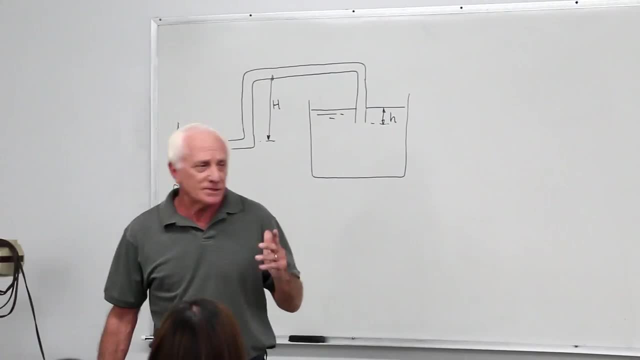 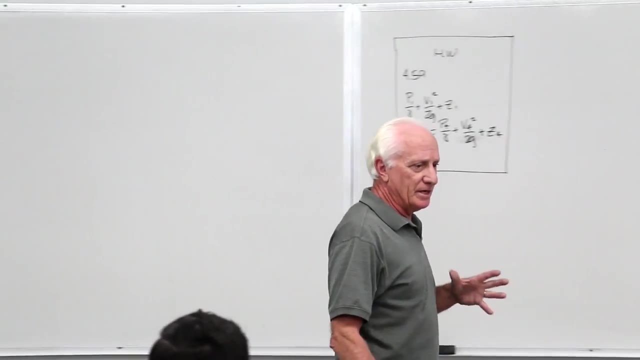 you put a multicolored graph up there, everybody says: what's that supposed to tell me? What's he trying to tell me by that graph? Oh, it gets your interest, Keeps people awake. See, we engineers are graphic type people too. We love numbers. 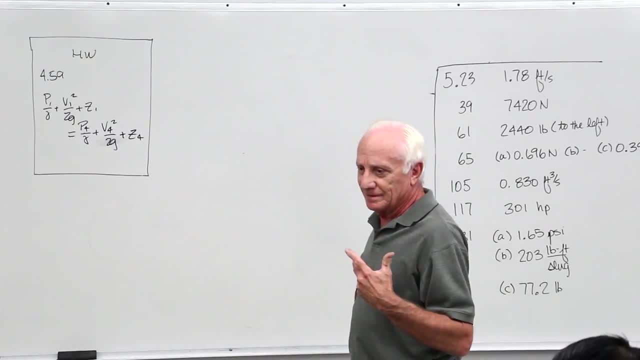 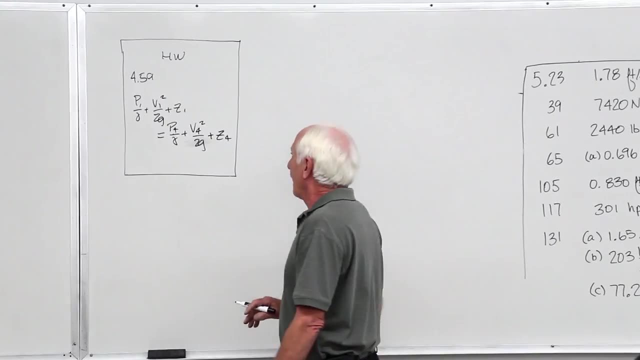 too, but we're not math majors, So sketches get our interest and they also guide us to the right solution, Okay. so number one is: draw a sketch, Okay. Number two: okay, I drew the sketch. There it is, And there's the first equation written. 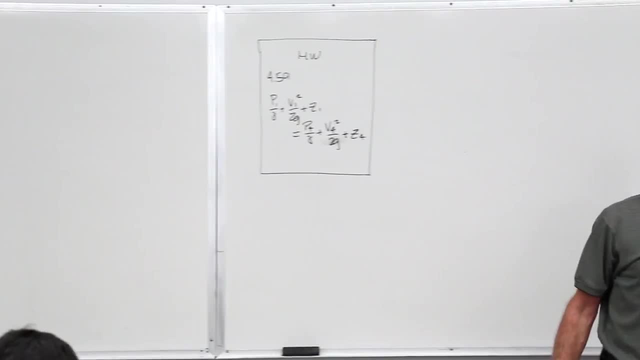 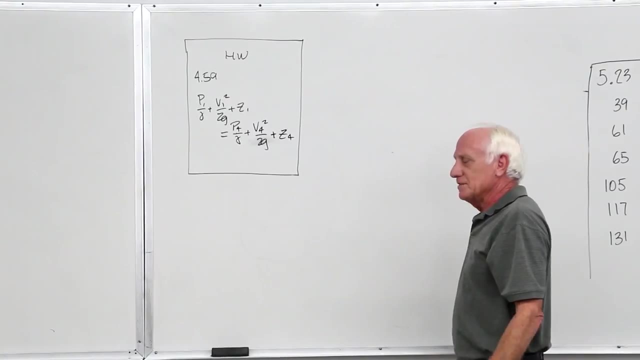 down And there's the error. The answer's wrong on an exam. And I say, oh, what did this guy do wrong? And I'll try and find it to the best of my ability. And if it's not clear to me, I say: you know what? You're not making any sense, I can't give. 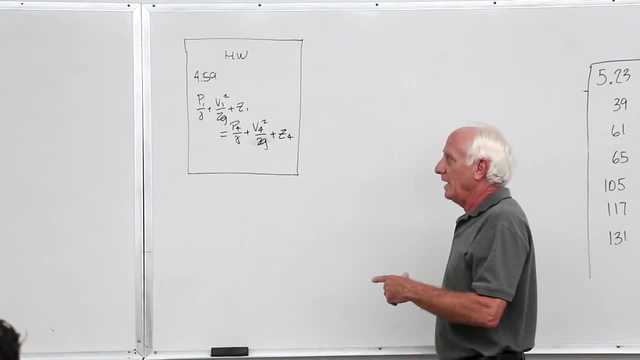 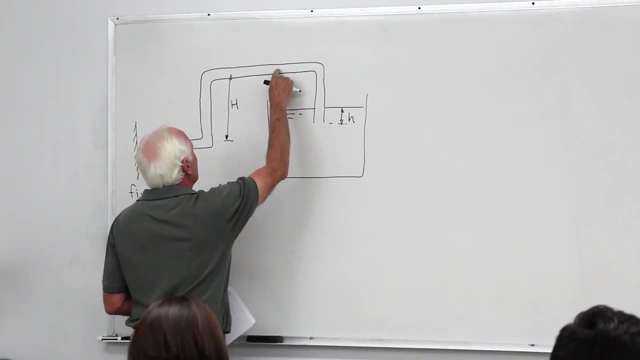 you partial credit. You don't deserve it. Well, you know why? Because I'm trying to find point four. over here Is point four at the bottom, At the entrance, At the top, At the exit, At the wall. I'm not going to guess. 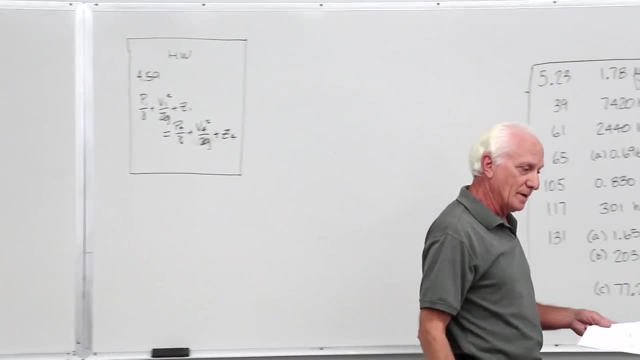 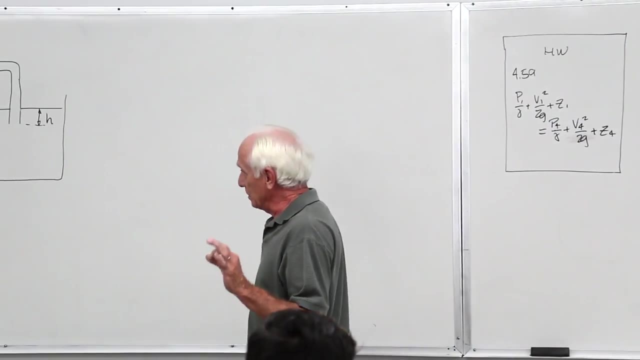 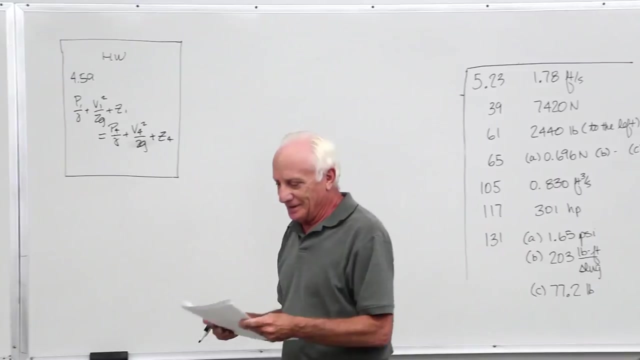 That's not my job, So you got to help me. Plus the fact, that's just the way we engineers are: If we're not precise, we're in the wrong major. So what you do is you put numbers on that guy, Okay, so first of all you draw the picture, Then you put. 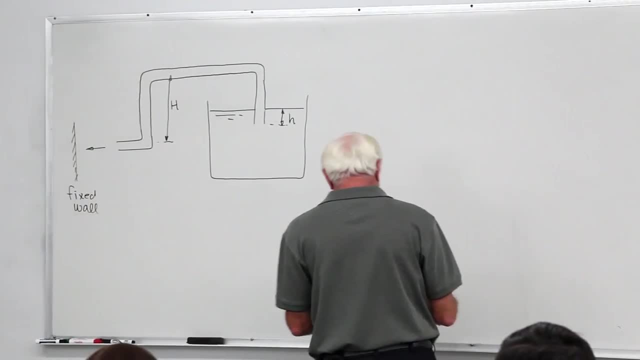 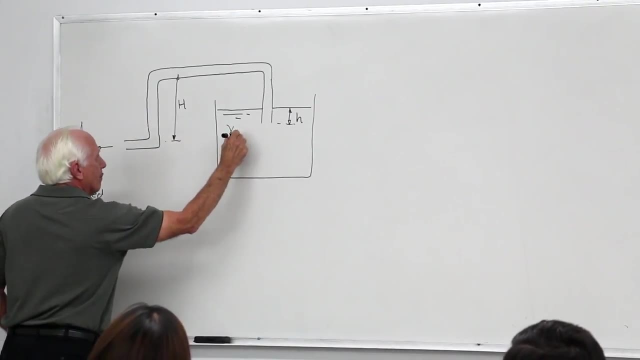 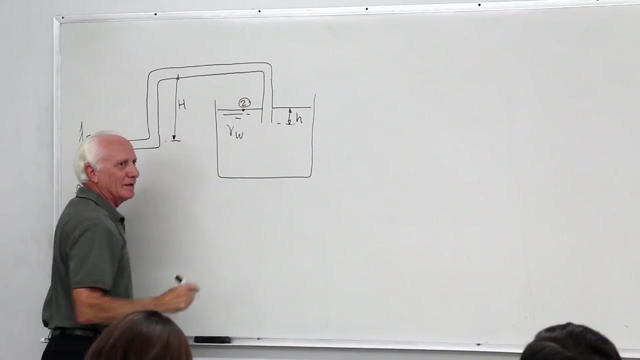 the numbers on there And don't do it this way. Say: you know what. The water strikes the wall right here. I'm going to call that one and I'm going to call that two. Why in the world would you do that? Maybe you read the book backwards. 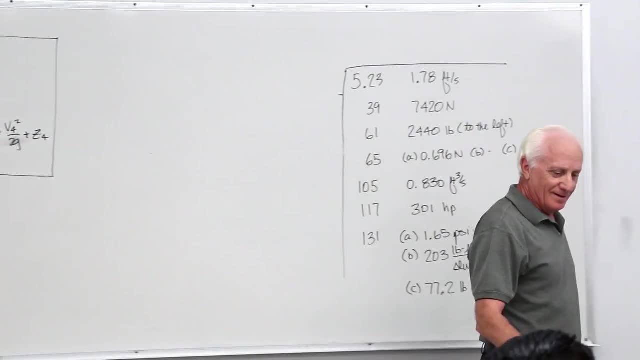 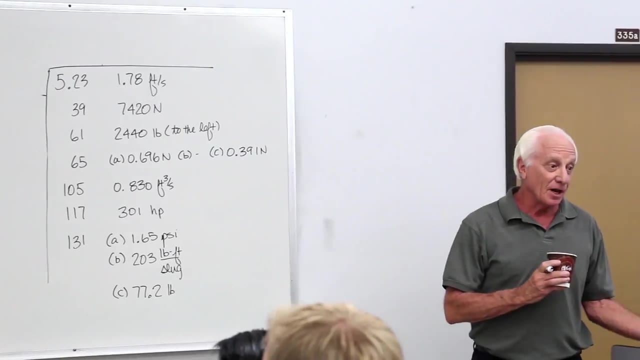 from the back page to the front page. Maybe I don't know, But hey, you know what Number it in a sequence from where the flow starts to where the flow ends up. That's the logical sequence. The logical sequence. Oh, you'll get the right answer. You'll get the right. 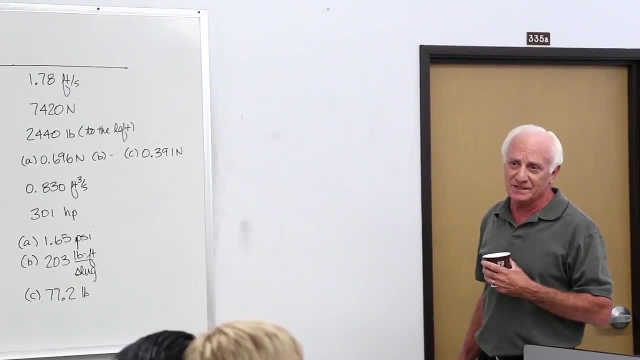 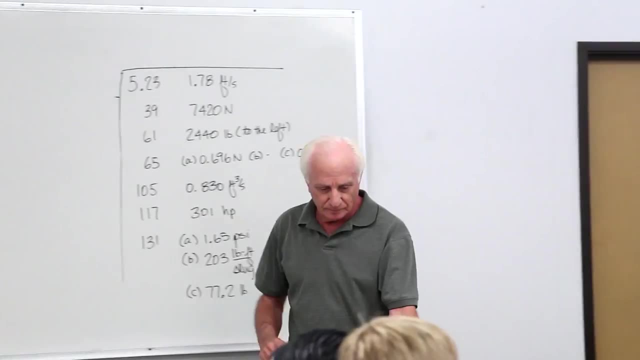 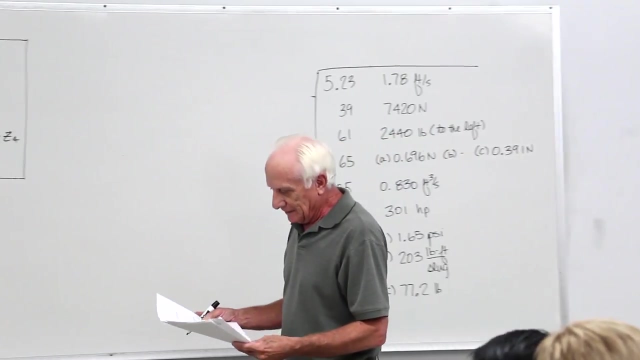 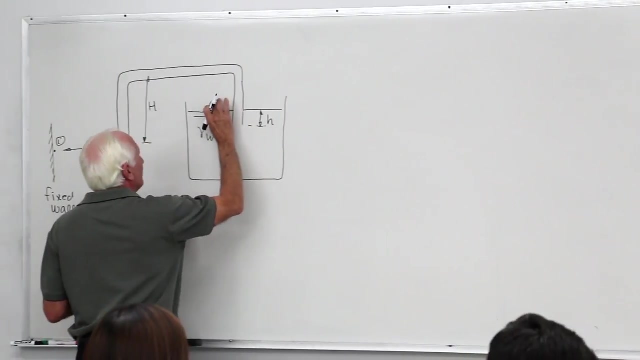 answer, But it's nonsensical. It shows something's missing. Okay, So I'm going to number the points, as you hope, logic prevails And let's see. We can start with number one, where the flow initiates. And, of course, why do you choose that point? Because you 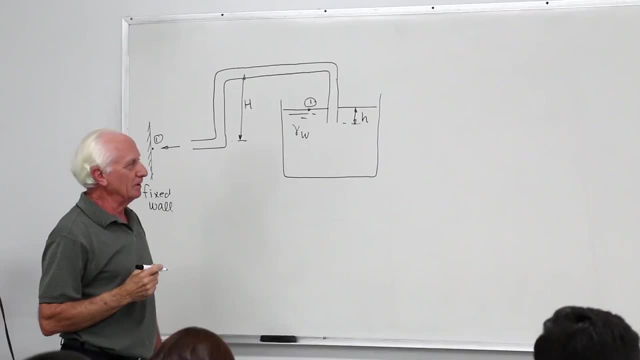 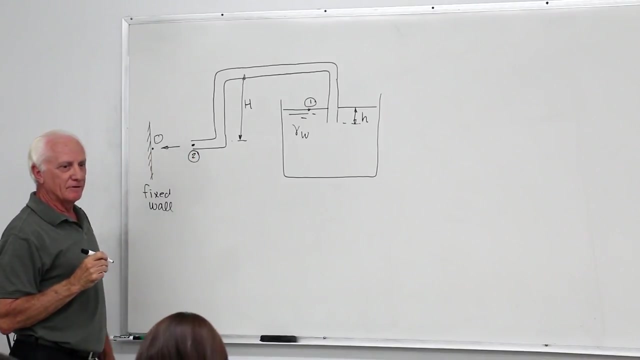 know the pressure there is zero, The velocity there is zero And you can typically find the elevation there. And the next logical point may be where the stuff comes out of the pipe. Of course that's a logical point. And the third logical point is where it hits the fixed wall. Because you may be asked for 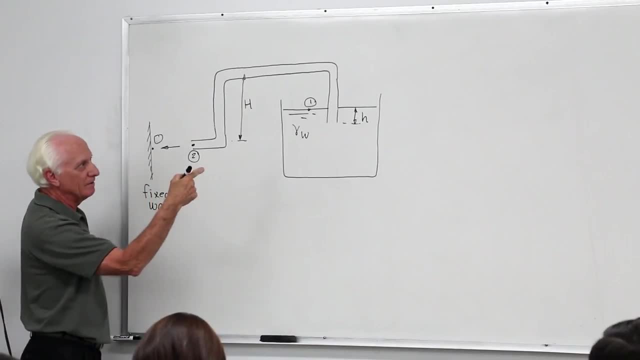 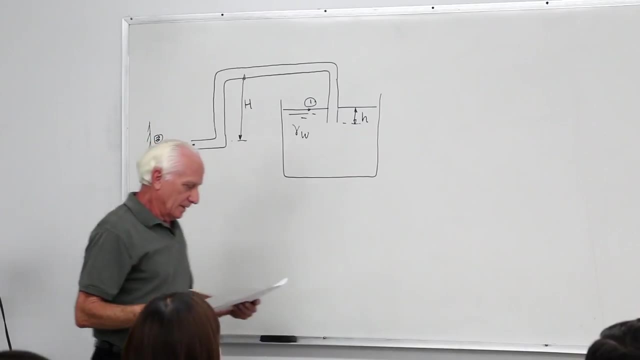 the stagnation pressure at the wall. Yeah, you have been. That's a problem. Whatever, it was 359.. There's three, Okay, So we have three of those guys Now. they're in the right sequence, They're numbered And 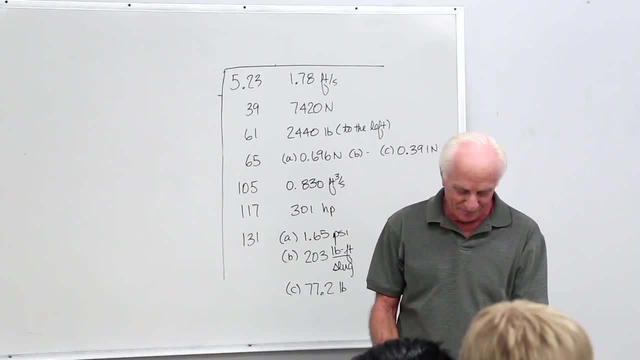 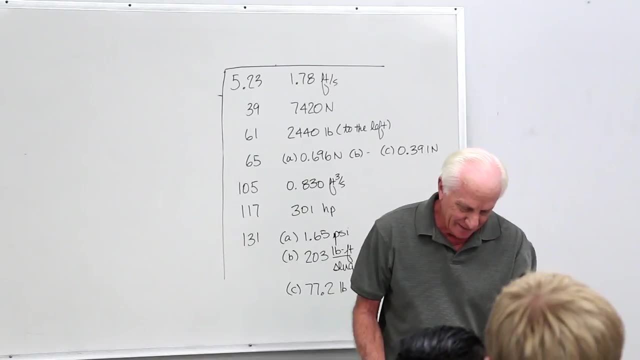 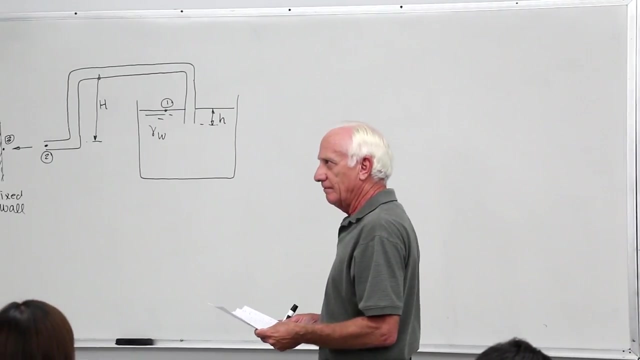 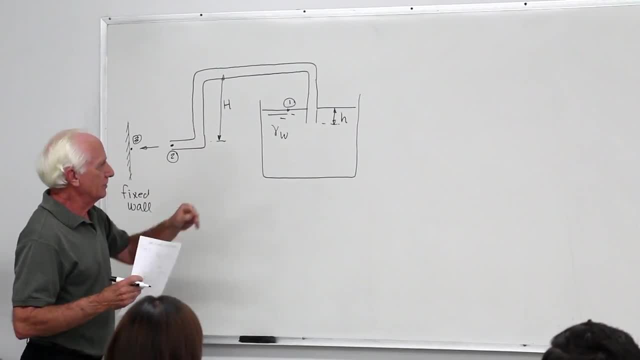 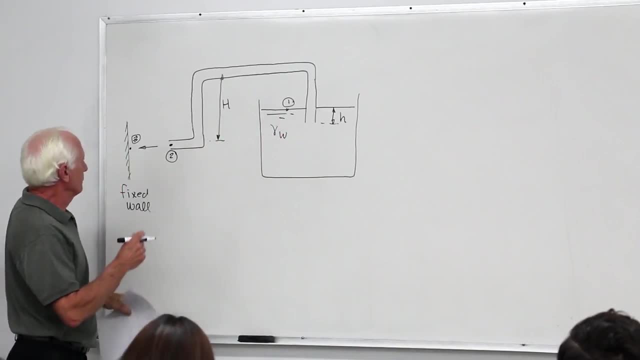 velocity: 0, and the elevation: we know that At the exit. 2. Pressure: Yeah, It's just outside the exit Atmosphere: 0.. Elevation Z: Yeah, We typically know it, It's given. 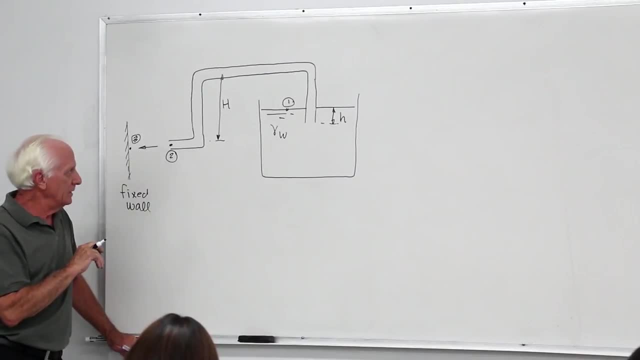 to us typically? Yes, we do. What's the only unknown in the equation? The velocity at 2.. Once you've got the velocity at 2, what does it do? It comes back. It comes back to 10.. Okay, 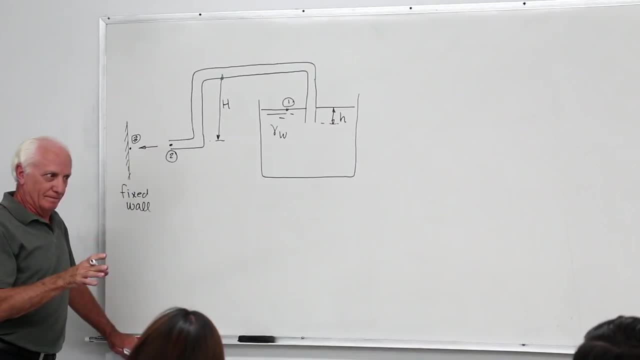 What is this? I'm a skeptic. It comes back. Yeah 10,000?. Yeah 10,000?. Posse of two. that's part of the problem. You want Q two. take V two times A two. 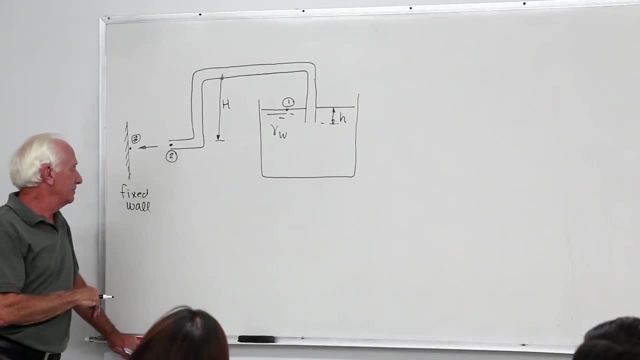 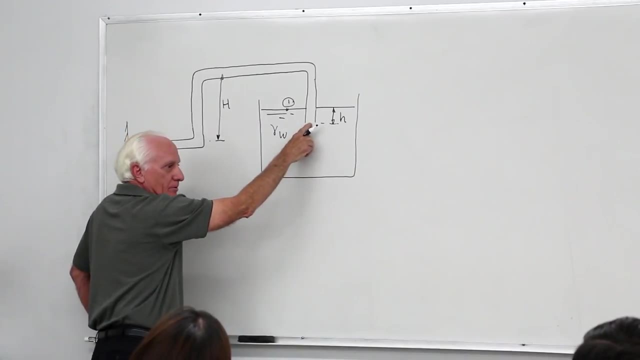 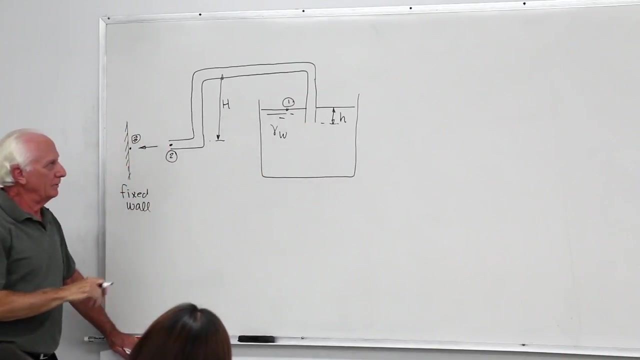 You want the mass flow rate. take rho A two, V two. You got it. so you got V Q m dot. What's the flow rate entering Q? the same Q Continuity, steady state M dot. same m dot as m dot two. why? 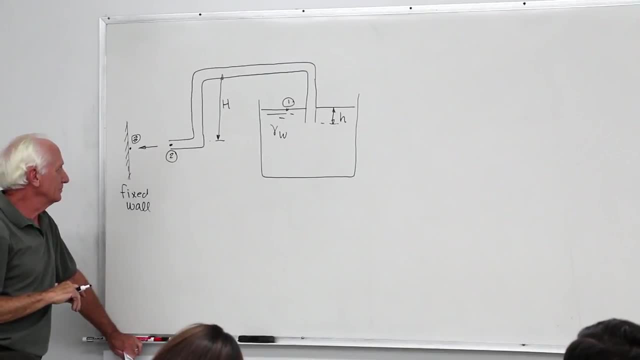 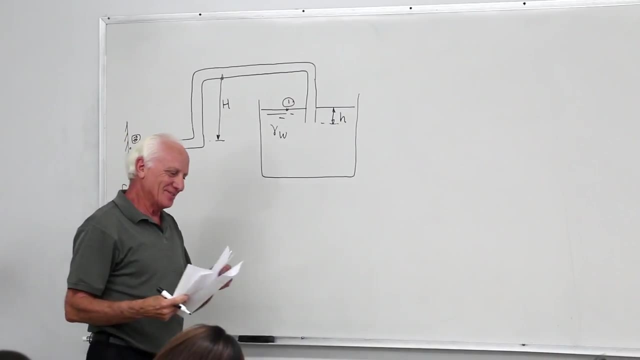 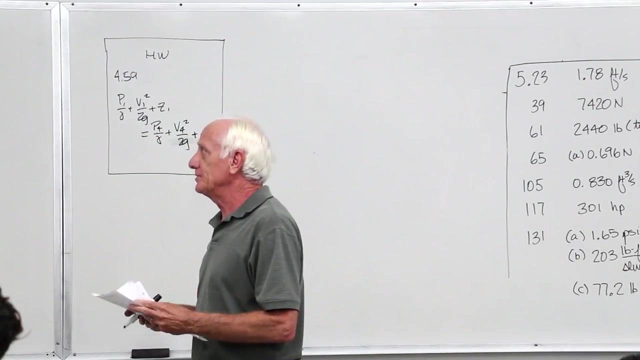 Continuity: steady state. Okay, I think that's all on that one. any question on that? So just help yourself, and especially when you're getting ready for the final. if you've got your homework done like this, I guarantee you'll save tons of time. 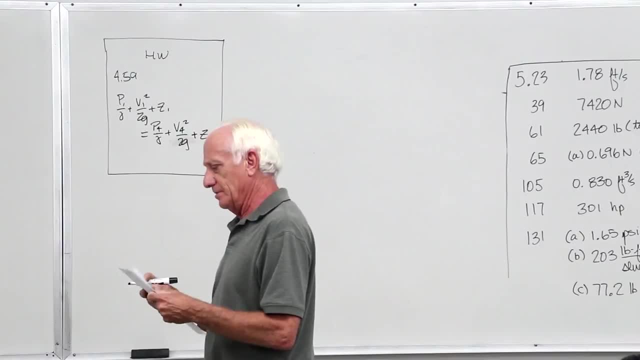 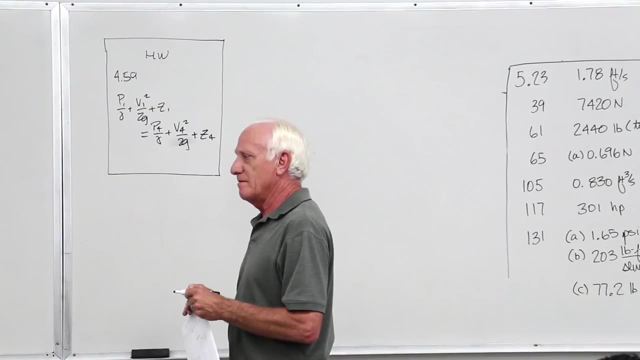 Otherwise you gotta go back to the book. look at the picture, figure out where points one and points two are. say, oh, I didn't put them on there for the homework. Well, you've gotta probably pay a price study for the final, yeah. 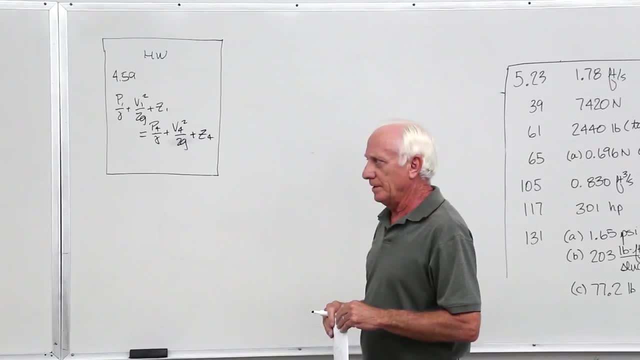 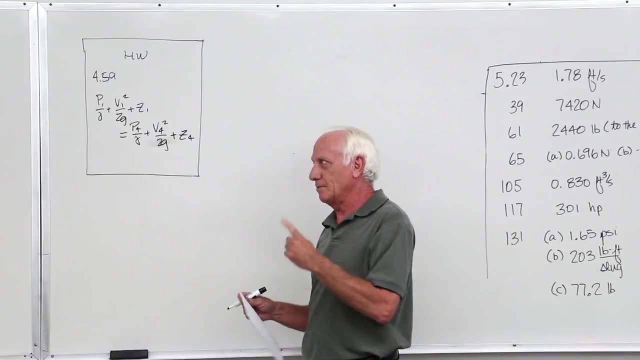 Everybody's busy. the last week All the projects are due. three finals: one Monday, two Tuesday, rest of the week's nothing. So you gotta find a way to budget your time efficiently and study efficiently. that's the way you do it. 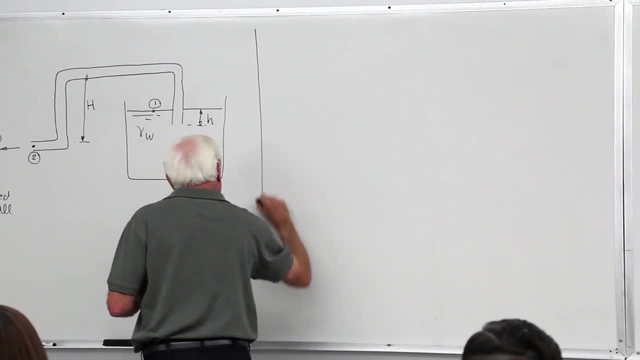 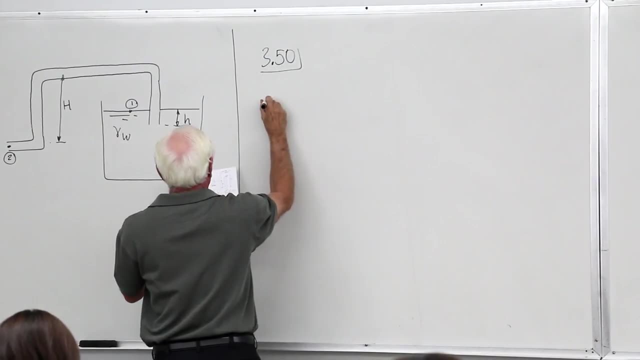 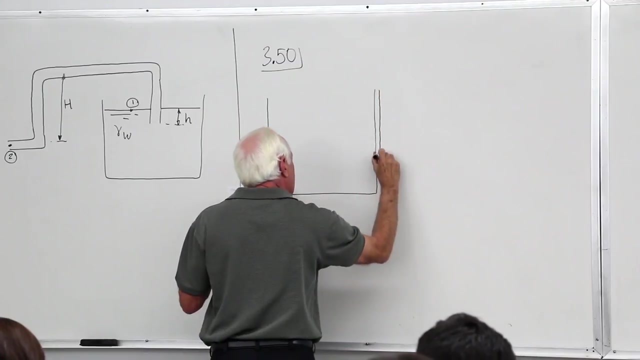 Okay, back to you. okay, let's save this guy. I might come back to him. Alright, let's look at problem 350.. This is the problem. Okay, We have. oh, let's see, I guess I made that, yeah. 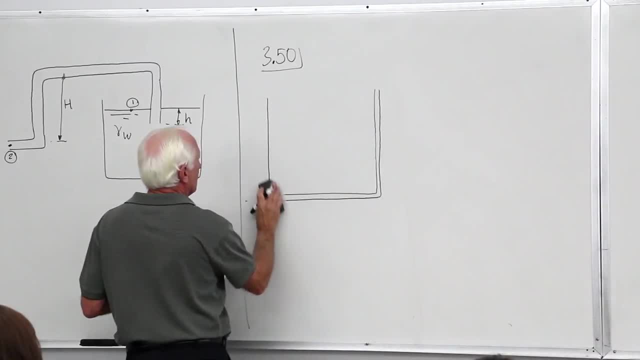 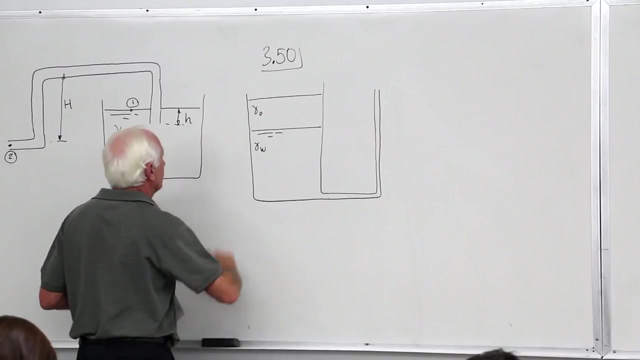 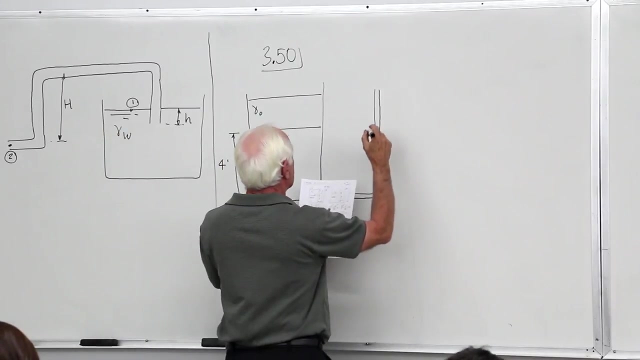 I think I made that wrong. There's a reservoir here. Okay, let's see. the water is right here. Oil is above it. We know this is four feet, This is four feet above here, And we know that there's a nozzle up here. 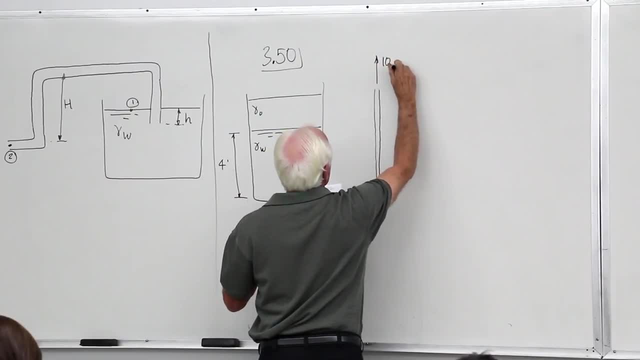 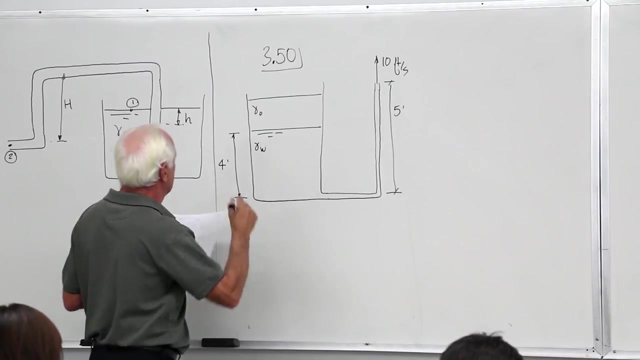 where the water comes out at 10 feet per second. Okay, Okay, Okay, Okay, Okay, But we know that's five. Okay, And let's see what else, Oh, where. oh, this is, oh, this distance here. 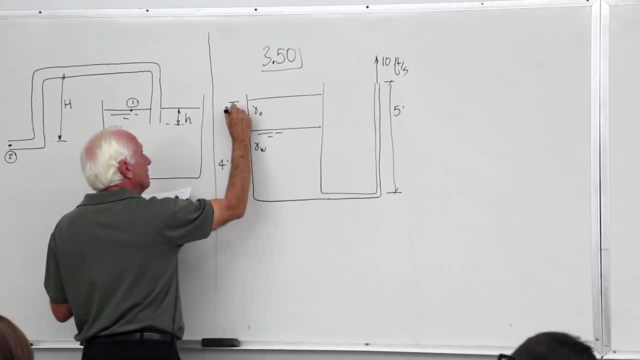 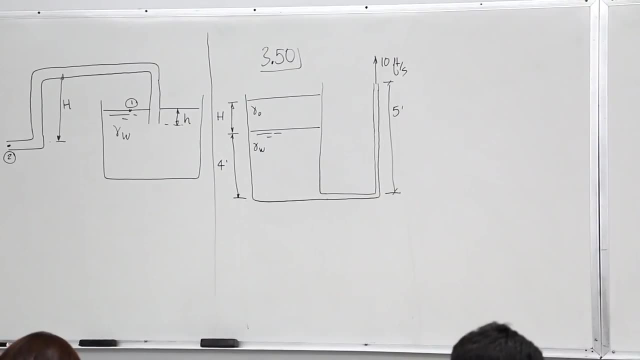 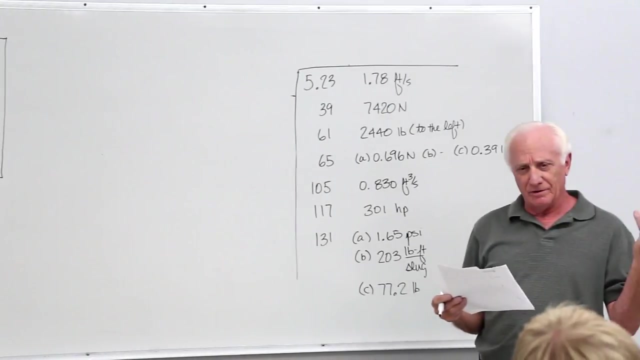 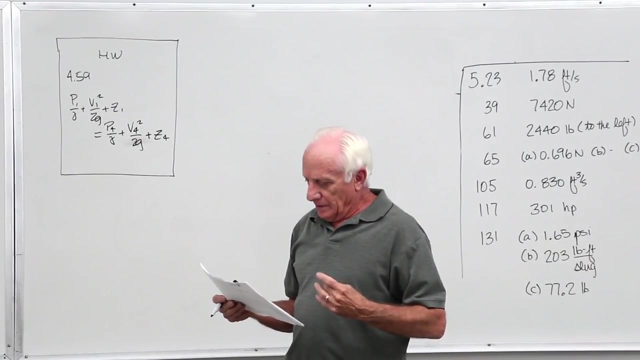 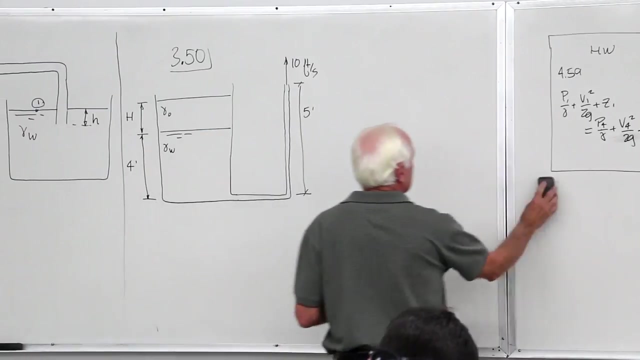 Yeah, it's h. I guess we didn't know h the. yeah, here it is. Yeah, find the depth H of the. I think it's oil or kerosene or something. It's got a gamma of 50.. It's a light oil, maybe. Okay. 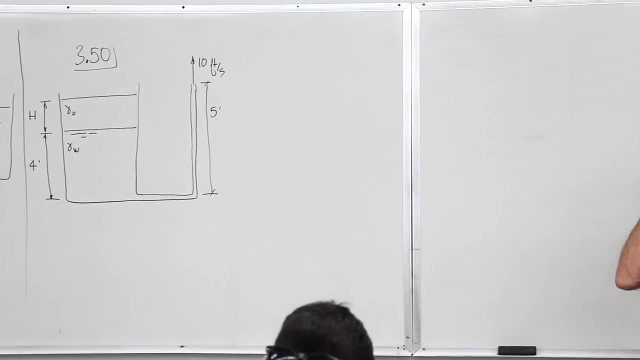 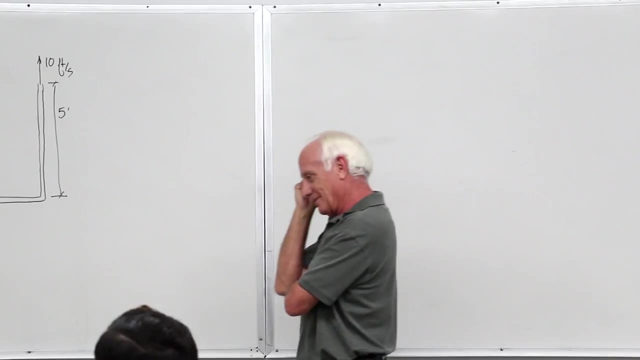 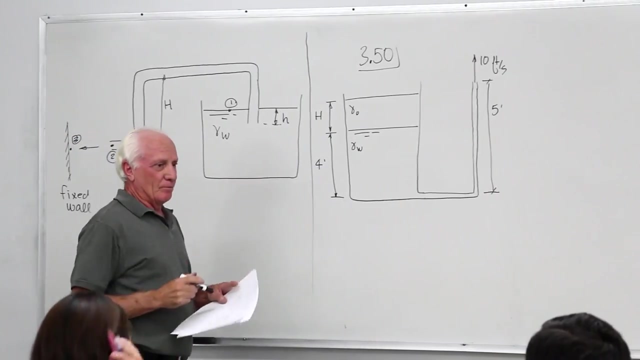 You have to assume it's incompressible, It's steady-state, It's inviscid. When you make those assumptions, then you can write Bernoulli's Okay From point one to point two, And then you have to put point one and point two somewhere, Okay. 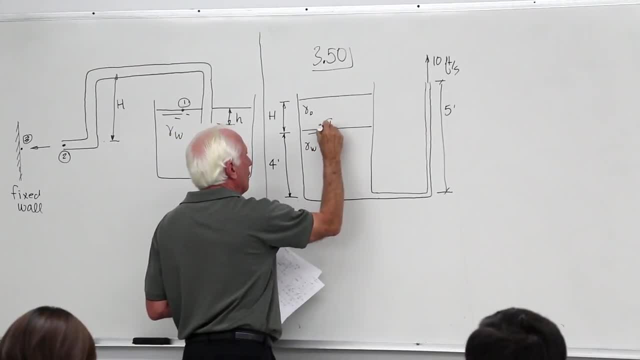 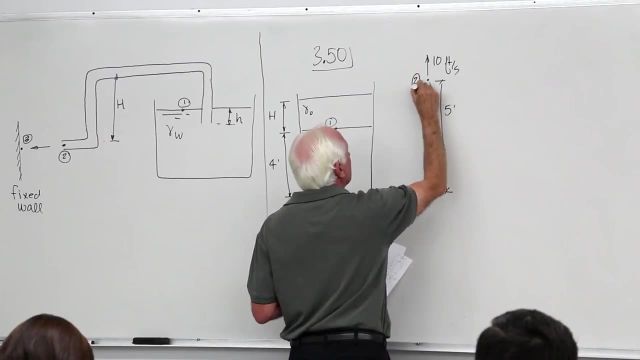 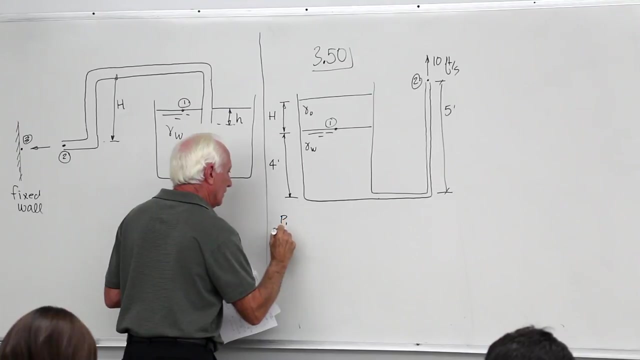 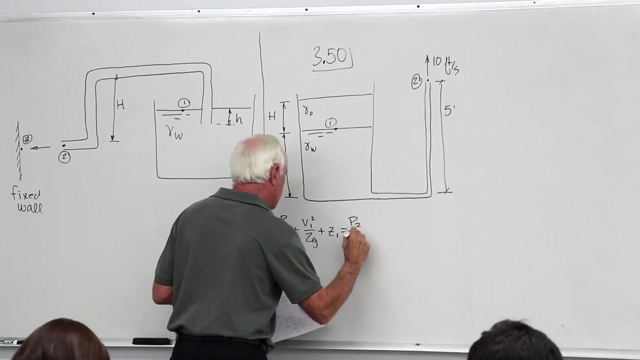 I choose to put point one here And I choose to put point two where it is right here. Okay, P1 over gamma, V1 squared over 2G, Z1, P2, V2, Z2.. At the exit, pressure's. 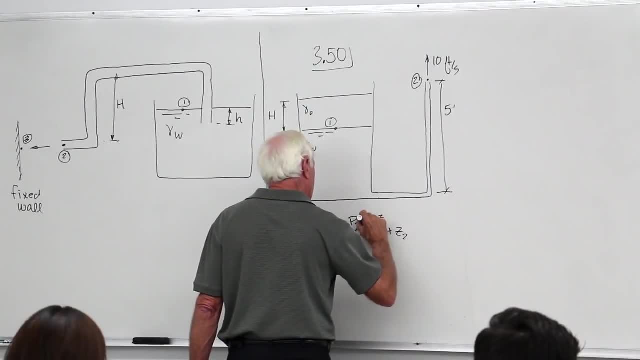 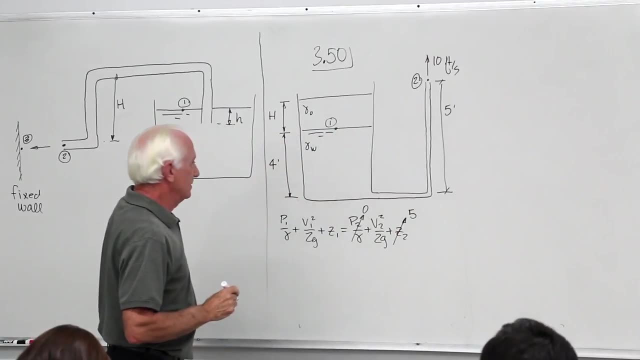 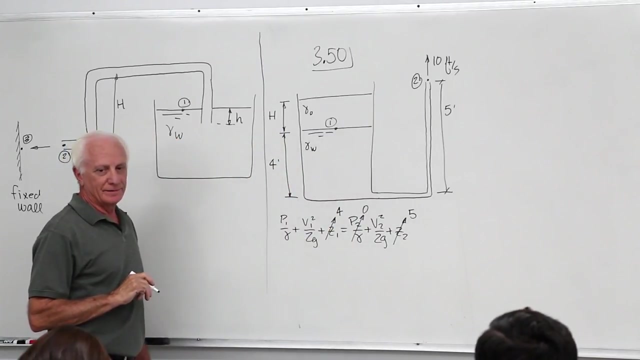 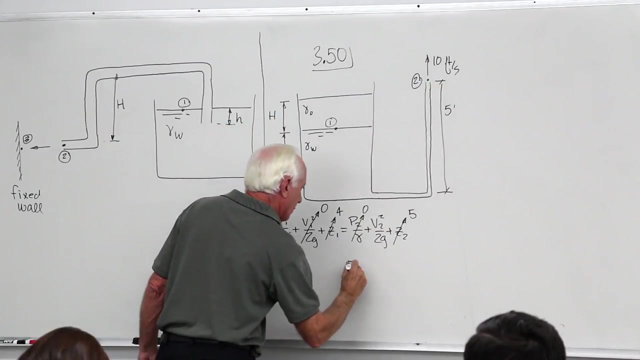 atmospheric: 8 to 0.. Z2, 5, Z1, 4, V1, 0.. Find H: Oh, I've got, I've got, I've got 10 squared P1 over gamma, V1 squared over 2G, Z2, 5.. 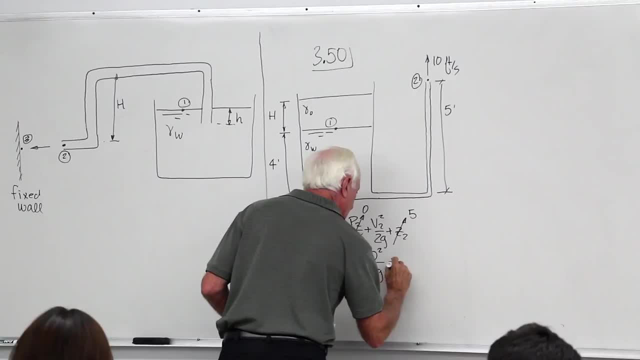 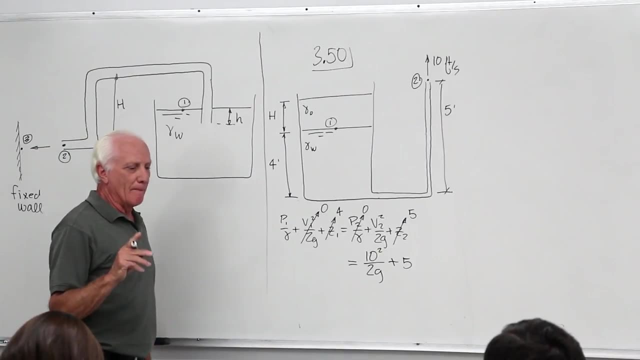 P1.. Is the oil moving? Is the oil moving? No. Chapter two: fluid static. yes, I go down. how far down Capital H. What's the fluid Oil? gamma oil H down plus. 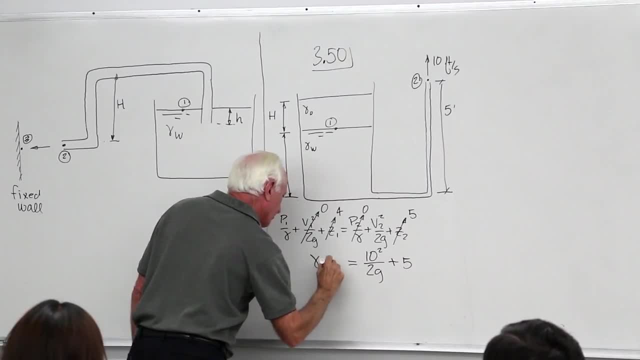 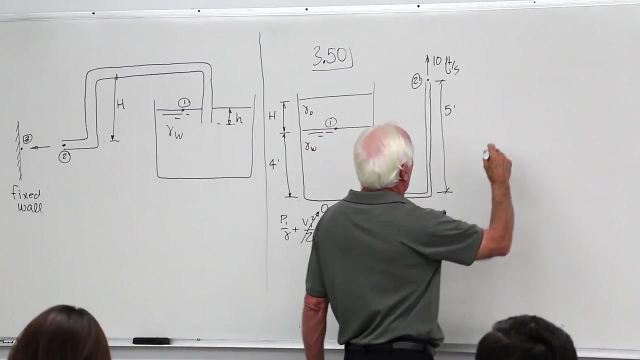 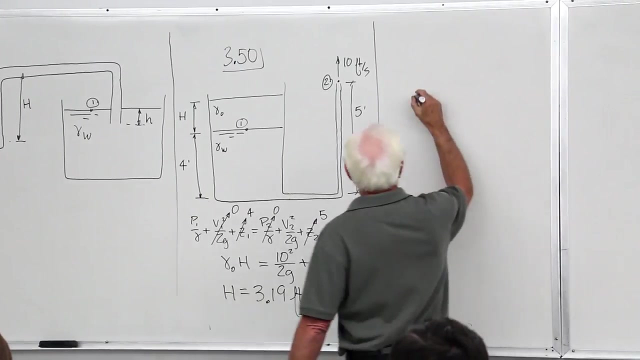 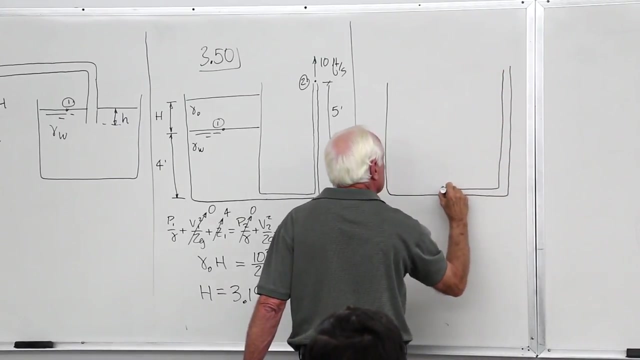 plus, Okay, Do I know gamma oil? Sure, I do. It's 50.. That's the way Joe did it. Mary did it this way. Hmm, Okay, Okay, Okay, Okay, Oh, I've got 10.. 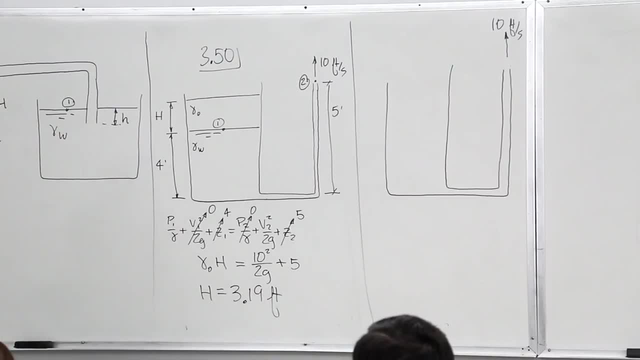 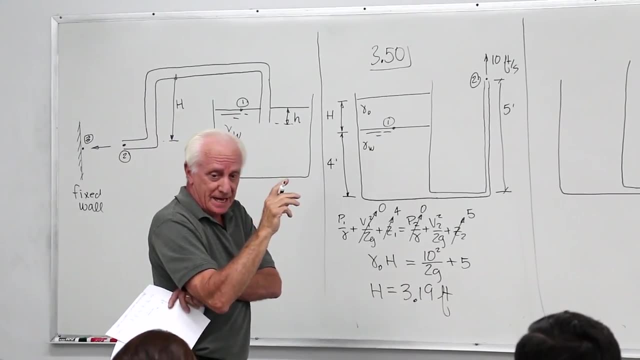 Mary said. you know, in my past Professor Biddle said you can replace the oil with the equivalent layer of water and then treat the whole thing as water. Now it can't be moving. to do that It's got to be fluid statics. Is the oil moving? No, 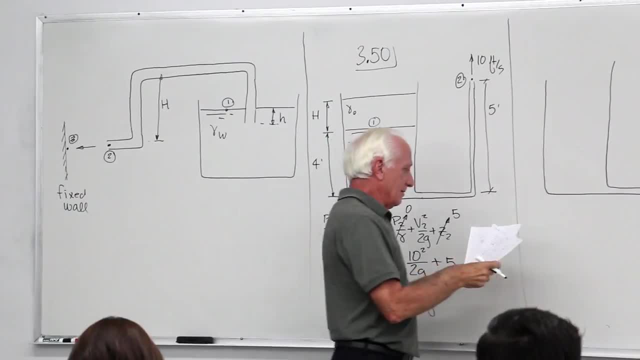 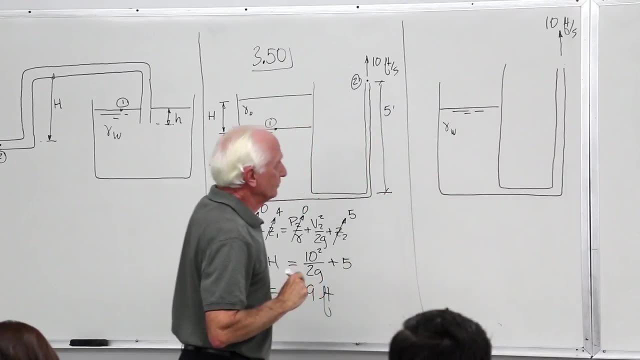 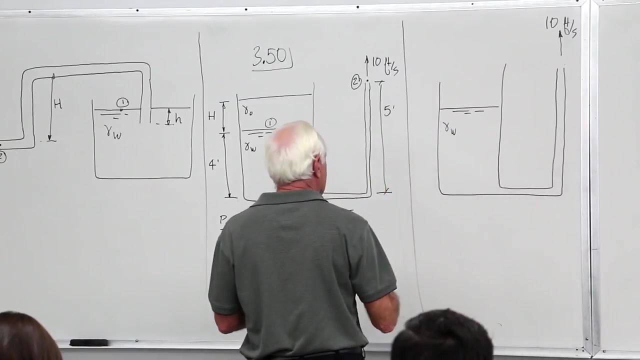 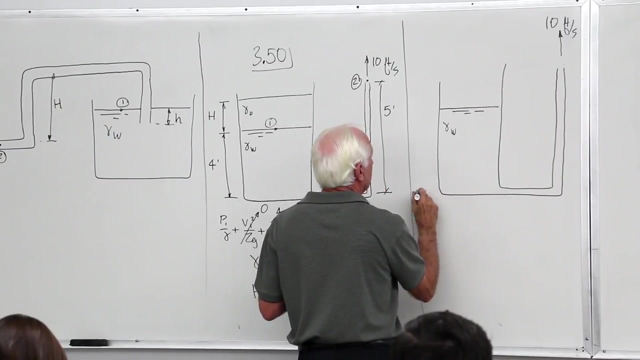 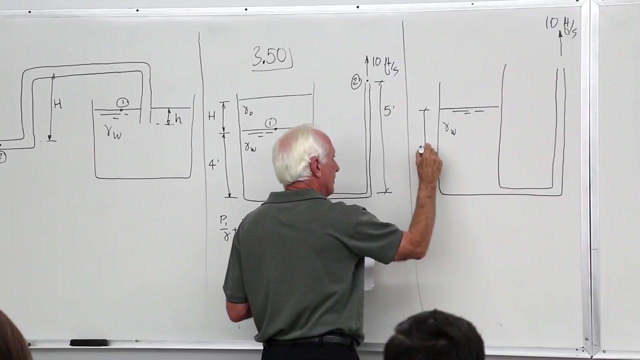 So we can do it, Okay. So now we do it this way, Okay, and now it's all. water comes off there. the height will call the height there, from here to here. okay, I'm going to show you that right here. that is, it's full. 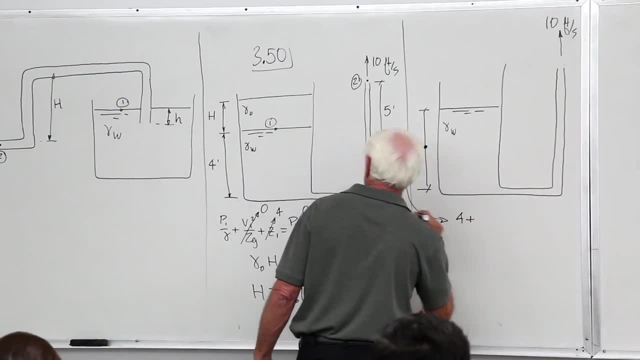 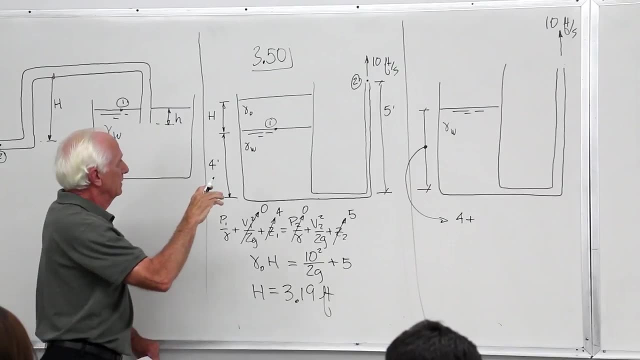 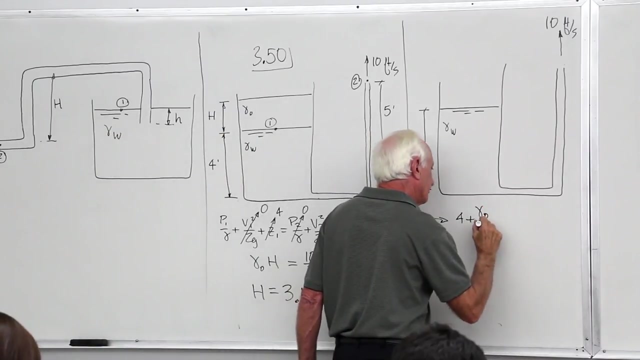 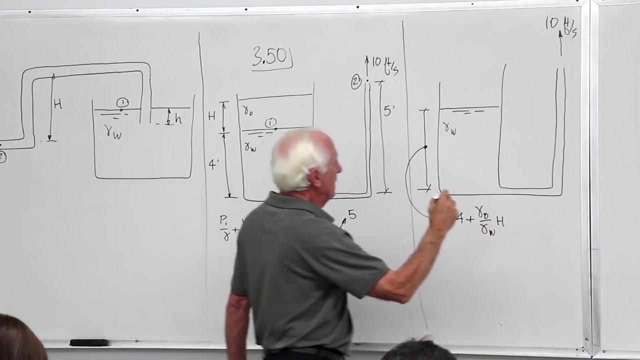 or plus. now, don't forget, when we get the oil up, we're going to replace it with the equivalent layer of water. so we take the ratio gamma oil over gamma water times H. okay, there it is, this guy up here he's. he's still five of. 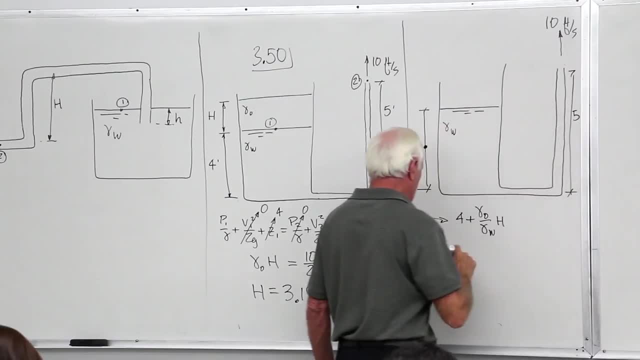 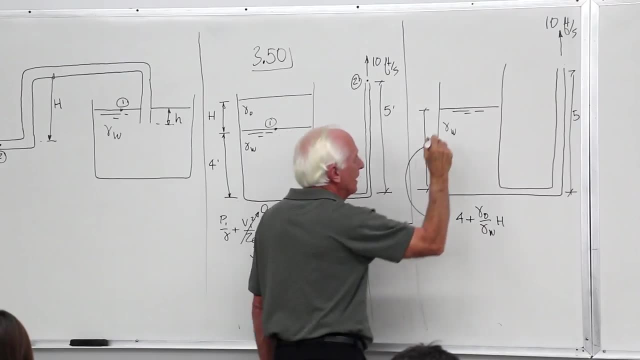 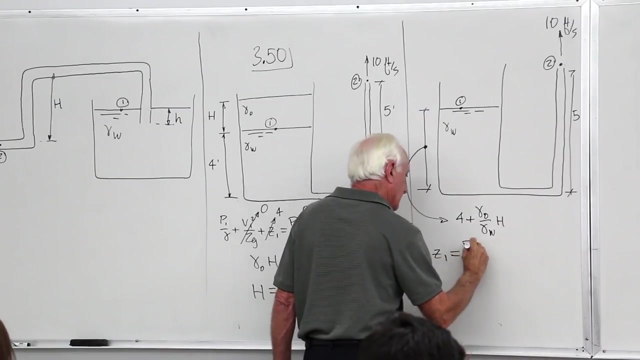 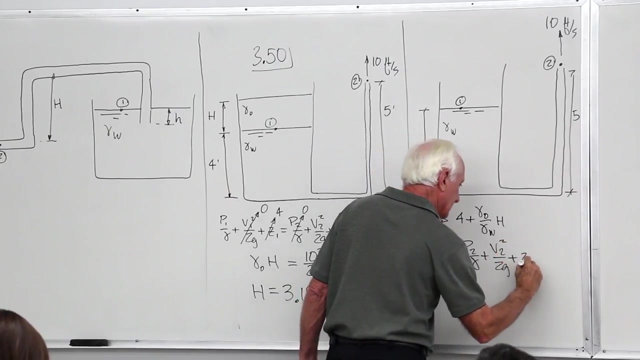 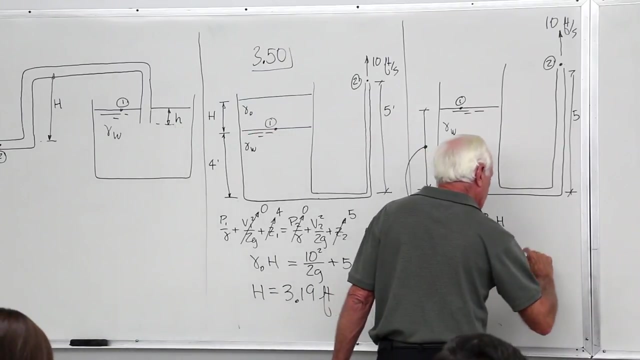 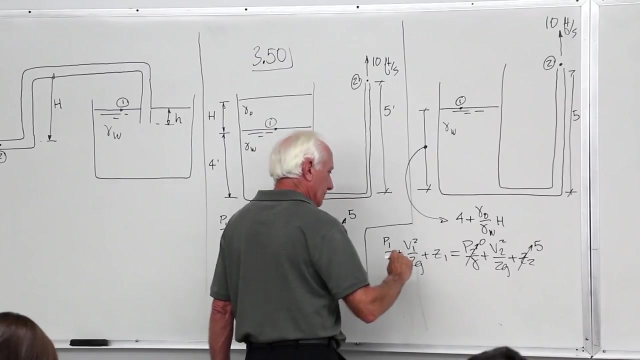 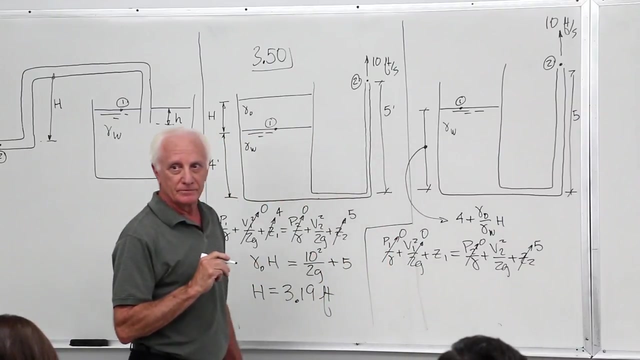 course. okay. where's point one now, at the top of the water? where's point two, just outside the jet? p1 over gamma, v1, z1, p2, v2, free jet at two pressure, zero, atmospheric gone, z2, still five, v2, I know it's ten- v10, p1, one, zero on the free surface of water. here comes the one. this: 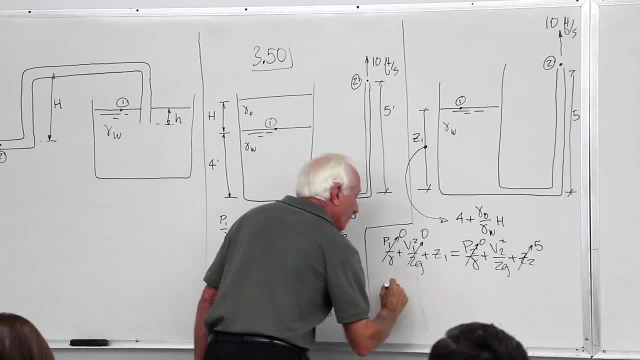 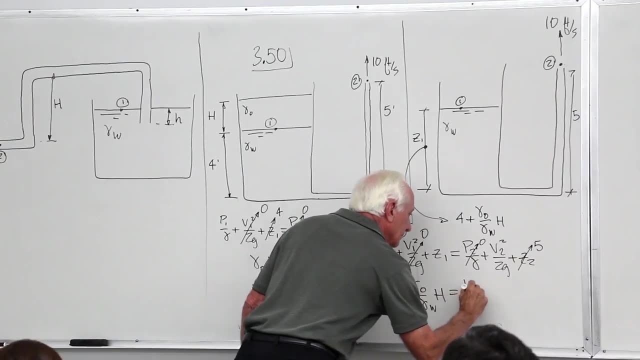 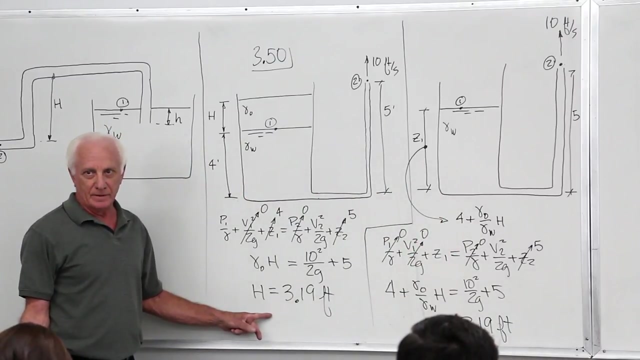 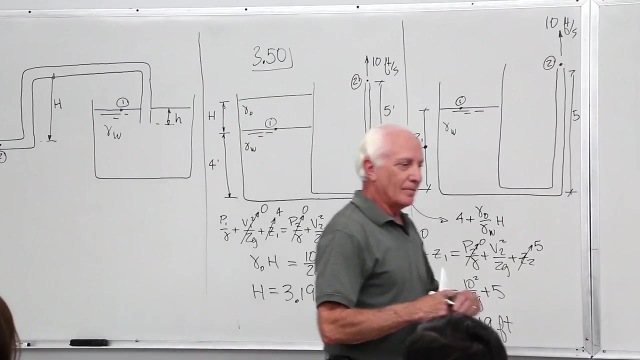 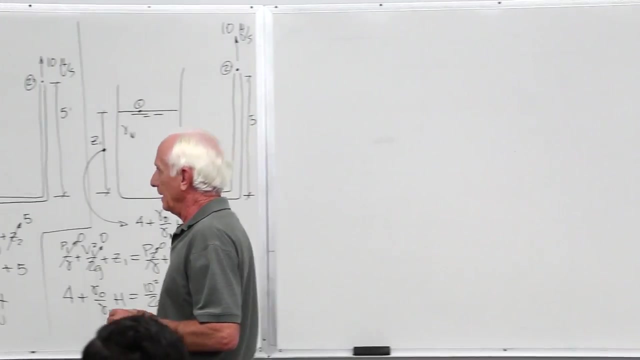 is, by the way, z14 plus gamma oil over gamma water, H equal 10 squared over 2g plus 5 H is equal to 3.19 feet. it gives the same answer. some people work at one way, some work the other way, but some people weren't very good at what they that, what they were. 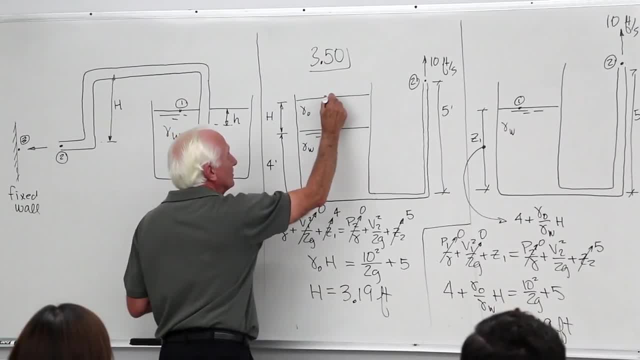 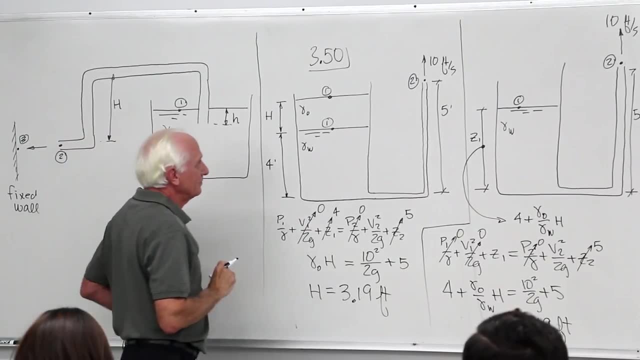 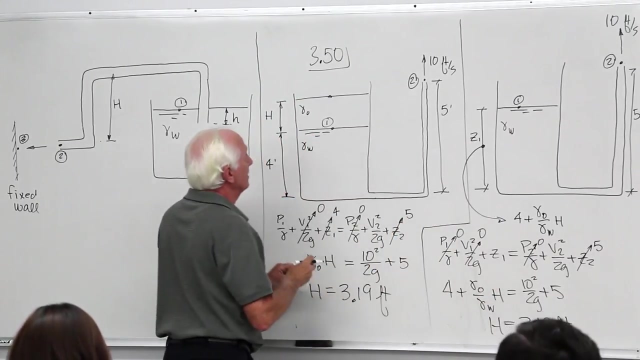 saying: you know, sometimes some people over put point one up there, no, don't put point one up there, no, no, don't go there. some people, when they solve it this way over here with the equivalent lay of water, they still think they didn't label that point one. they still showed point one over here. 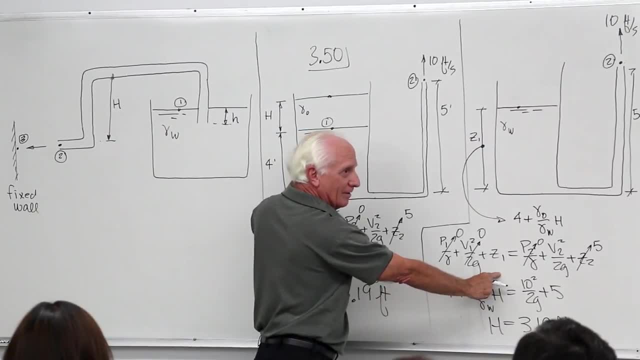 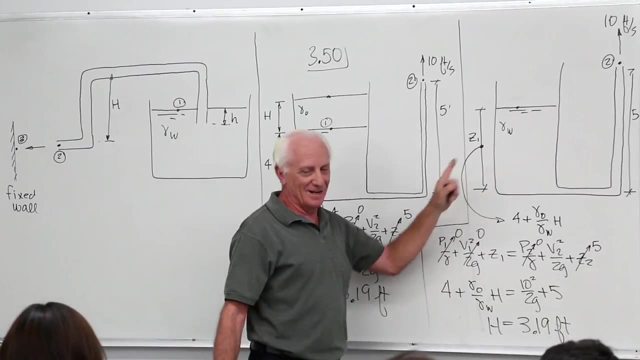 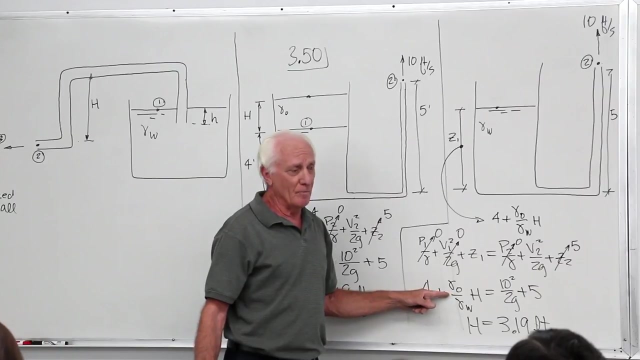 you, they should, they should point one with that equation: oh, that's not good. that's not good. if you're gonna do it that way, you better draw. my lesson is: you better draw a new picture or I'm gonna get maybe confused. great homework and exams. you better help you all you. can you draw a new picture? 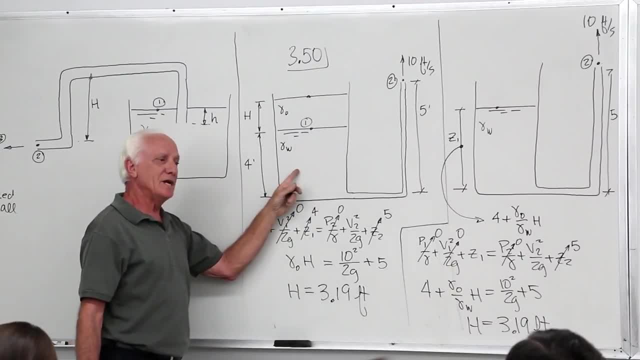 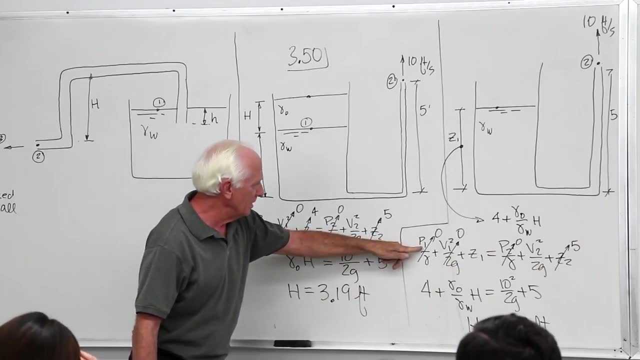 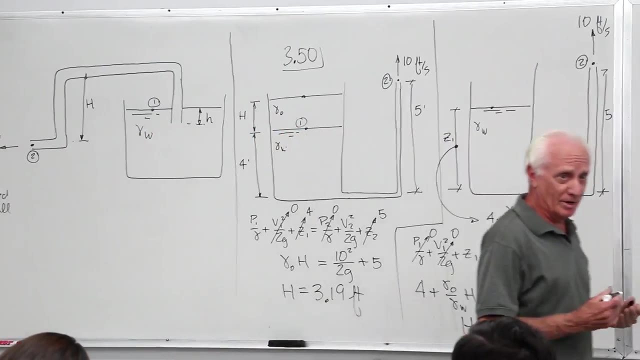 if you want to do it this way, fine, you don't need a new picture. you want to try and put this equation right here with that picture? oh no, I say point point one, point ones up is here. that's not right. several people at the wrong location for homework. just be careful. these are little things that when you 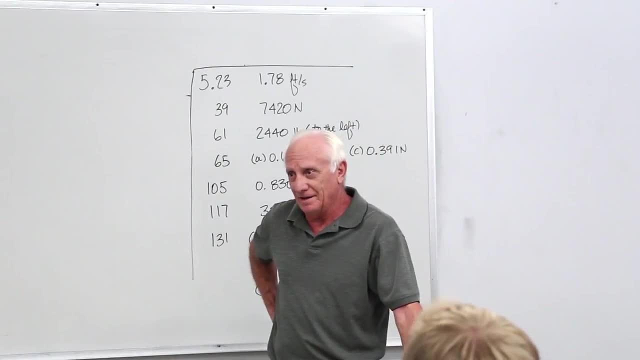 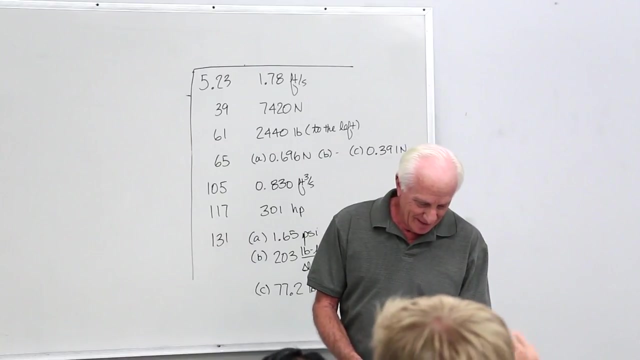 add the points. you go from a 91 to a 78. I just yeah, I know, just be careful, try and be. be a little more cautious on it. job, draw up another picture. okay, let's look at another one. sure, how did you switch in the first? 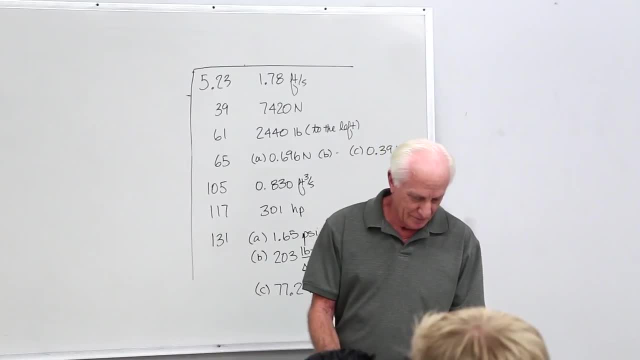 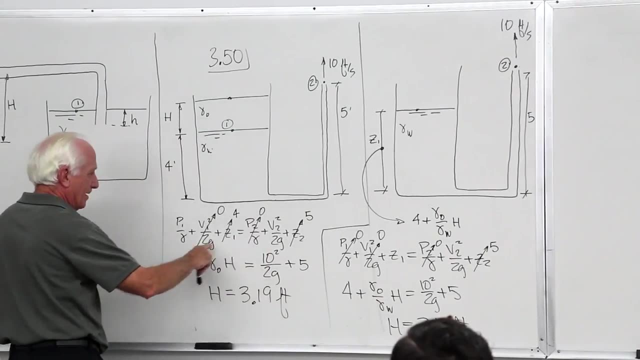 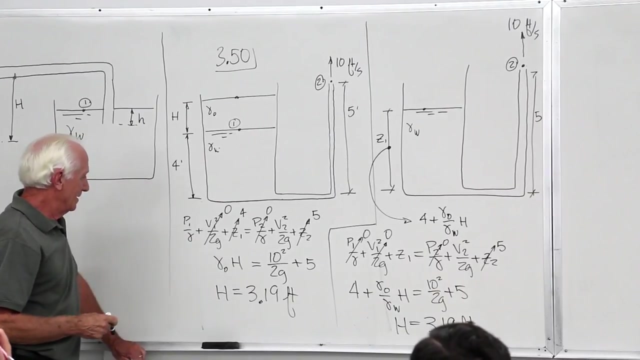 picture p1 over here. yes, you want to know. to look on the left side here, equation: yeah, just a little bit more over there. there you, yeah, how do you turn that into? is that alpha, or I forget what that's called? yeah, gamma, gamma, gamma, gamma, knock times. okay, yeah, this is. this is a good point. thank you here's. 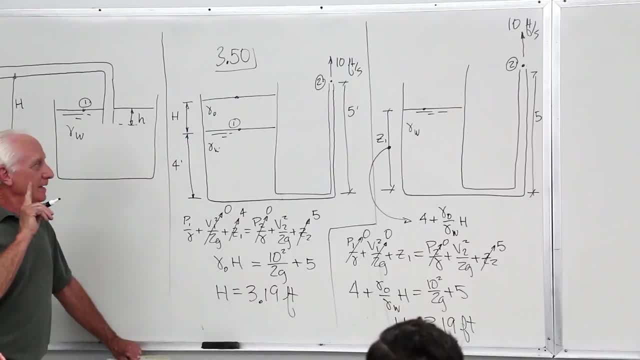 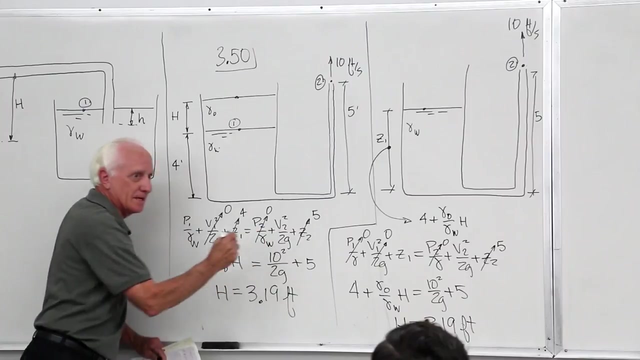 here's a deal. you gotta be real careful. there's two gammas there. here's the deal. Bernoulli's is applied to a fluid in motion. look at that picture. tell me what's moving: oil or water. thank you, that's how you tell us. go, sir, but 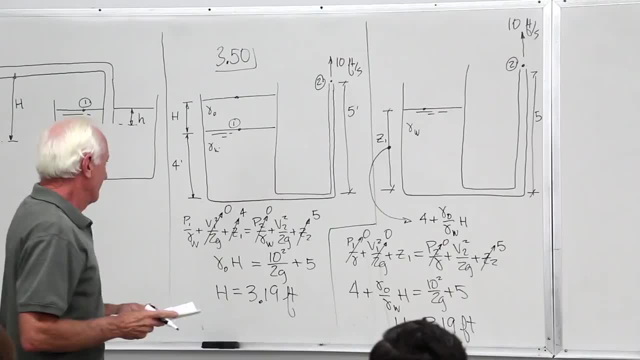 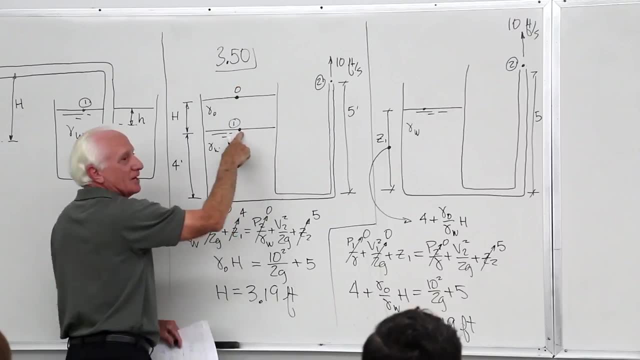 there's a choice, that's good, yeah, but how do you go from that step to the next step, to the next one underneath? oh, okay, yeah, if the pressure here is zero, what's the pressure? right where my fingertip is, chapter two go down in a static fluid. 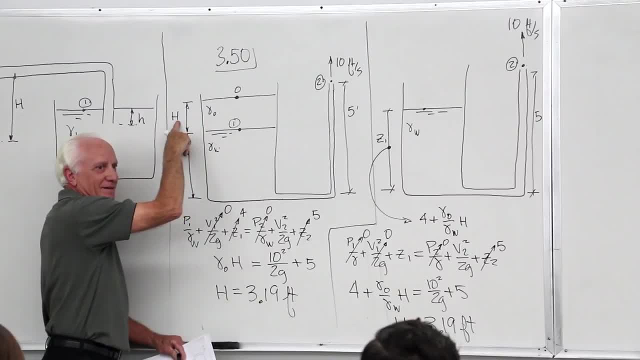 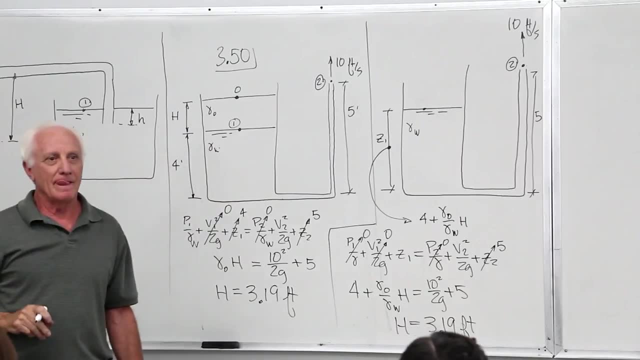 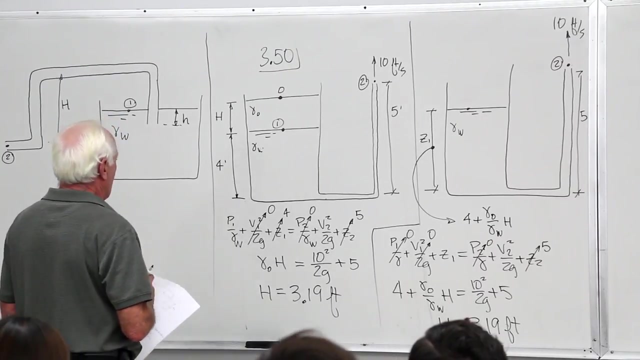 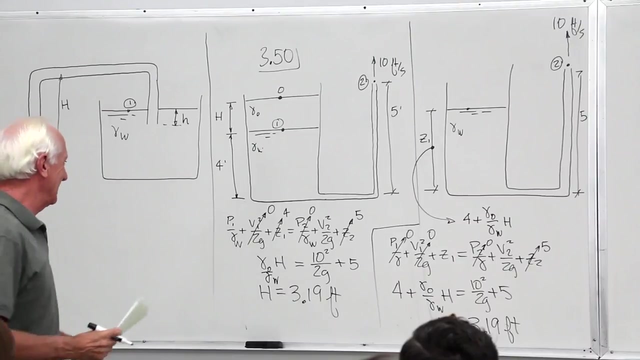 gamma Delta Z. what's Delta Z? what's the right? gamma gamma oil times H. but for your equation I think you only wrote gamma H, but you need it over gamma w. oh, yeah, yeah, yeah, yeah, thanks. yes, there you go, you got it right. yes, good, and plus four, yeah, yeah, yeah, yeah, yeah right, yeah, my, for, yeah, I skipped. 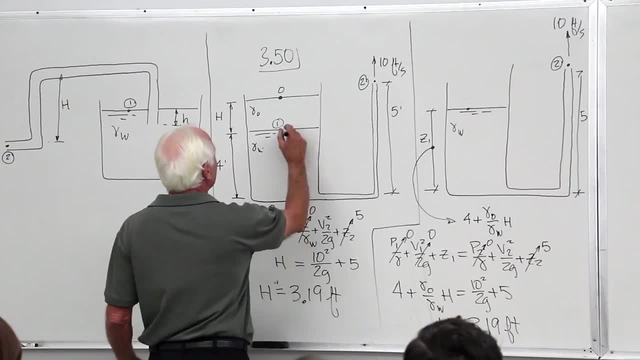 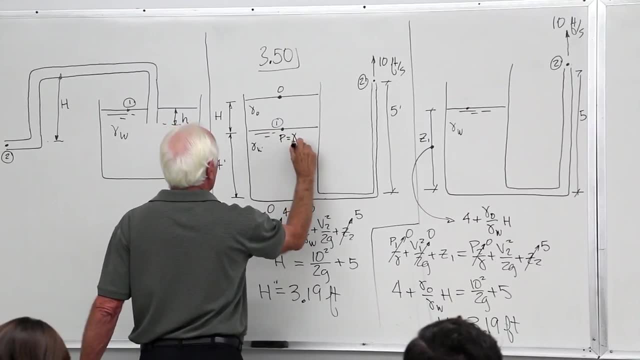 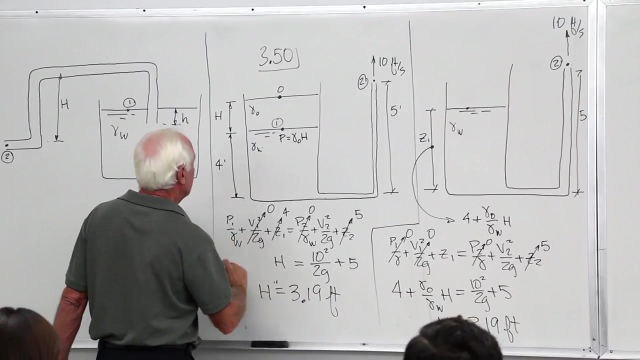 that step there. didn't idea where we go there. anything to put in this. this right here is a pressure here is equal to gamma oil times H plus the pressure up here zero. V1 is gamma oil times gamma oil times H divided by gamma water. Is that right? 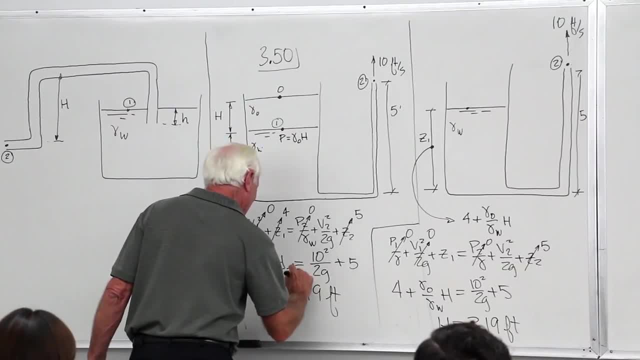 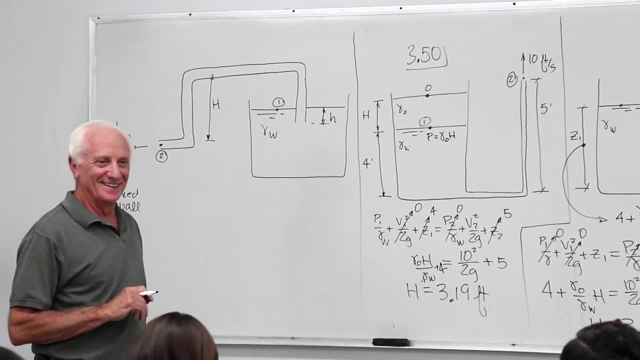 And then plus 4.. Plus 4, yeah, I'm glad you came to class today. It's funny, the answer didn't change, did it though? Because it's right here but it's not right there, But I'm. 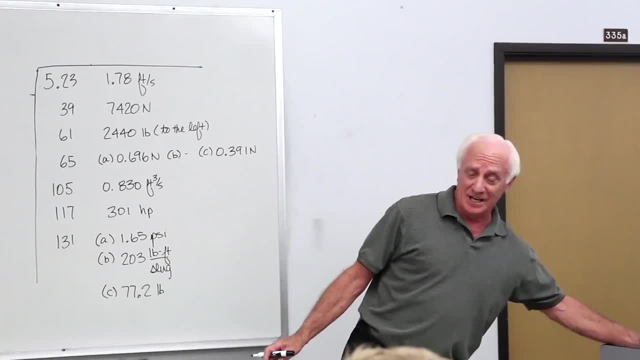 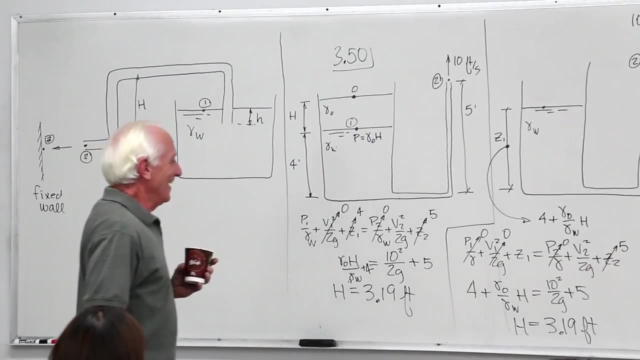 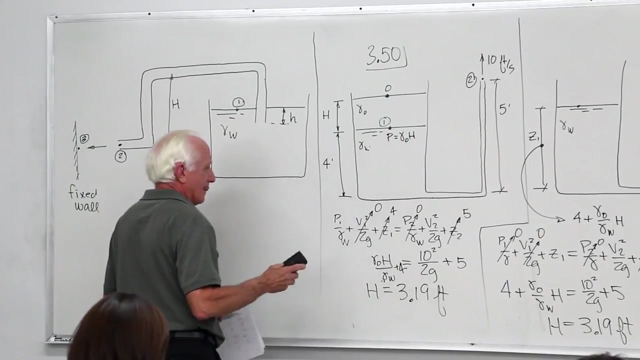 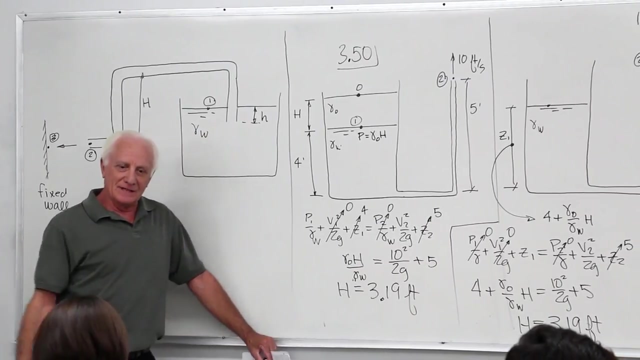 sorry. Okay, good, Thank you, because we need to catch those things in class. Sometimes I go a little fast and I jump over it. Okay, now let's continue on. Let me just mention this to you so you know If you do something like that on. 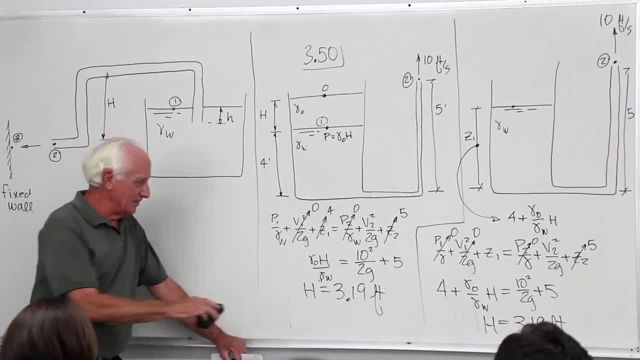 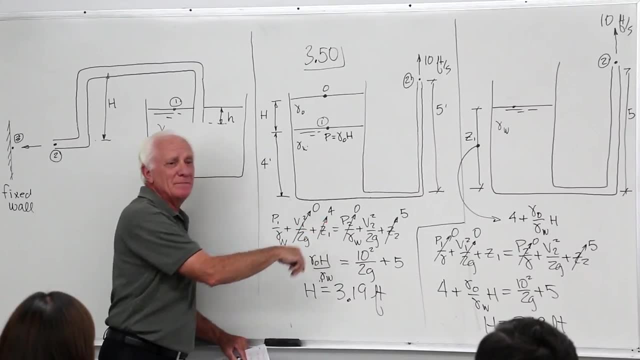 exams that I do on the board. I'm not going to penalize you as long as I see that 4. 4 right there. I know when you're in a rush sometimes you know you miss something, So I'm not going to. maybe half a point, which is nothing you know. 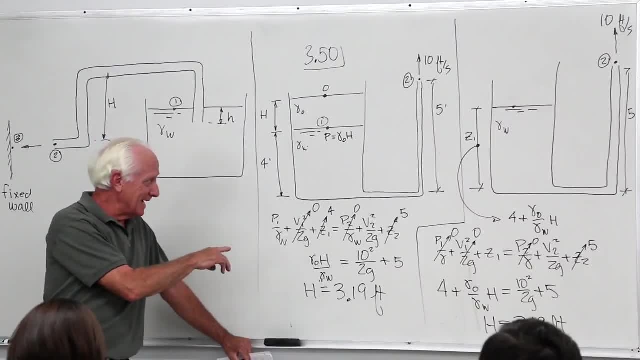 But you know I'm not going to penalize you, Just if it's written down somewhere like that, or if you write down Z1 equals 4, but then don't put it here. I'm not going to say, you know, minus 10 points. No, that's not right. 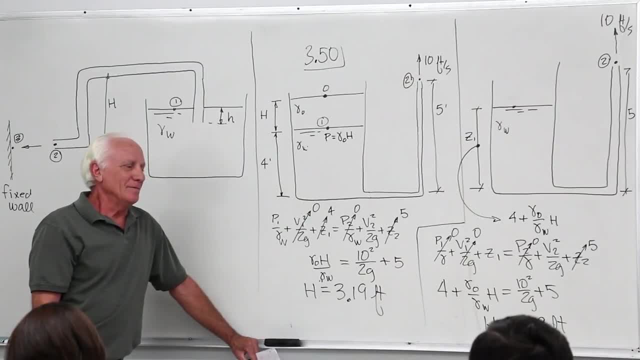 Because you saw it, You just in a rush, you didn't put it down there, So don't try and be careful, but I understand if you do miss some things like that. As long as it's in the equation written down, that's fine. 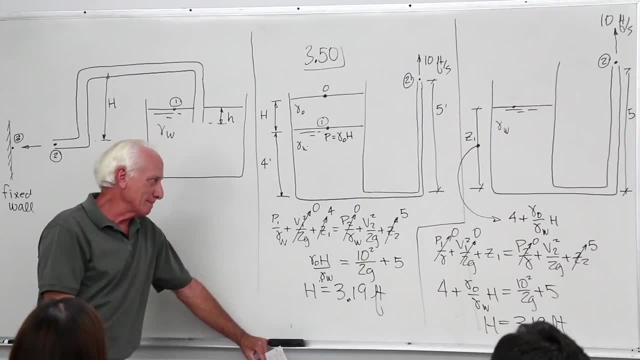 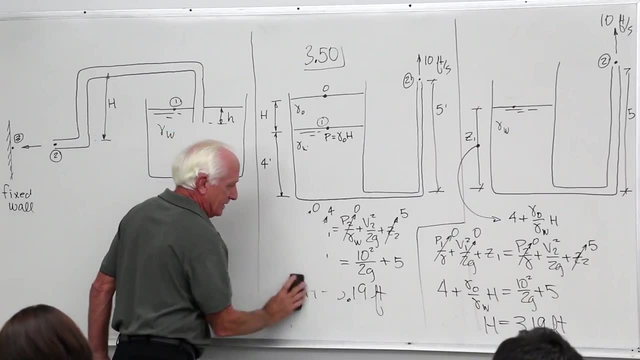 And the number somewhere for that symbol. I'm okay with it. Okay, Now let's, I'm going to erase this because I want to go back here and do this problem one more, a little differently than you would ask for homework. Now you see what. 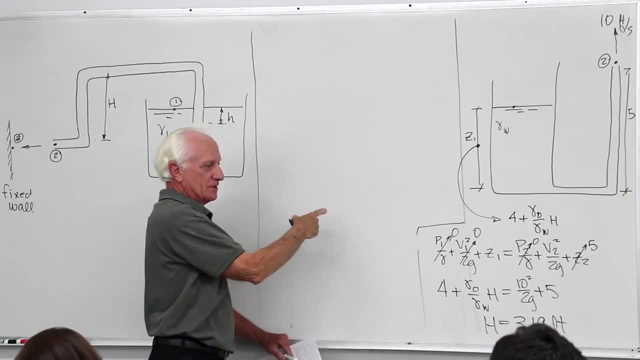 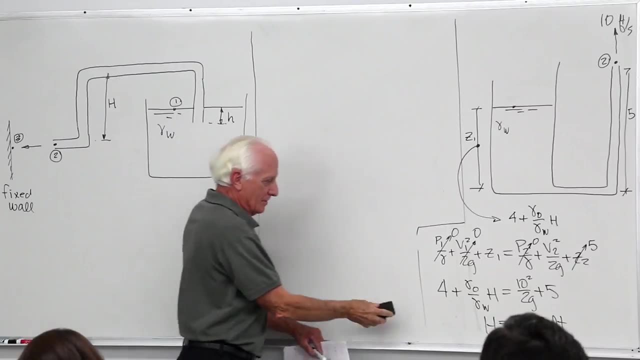 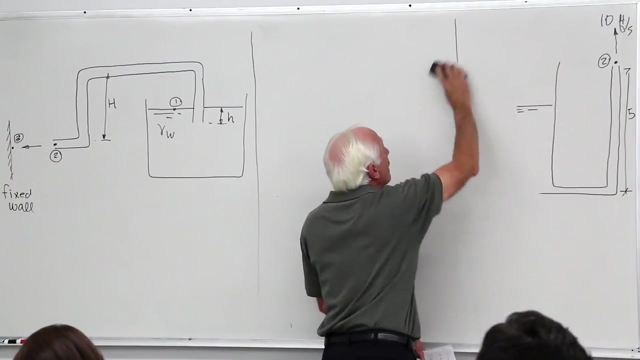 we're getting into here too, is these problems. This one here, for instance, involves chapter 3 and chapter 2.. Okay, So the further we get along in the course, the more chapters these problems may be covering. As I mentioned that one. 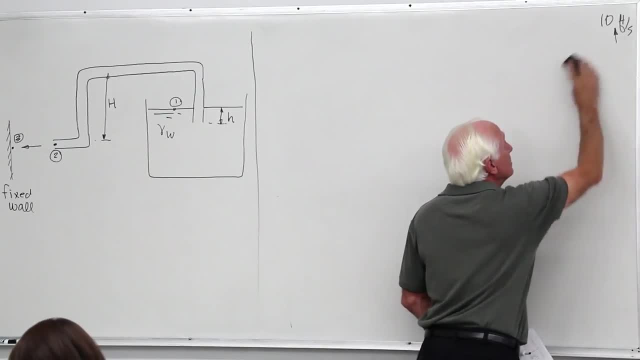 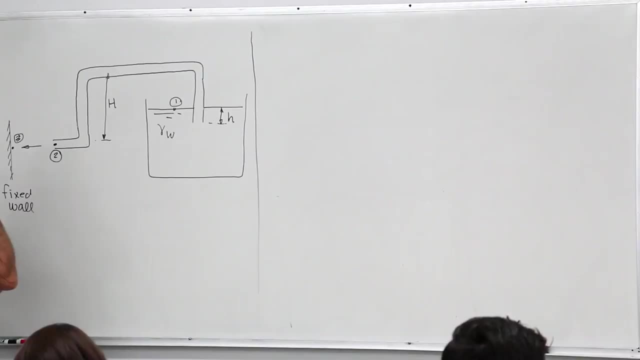 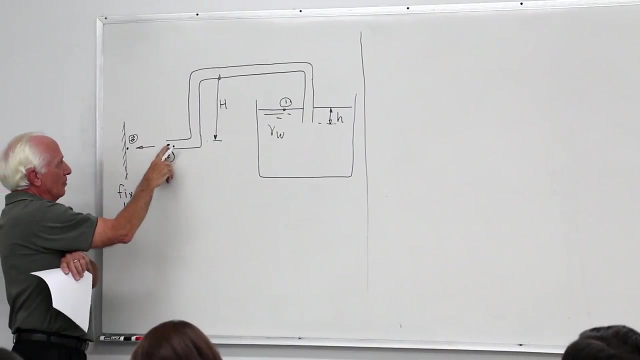 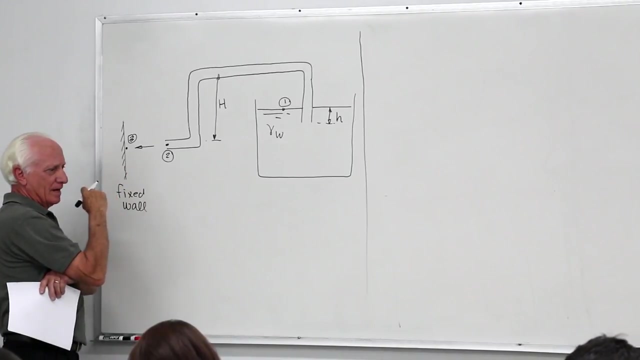 problem we just had with momentum and conservation of mass and Bernoulli's. All right. Point 2, the pressure is zero. just outside there We found the velocity of that Bernoulli's. I think. maybe my capital H is enough. Let me check my capital H on. 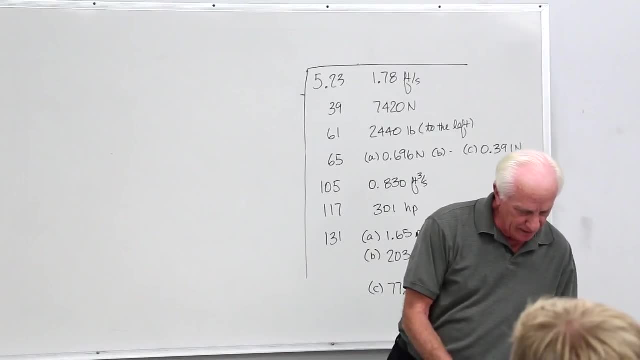 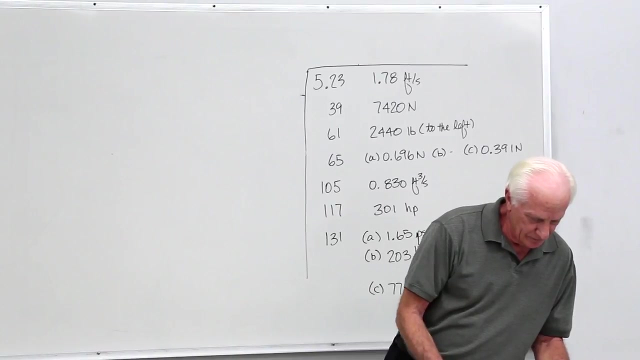 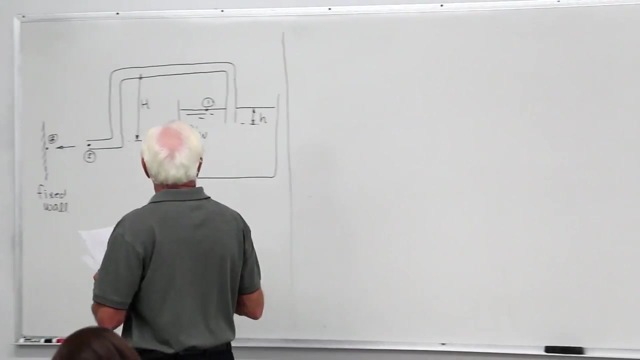 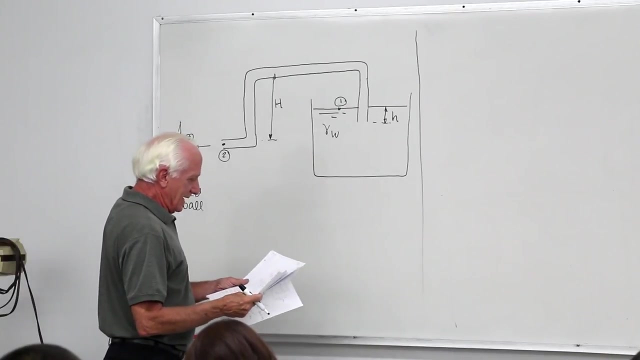 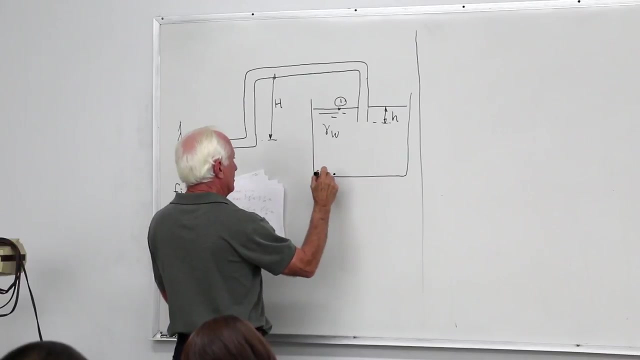 this one. I think I defined capital H differently, Okay, Well, I'll just go ahead and find it that way, And let's, let's see What if I ask you to there's point 1.. What if I ask you to find the pressure at point A? 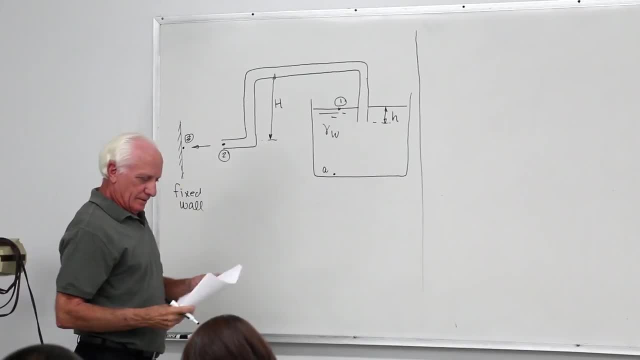 See, as we're going through stuff like this, we're reviewing for the second midterm, because a lot of this stuff involves earlier chapters, earlier chapters I just mentioned over here with the oil. Is the water moving there? No, Is it fluid? 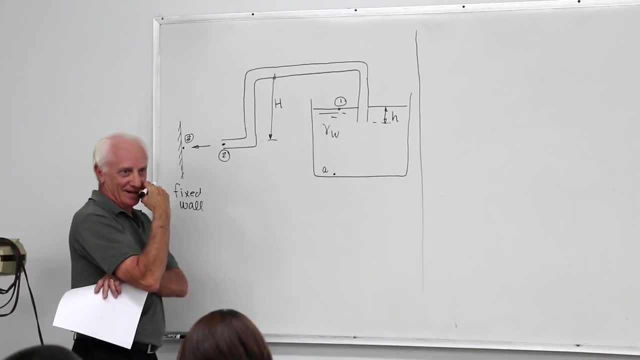 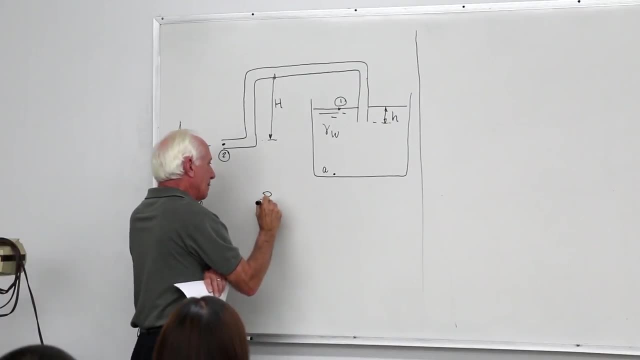 statics? Yes, Is it chapter 2?? Yes, How do I find the change in pressure Gamma times the difference in depth? Okay, PA equal P1 plus gamma. I'm going to call it gamma Gamma times the distance H. I'm going to change that because I think it's better this: 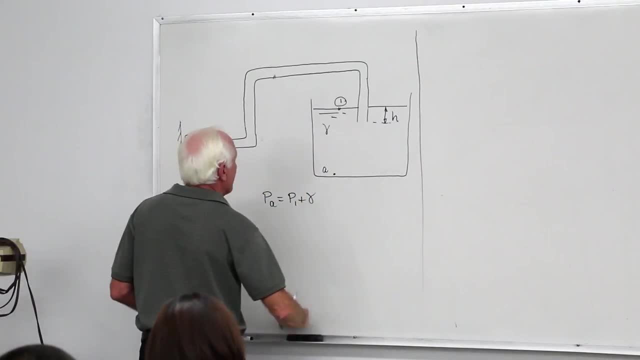 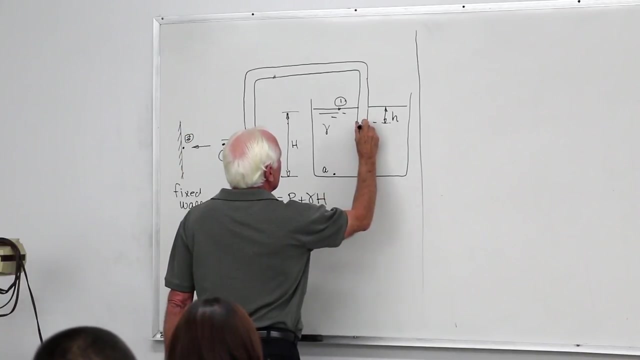 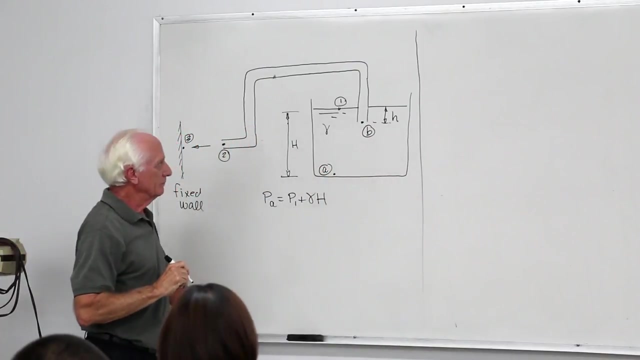 way with capital H up there. I might need to add more of this later, but I'll see. Okay, I've got the pressure at A. Now let's go from A to let's go to B, A to B. 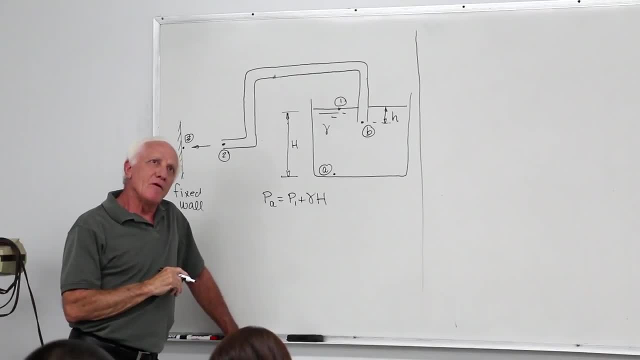 Okay, Here we go. now. Is the fluid moving at B? Oh, yes, it is. It's going onto a pipe. Okay, Can I use fluid statics? No, I can't. Can I use Bernoulli's? Yeah, as long as I. 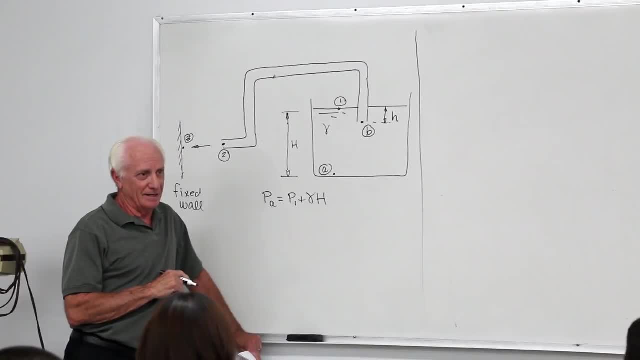 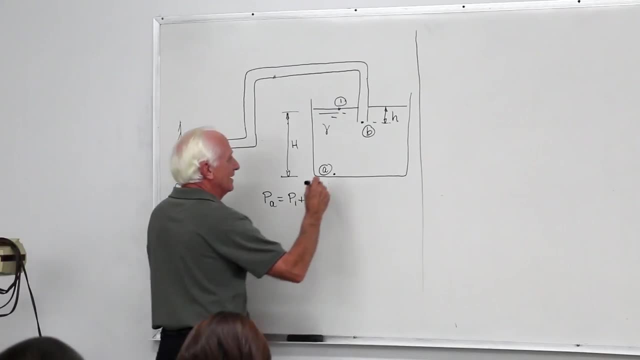 assume. What's that? again now, Incompressible steady state in this along the streamline. Where's my streamline? I don't know, but I'll pretend I know I think it goes from here up to there. Of course I don't know that, but I'm, that's my. 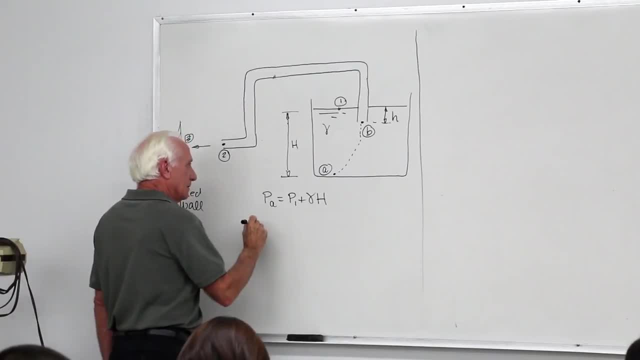 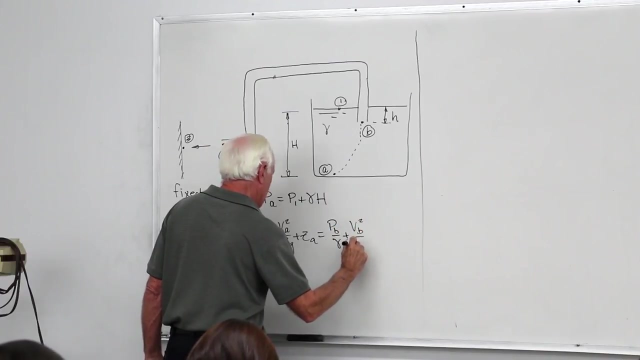 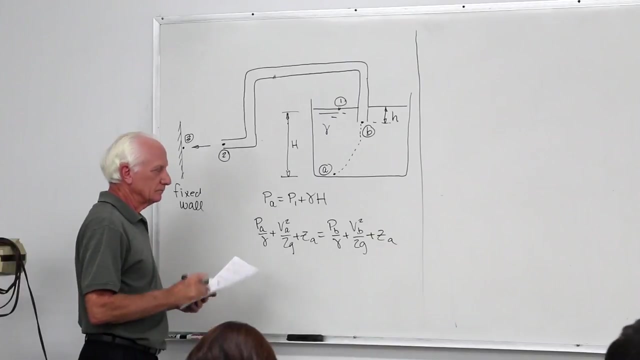 assumption. Maybe it does, It's okay. B A squared Z A, P B. B B squared 2G, Z A At A. I told you before, from the first going from 1 to A, velocity at A is 0.. I'm 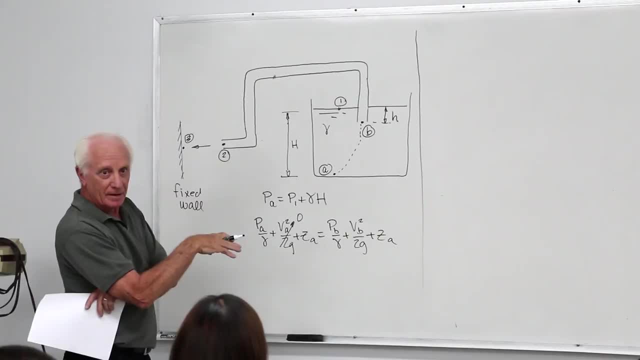 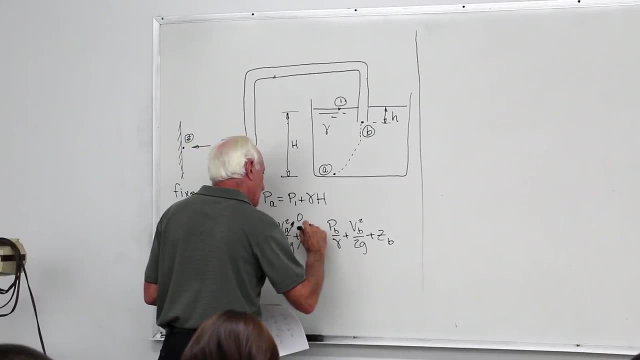 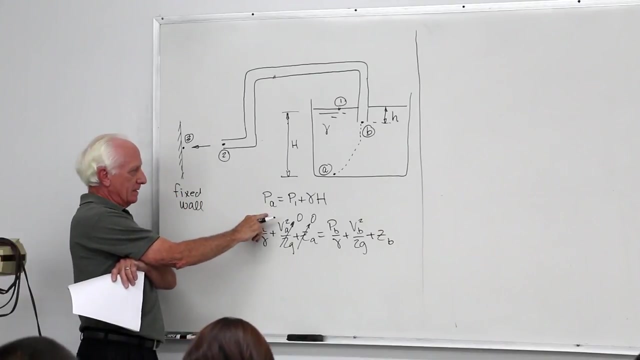 going to go to the bottom of the tank. I'm going to go to the bottom of the tank. I'll call it my data. Okay, Z A, 0.. Point A: fluid statics. Oh, right there, There, it's right there. There it is P1 plus gamma H. 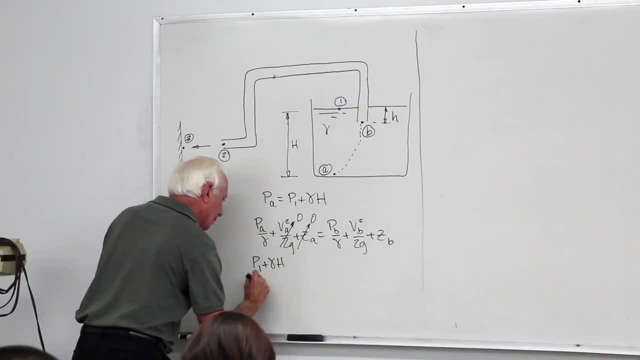 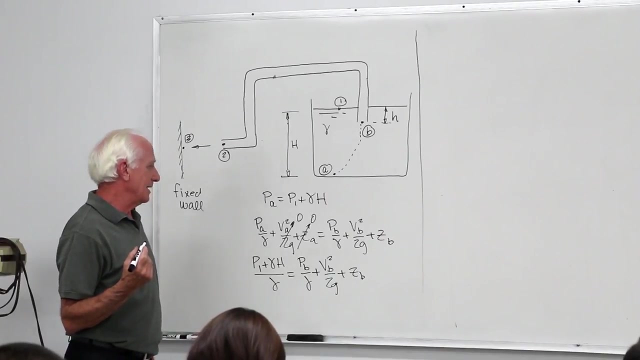 I typically know that distance C B, I know that distance C B, It's a knowing What don't I know. Well, I don't know. I don't know. P B, I don't know, B B, I don't. 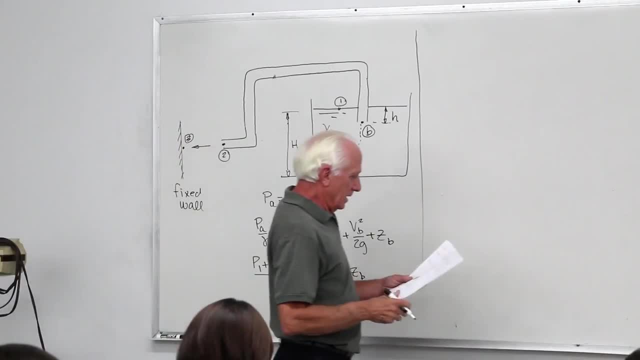 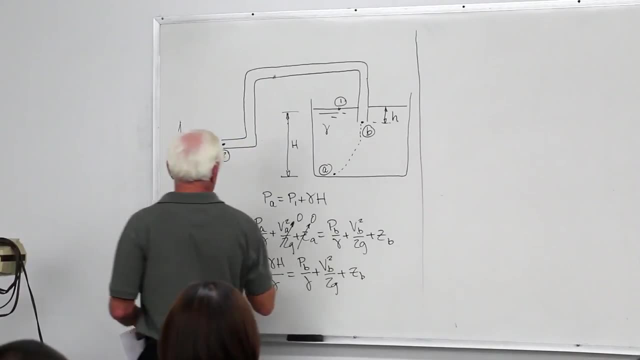 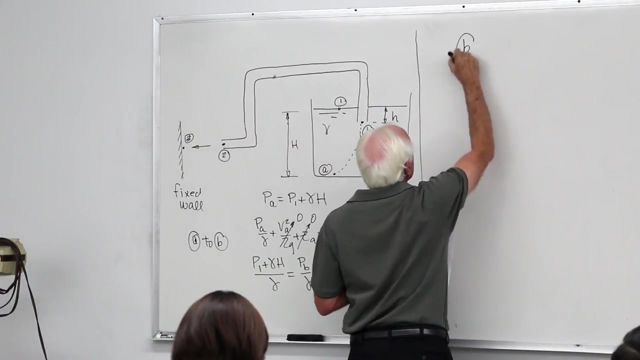 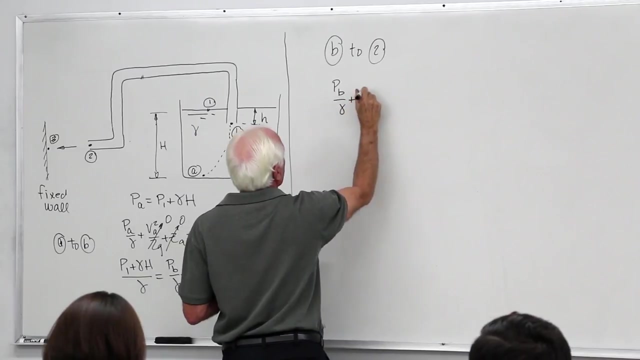 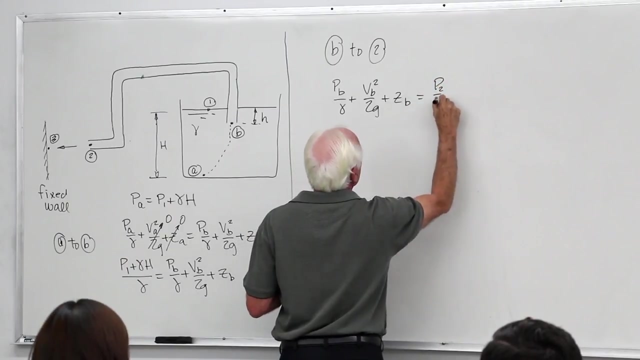 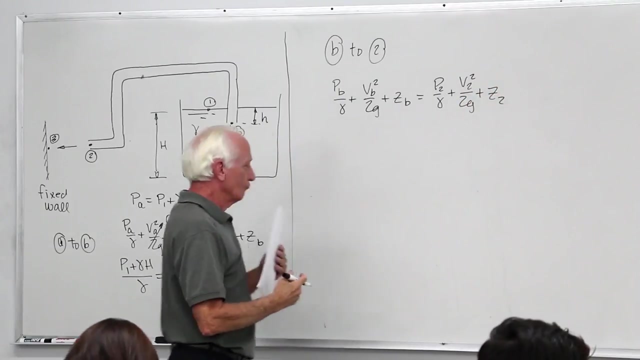 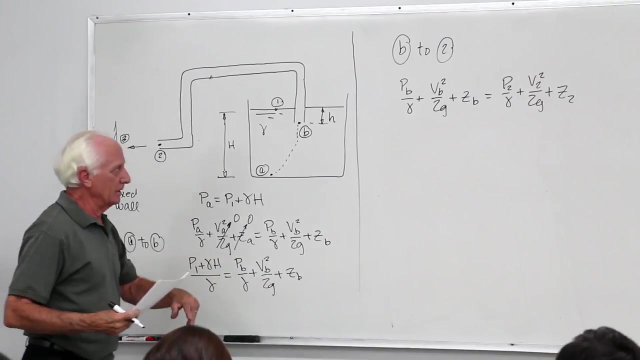 know, B, B. Okay, I'm going to write it from B to 0.2.. This is Bernoulli's A to B. This is B to 2.. Let's go back to B. Okay, None of those are 0.. Let them go. But this guy right here. 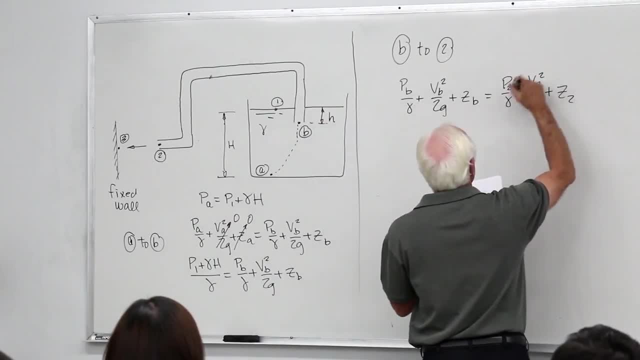 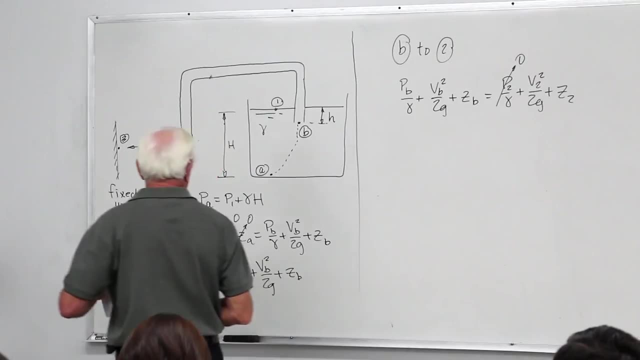 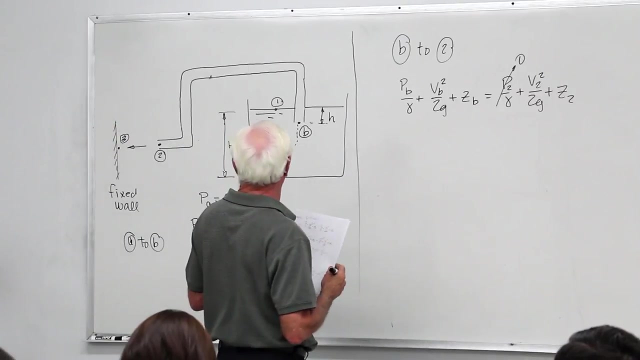 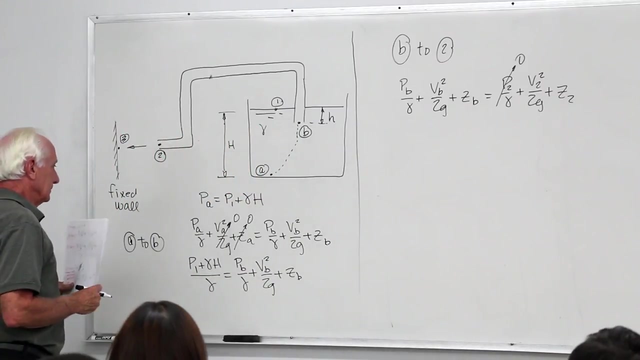 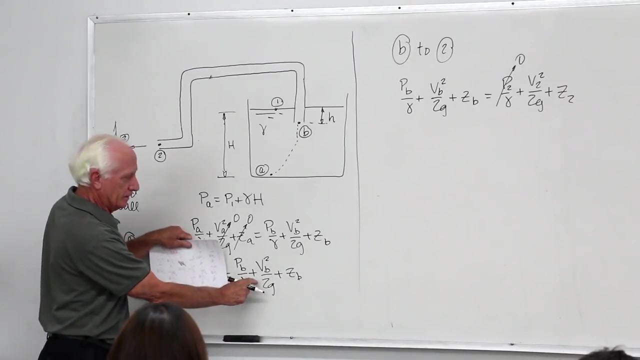 we know it's exhausting to, it's exiting to atmosphere. So P2 is 0.. We typically know Z A and Z, Z, B and Z2.. Okay, Those three terms right there. Are those three terms right there. 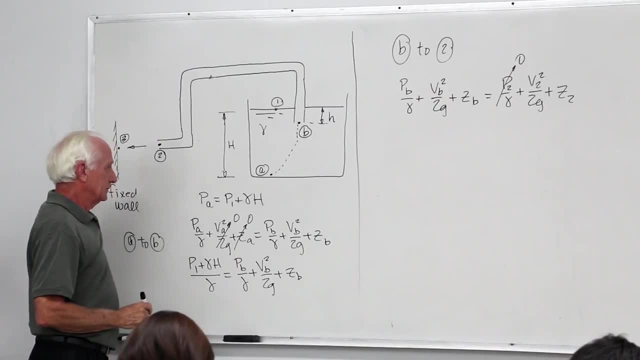 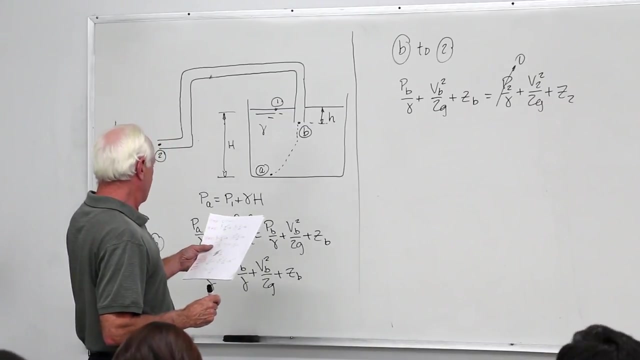 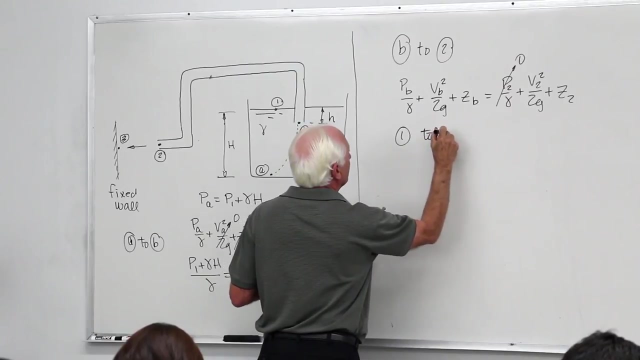 Those three terms are the same. Okay, Let's see what, Z, B, Okay, H, Z1.. Okay, Let's go from B to 2. we did. Let's go from 1 to 2 directly And don't stop at A and B. Don't stop at A and B, Go from 1 to 2 directly. 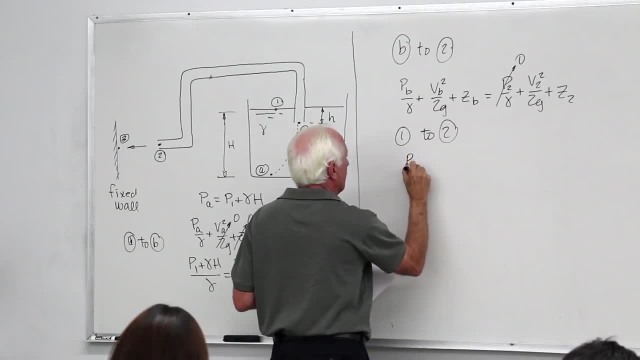 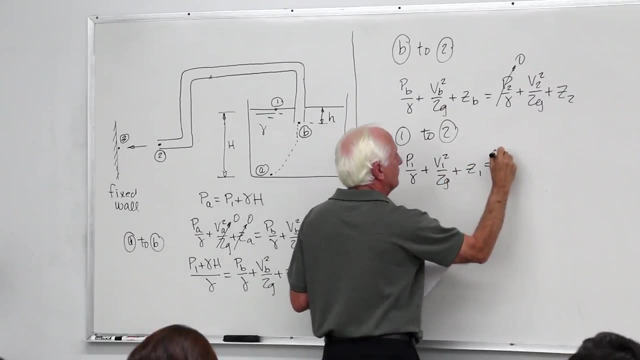 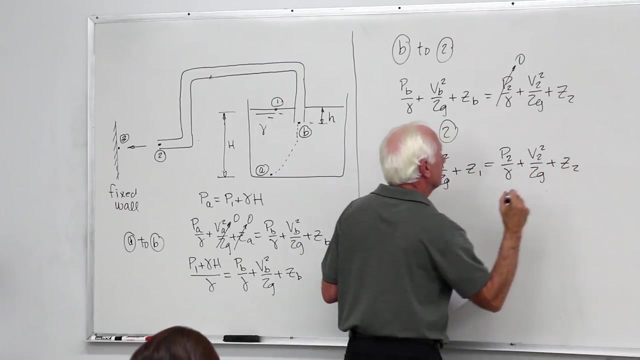 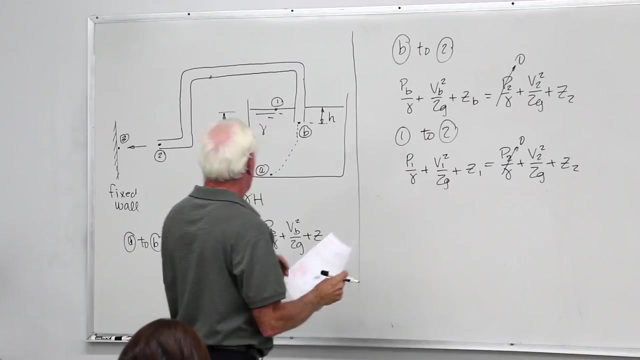 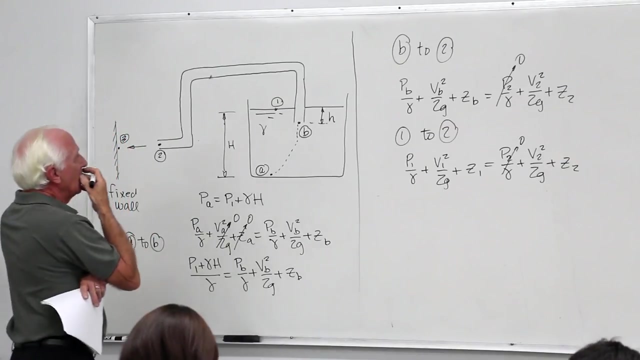 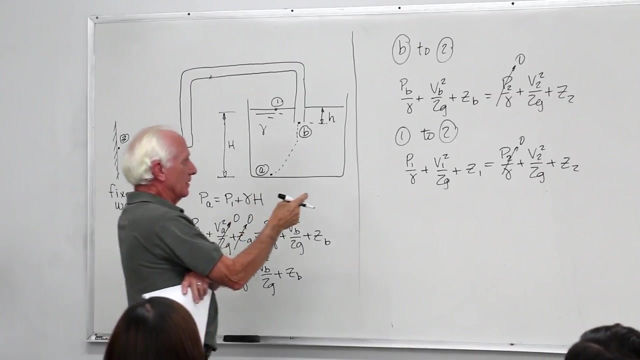 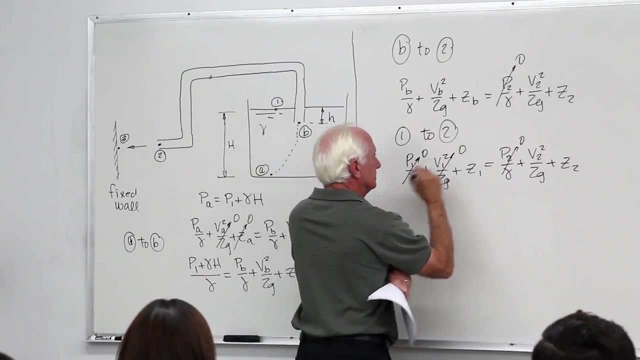 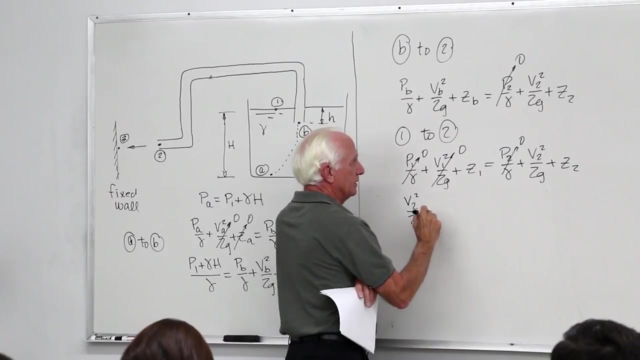 Okay, Okay, We know this guy Typically. we know this guy is 0.. This guy is 0.. So B2 squared over 2G is equal to Z1 minus Z2.. Delta Z, call it. So: B2 equals square root of 2G, delta Z. 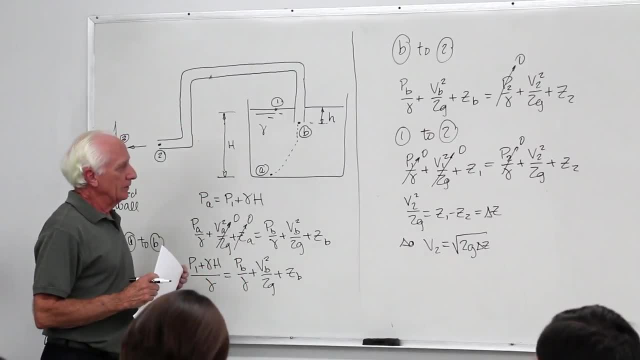 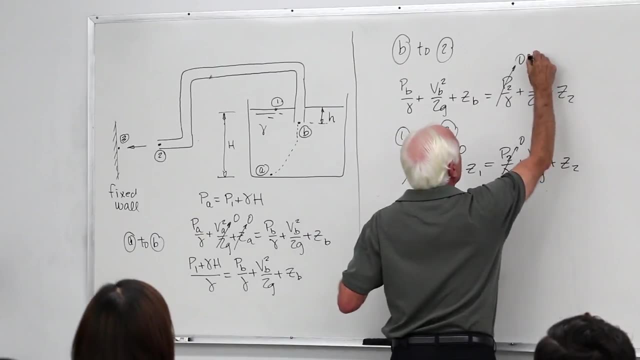 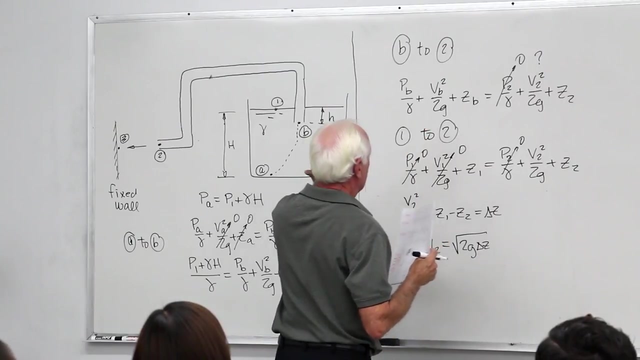 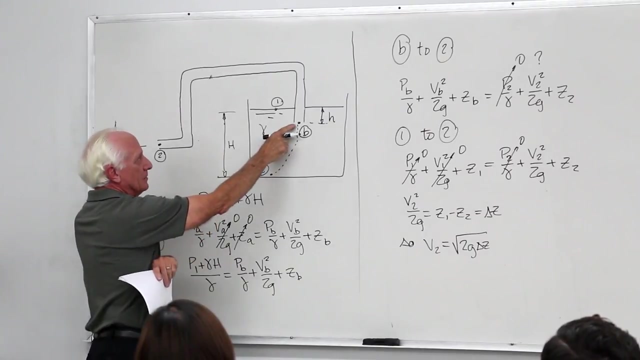 Could I get B2 from this guy here? I don't know that. Do I know B at B? Do I know B at B? Conservation mass: what comes in there must go out there. if it's steady state, Okay, Steady state. 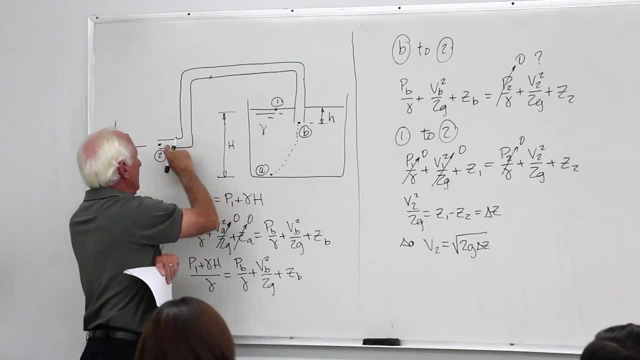 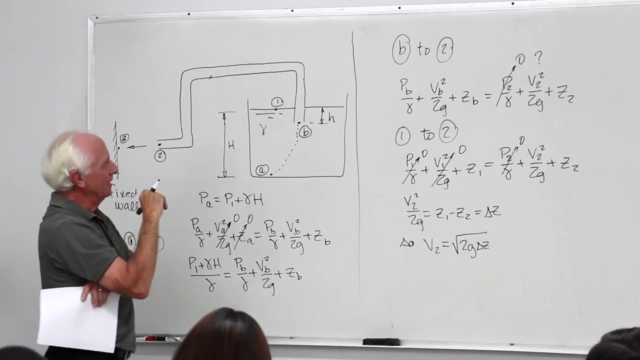 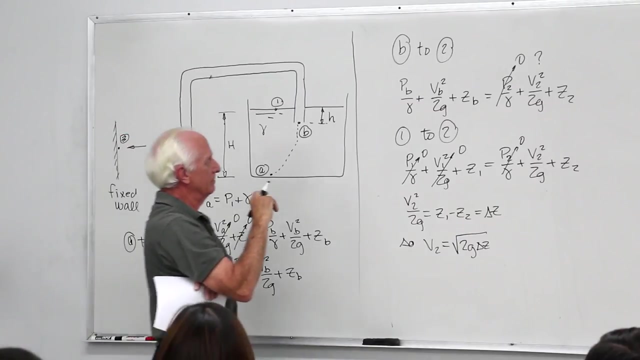 That's what it is: M dot B equal M dot 2.. Is it incompressible? Yes, it is Rows. cancel out. QB equal Q2.. It's at the same area. Yes, it is Same dimer pipe: BB equal V2.. BB equal V2.. BB- V2.. 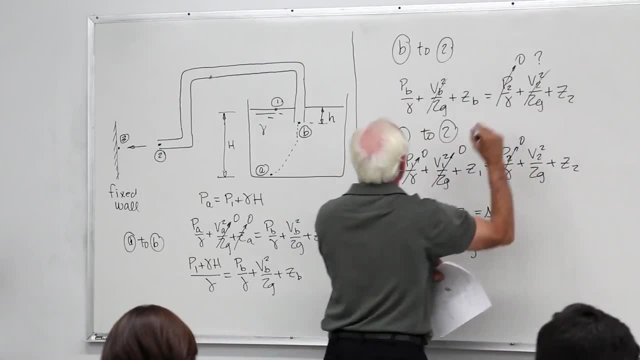 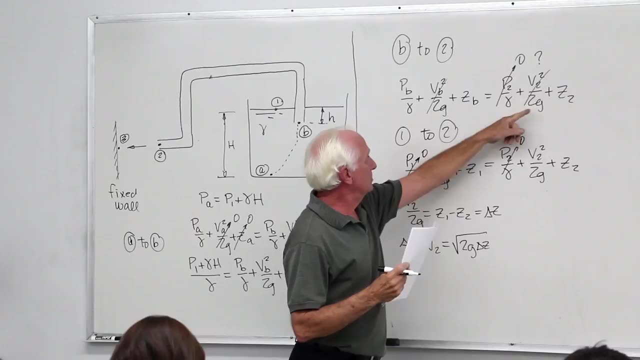 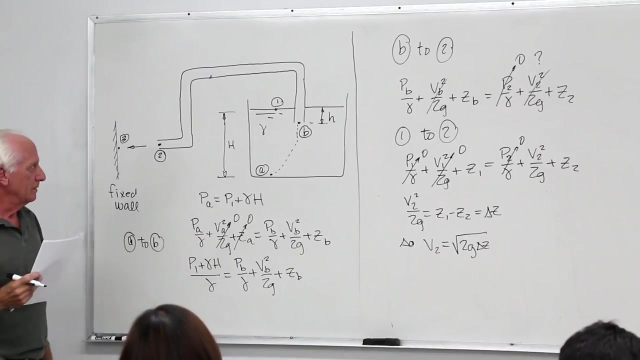 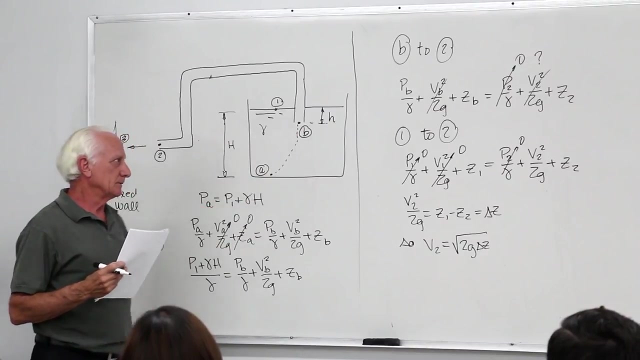 Okay, You want to find PB There. it is PB equal gamma times Z2 minus ZB. Yeah, So now we can find PB. Don't say it's gamma times H, Why? Because the fluid's moving at point B. It's not fluid status. You're going to find H, You just found. 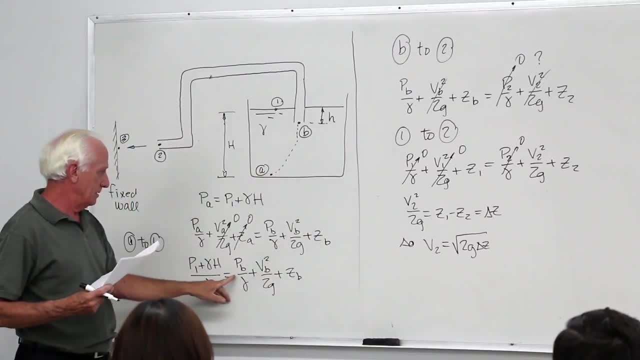 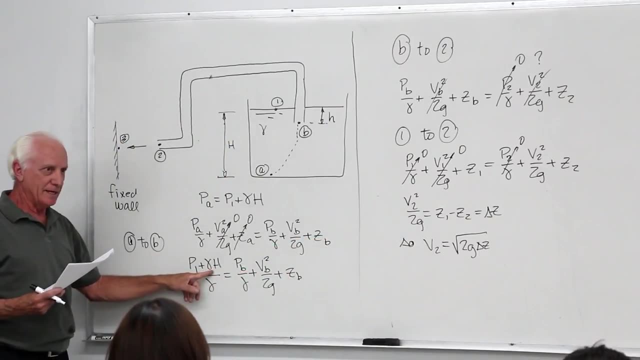 PB. I told you: right there, PB. You found PB, You found BB There. it is right there. And now guess what? Now you solve for H. So yeah, you can write many Bernoullis, but do it correctly. If somebody says what's the pressure, far away from the 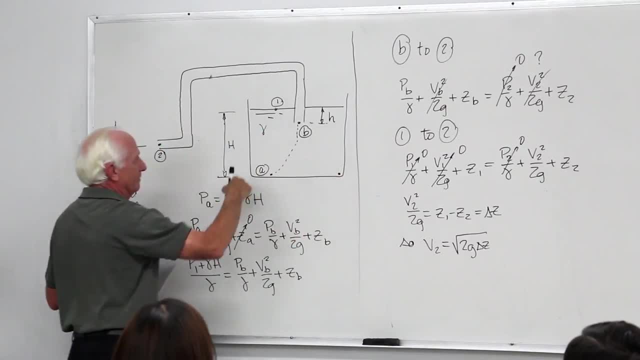 entrance is the key. What's the pressure in the corner? H times gamma. And the answer is H times gamma. The reason why? Because you're so far from the entrance to the tube that the fluid is almost at rest at that point, Almost at. 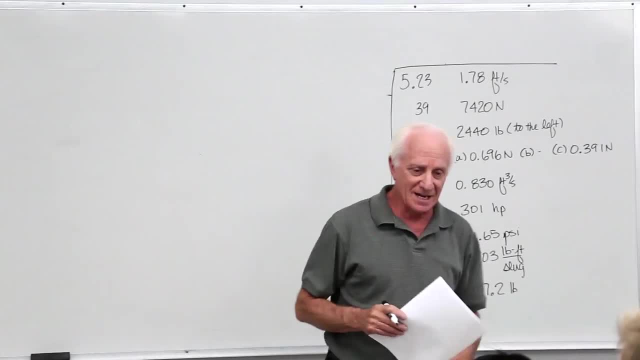 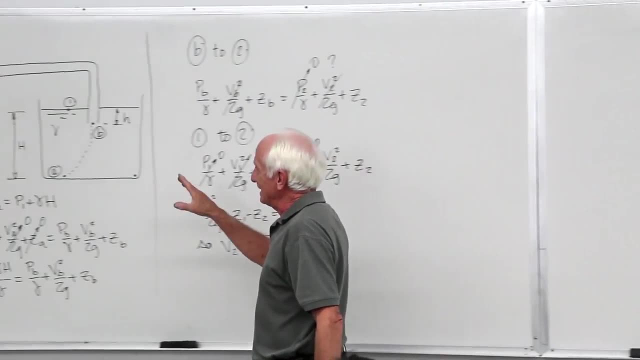 rest at that point- And we're going to assume it's at rest at that point- The velocity is essentially zero at that point. So there's lots of ways to solve that problem that you had for H And, by the way, you were asked to find the. 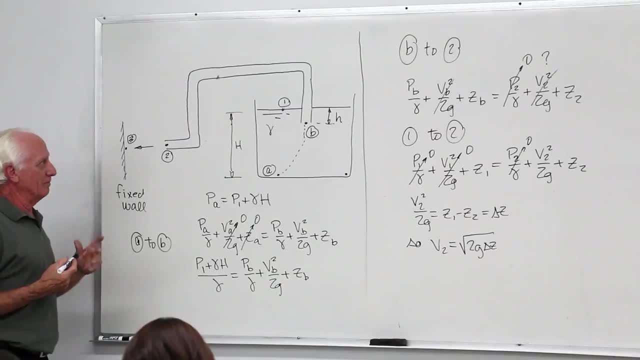 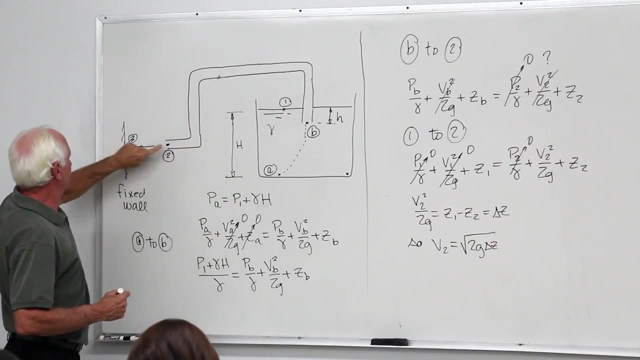 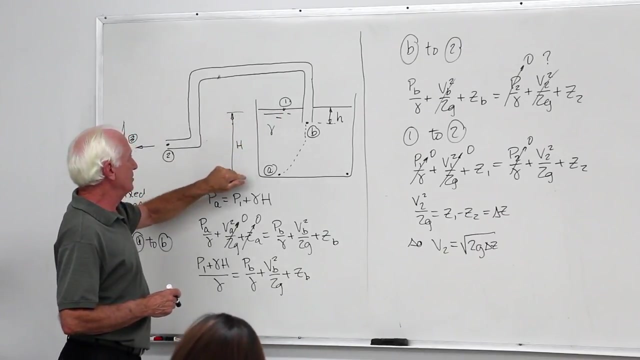 stagnation pressure. You want to make it. you want to start at one, go to the center, go all the way around until you get to there. Or if you drather, go from Bernoullis, go from two to there. If you start from here at one, you know H. 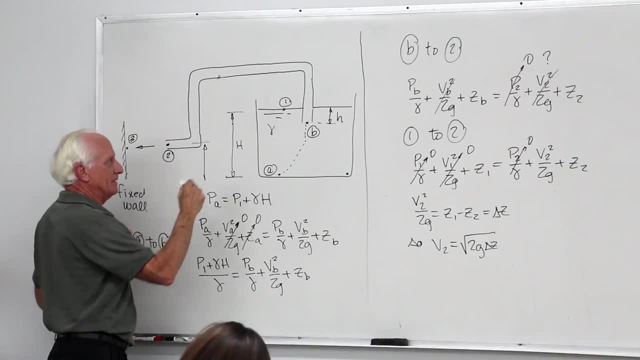 You're typically given this distance right here. I mean, in your case it might be the same as that. I get it the same height as that. You get that height, Okay, Which is a hundred percent. Like I said, you're given that height. So if you get 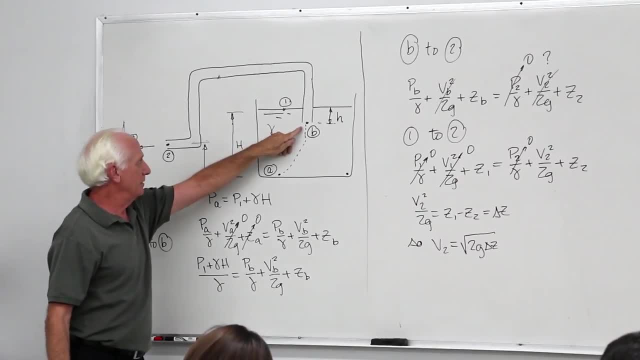 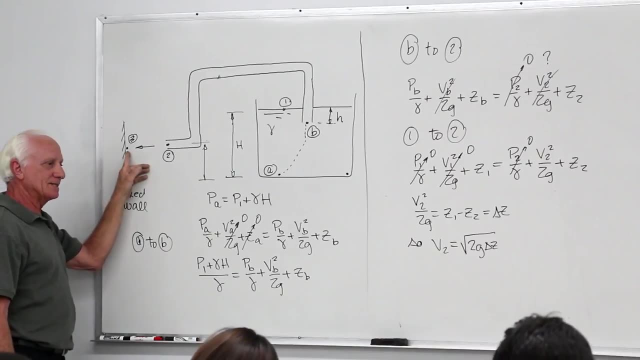 height of 3, like that. So if you go from here, if you go from here 1 to 2, or 1 to 3, pardon me, 1 to 3.. What's the velocity of 3? 0.. What's the elevation of? 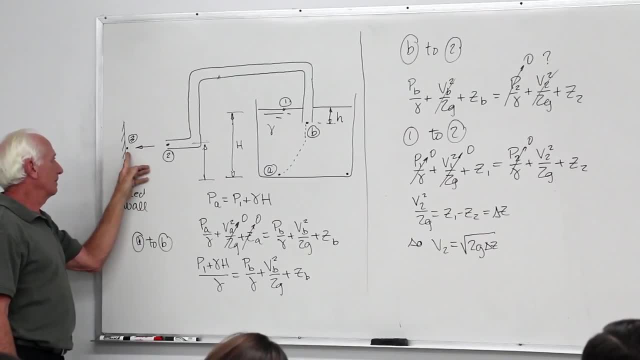 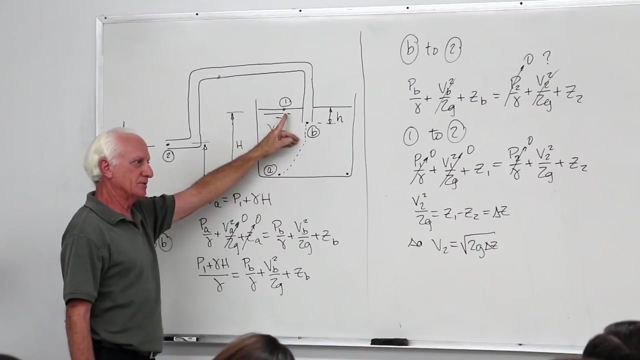 3? Z3.. I know it usually. What's the pressure of 3? Stagnation pressure. I'm supposed to find that Unknown Solve for P3, because P3 is Pstag, Do I know? velocity 0.. Pressure 0.. Elevation: Yes, H. That's how I find stagnant. 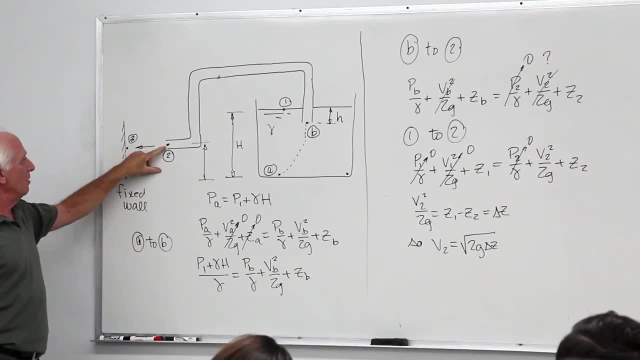 pressure. You want to start here, Not a problem. Do I know the velocity here? Yeah, I just solved for it right there, right there. I know V2.. Do I know P2?? Yes, 0.. Do I know Z2? Given to me usually Over here. do I know Z? Yes, I know. 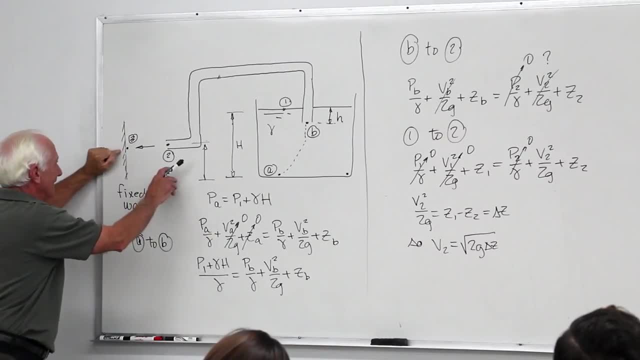 Z? Do I know velocity? Yes, I know velocity 0.. What's the unknown equation Between 2 and 3, the only unknown, P3. Solve for it: Stagnation pressure. So you can do this problem more than one way, You. 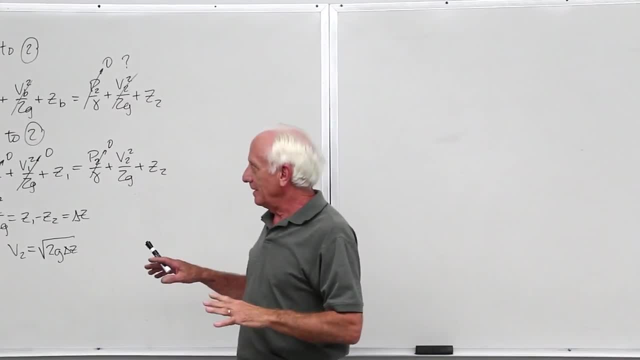 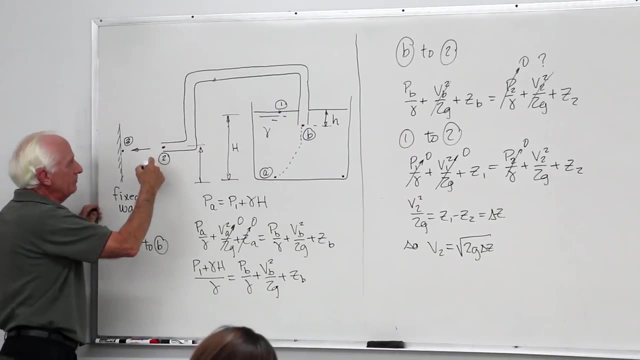 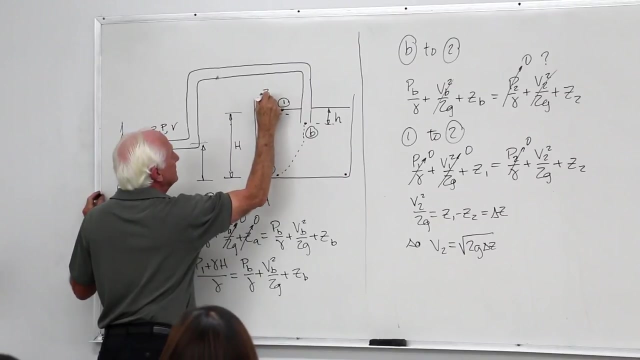 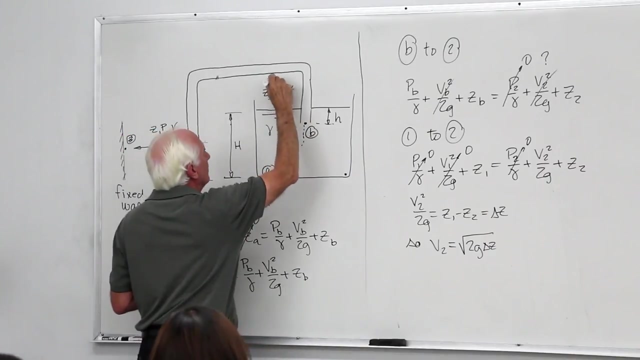 know, it doesn't matter. You write the equations down And I told you the rule: If you can put down where you know the most stuff: What's here Z P V, What's up here Z P V in Bernoulli's, What do I know? I know it. I know it. I know it. 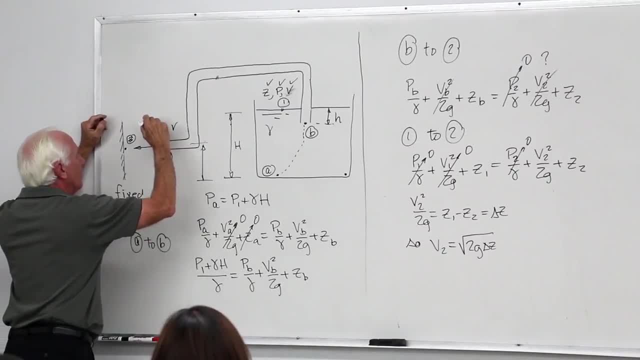 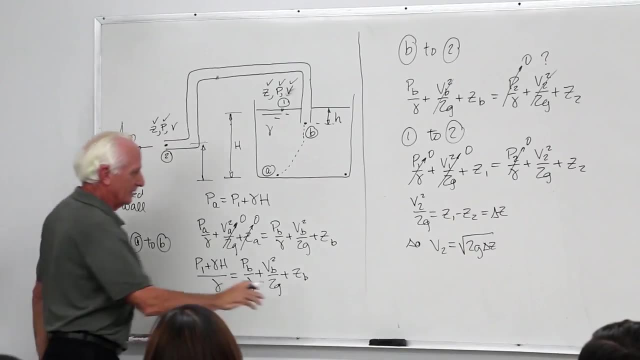 Good Over here. at point 2, what do I know? Oh guess what? One equation, one unknown. Now I go from 1 to 3.. Z, P, V, Okay, Okay. So this puts it right there. What do I say? 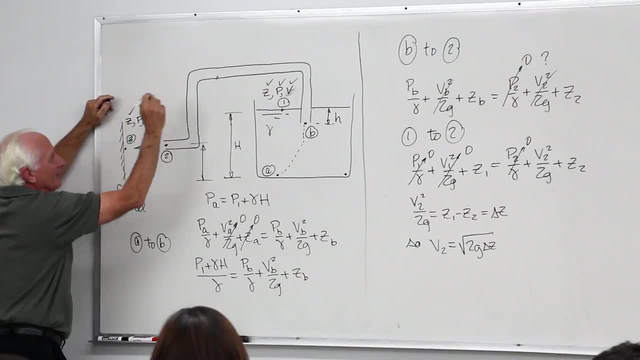 Do I know V? Yes, I do. Do I know Z? Yes, I know. Do I know Z1? Yes. Do I know P1? Yes. Do I know V1? Yes, Ah, unknown P. That's the way you play the game, So you logically think those things out. 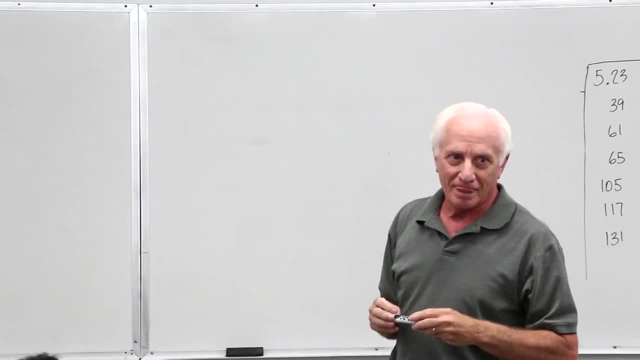 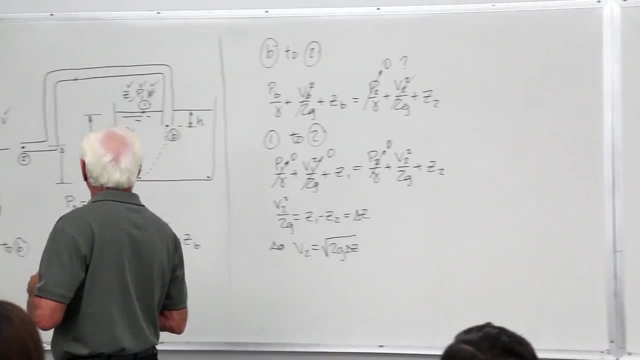 Would we ever be asked? well, there's a possibility to be asked, like how high the see the bend in the hose on the bottom 5.2, would be. Now, which one? now, I'm sorry, The for this left height. 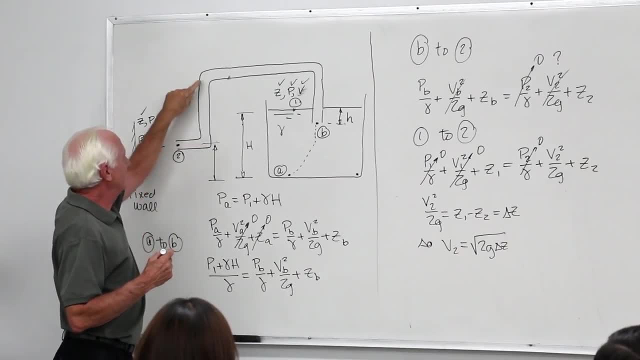 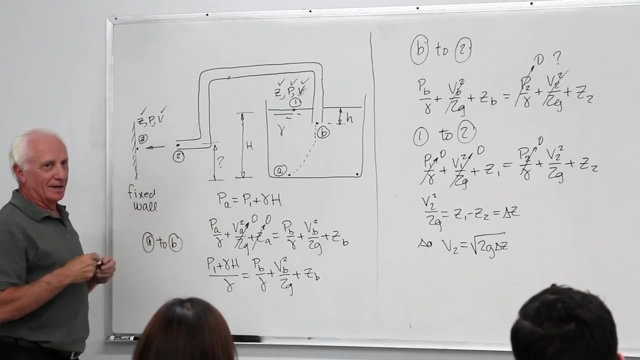 Left The height that you have not labeled That height right there, No, the height of the bend. Oh yeah, yeah, yeah, yeah, yeah, this height, Yeah, Is that variable? does that affect? would that affect the velocity, Like if it were lower? would that increase the?